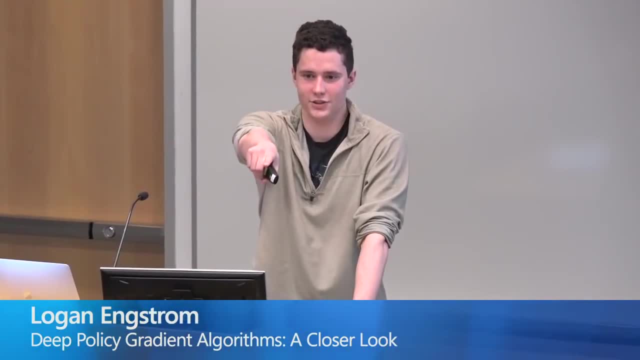 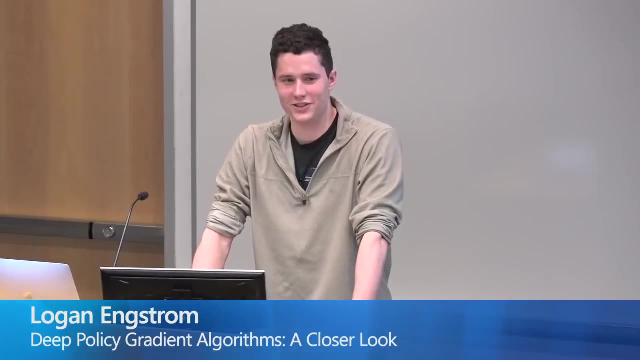 of deep reinforcement learning. This is joint work done with Andrew right there, and Dimitris and Shabani, and also some of our collaborators at Two Sigma and, of course, our wonderful advisor, Alexander Mondry. So let's just get started. 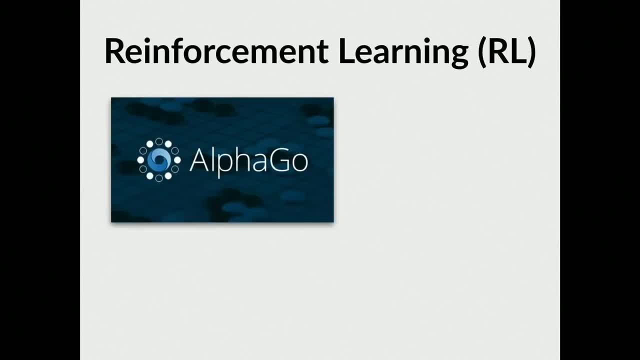 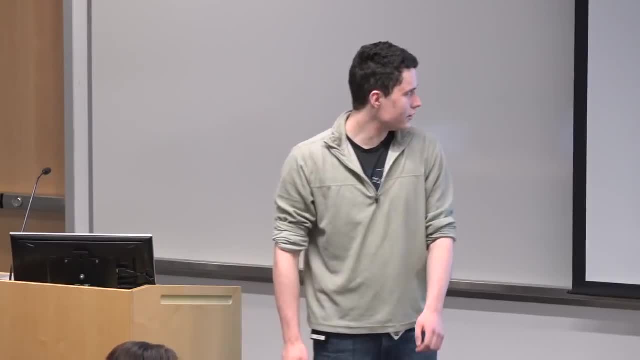 So we've all heard quite a lot about reinforcement learning. Probably the most well-publicized example of reinforcement learning recently has been AlphaGo, in which Google made some kind of reinforcement learning algorithm to play the game of Go. There's also applications in robotics. 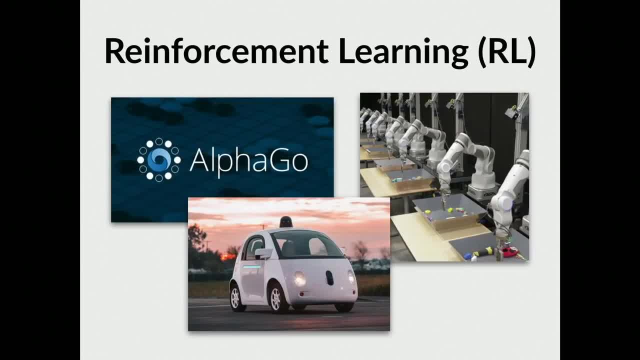 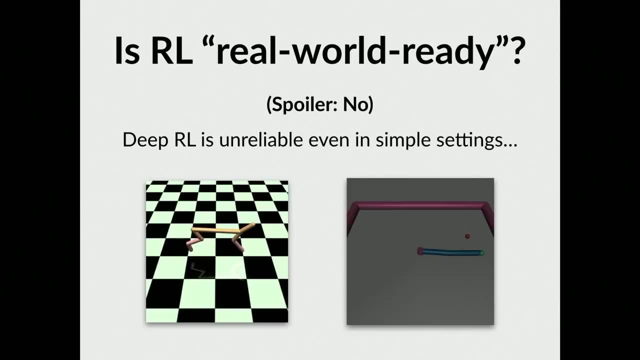 as well as even self-driving cars. But all these applications begs the question of whether reinforcement learning is really ready for the prime time, and the answer is no. Deep reinforcement learning is pretty unreliable, even in very simple settings. You can see this in these two examples. 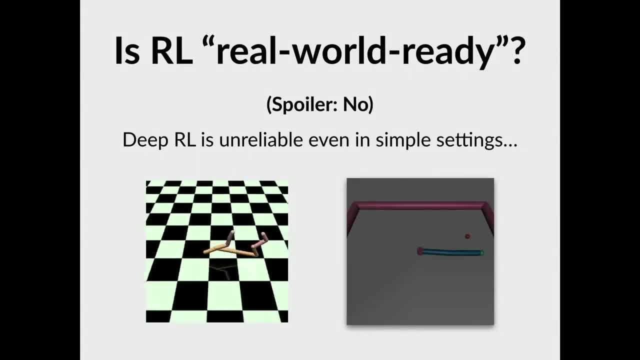 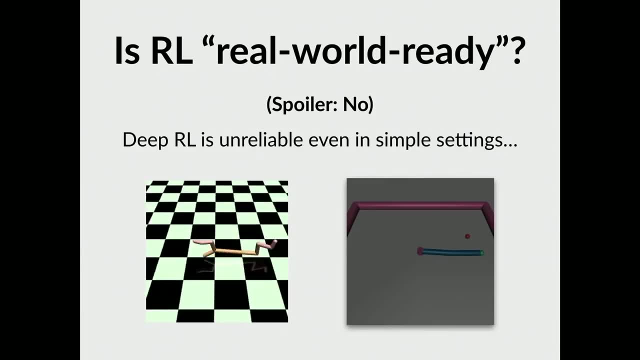 One example. so there's this little half cheetah and it's supposed to be running along like a real cheetah, except in two dimensions. But it's not really doing that. it's going on its back because it fell into a local minima and it can't get out. 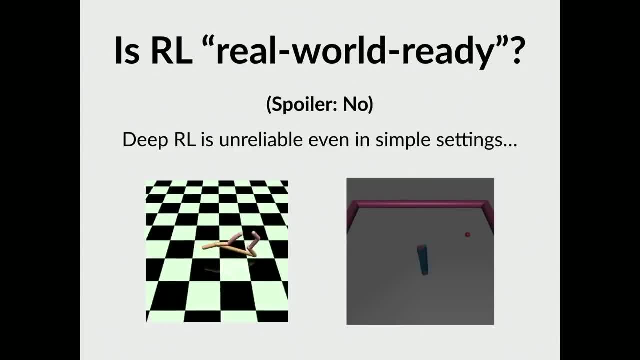 Another example is this little reacher robot, and so it has his arm and it's supposed to be reaching to touch the dot, But what happened was initialization. this reacher robot had really high weights or something, and so it just got into the spin and it takes too many steps. 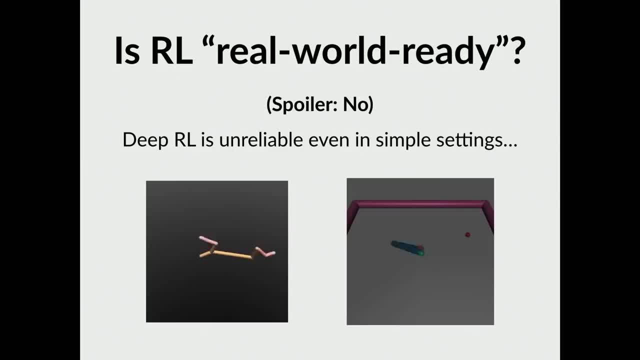 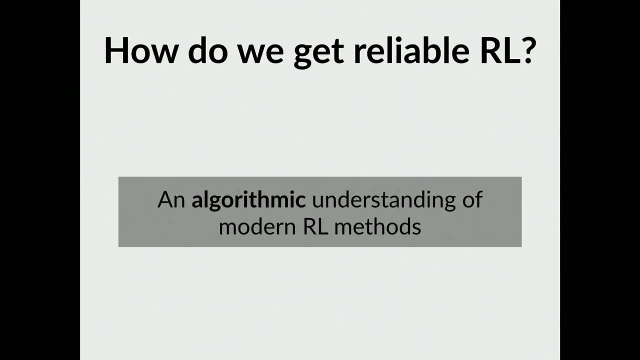 It's a classic exploitation trade-off and it was not able to get out of the spin because it's in another local minimum. So how do we really get to this reliable reinforcement learning? Of course there's a bunch of problems that need to be. 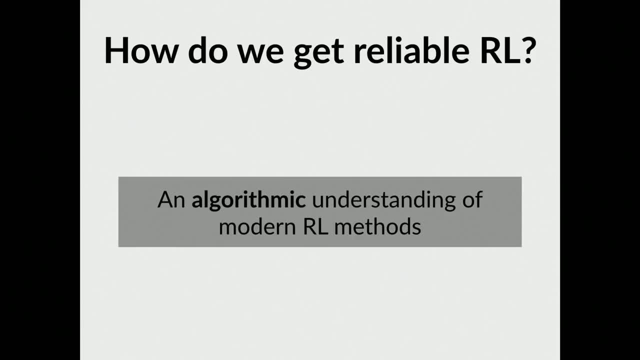 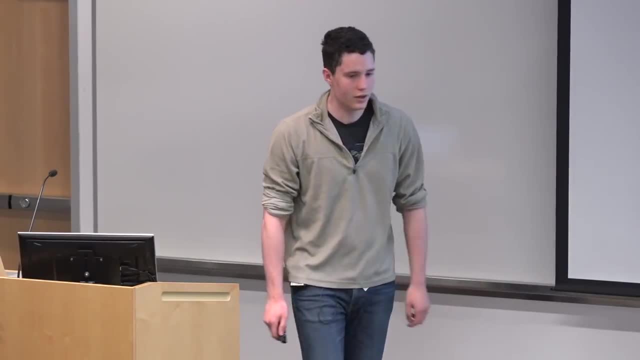 solved, like value alignment, among other things, But the avenue that we're going to look at today is obtaining an algorithmic understanding of reinforcement learning, because you can't really make something reliable until you understand how it works, So we're going to first give. 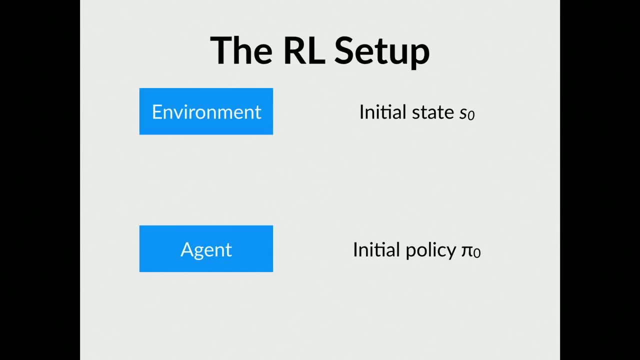 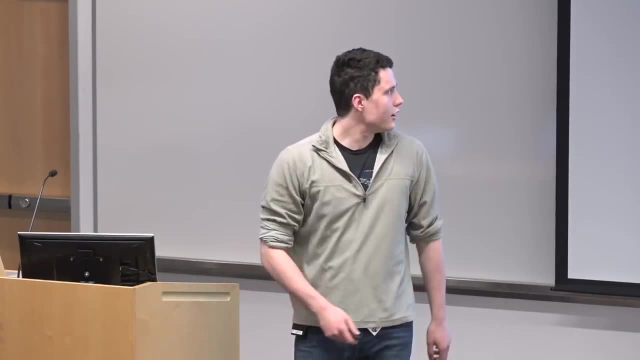 a brief overview of what the reinforcement learning framework looks like. So you start off with some kind of environment, and I'm going to use the example of a stock trading environment. So you have the market, that's your environment and you have the initial state. 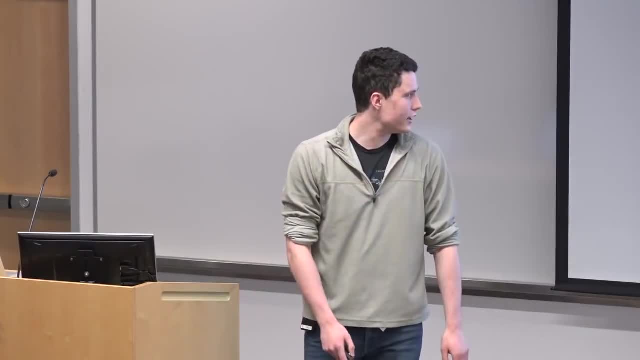 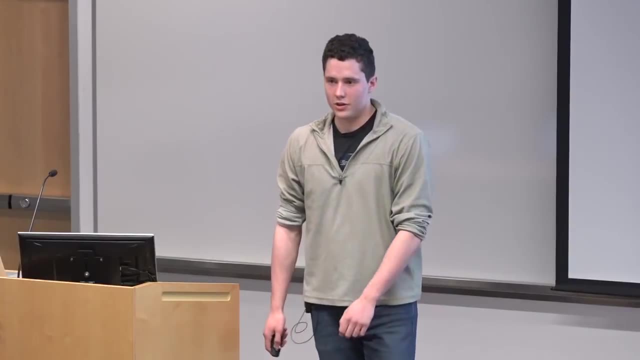 which is a bunch of stock prices and a bunch of tickers, and our agent is going to be a robot and the robot is going to be trying to trade on the stock market and make a lot of money. It has some initial policy. 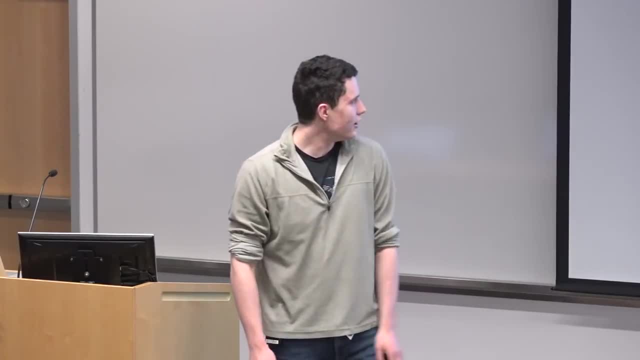 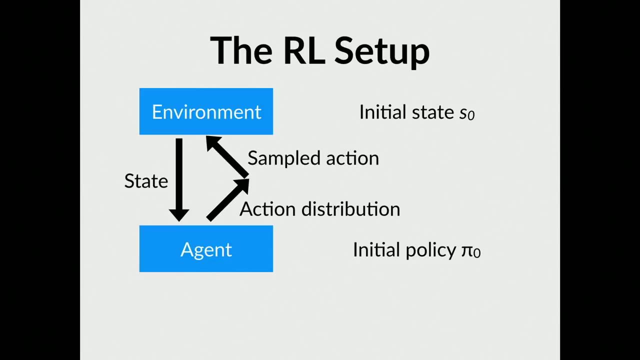 maybe some kind of expert policy or just random initialization, and at the very beginning the agent sees the state of the market, and the state of the market is, as I just said, all the stocks and the prices, and then the agent takes that and then it uses. 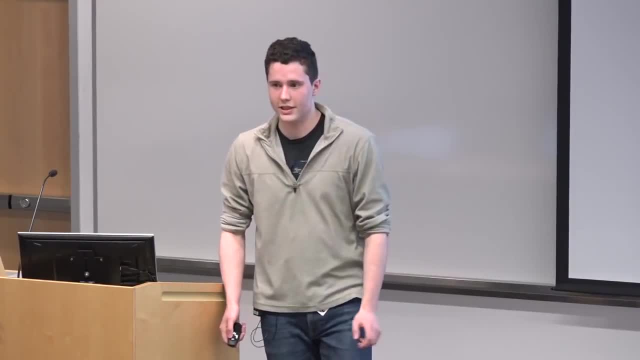 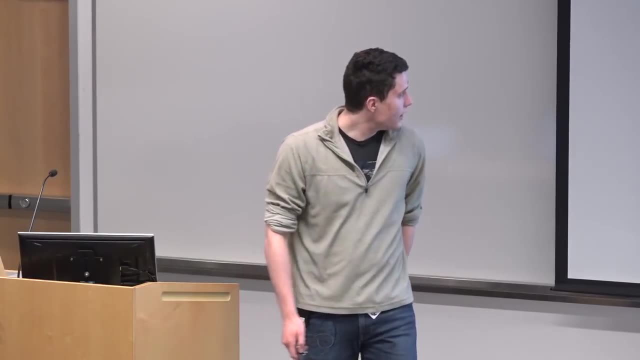 its policy to make a distribution over all the actions they could possibly take. So that could be like sell a stock, buy a stock whatever. Then it chooses from that action distribution uniformly and then it feeds that back in the environment by playing it. 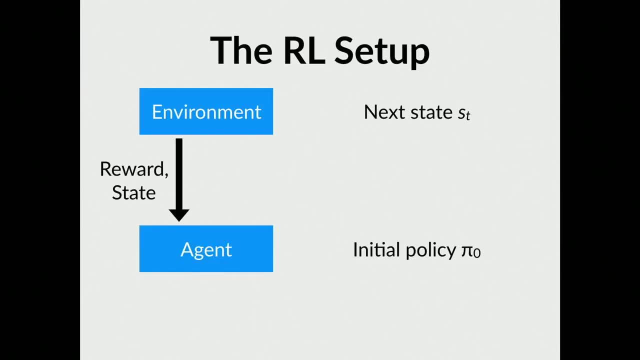 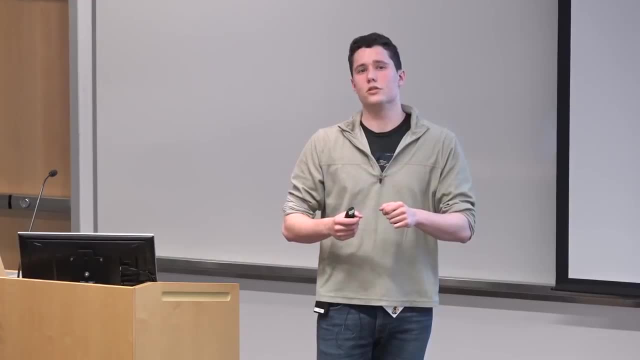 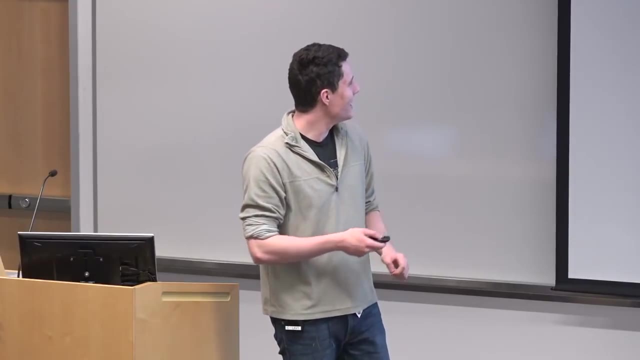 Then after that the environment shifts to the next state. So if you sold a stock, maybe the stock price for that stock will go lower. Yes, Then that's why we're not two sigma anymore. So anyway, the state will change. 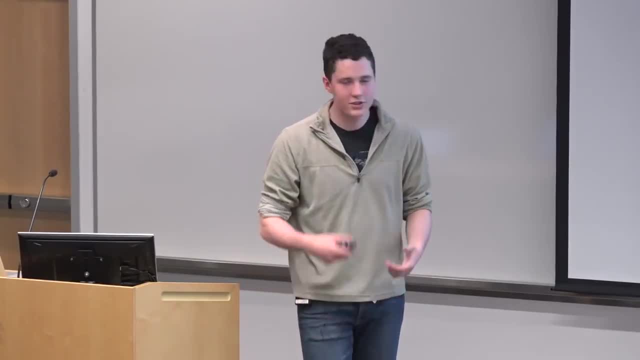 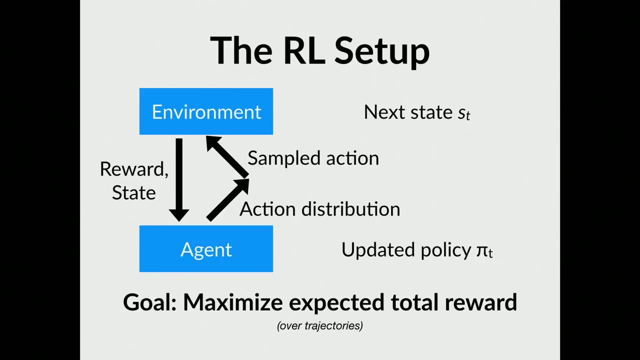 and then you'll get some reward, like maybe you made money, maybe you didn't make money, and then, based off of that information, you're going to shift your policy To make your agent even better for the next round. and that's going to repeat a bunch of times. 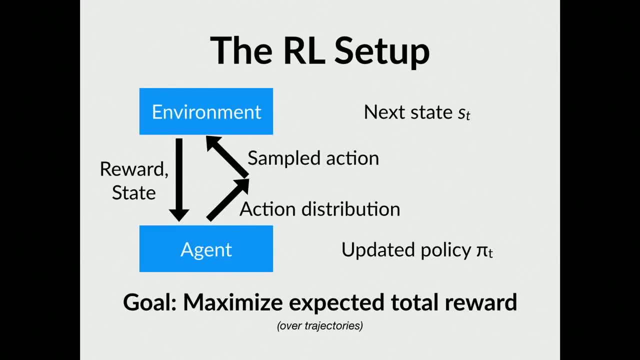 You're going to update your policy, You're going to do the same thing again, You're going to play an action and then you're going to get another reward in state, and the ultimate goal here is to be able to maximize your overall expected reward. 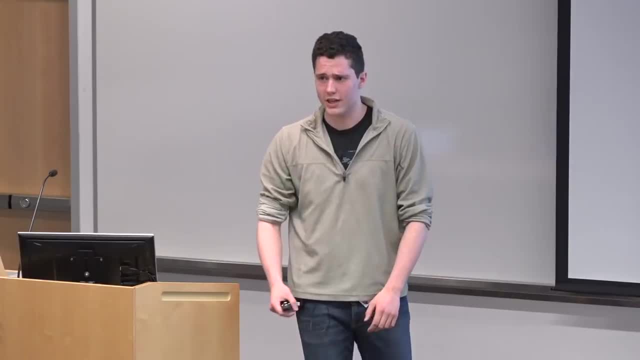 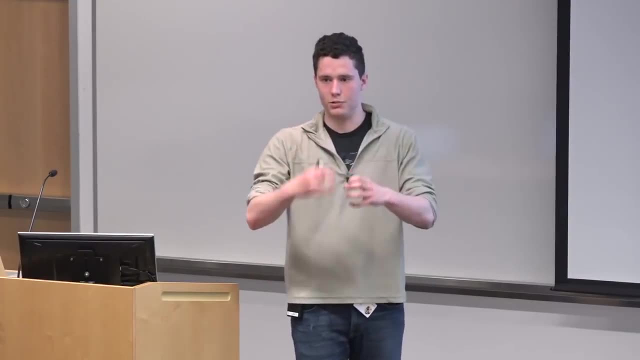 over the trajectory that your agent is going to play in. So trajectory is just: you start some initial state, you take that state, you play an action. you see the next state, you get a reward, then you see that state and then you play another action. 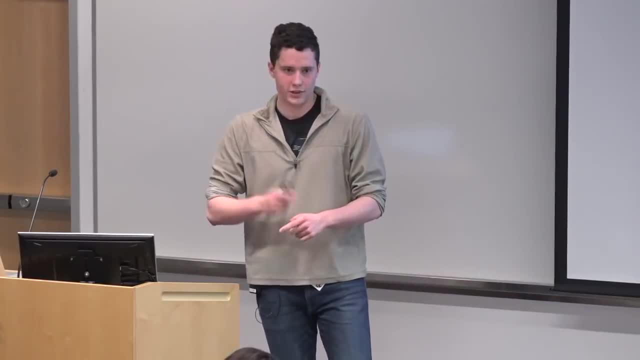 and then you get a reward back and so on, and you just do a state action or a state action reward over and, over and over until the end of your trajectory. and that's one trajectory and you want to maximize the total reward. 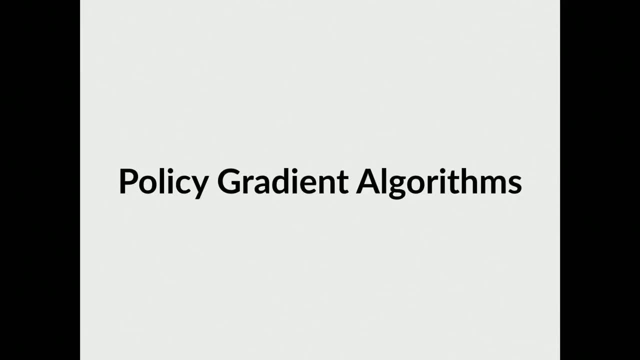 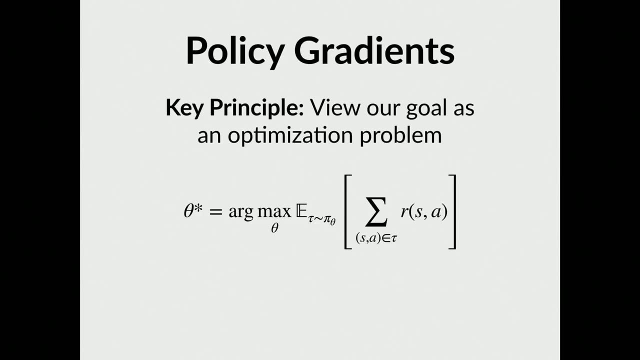 that you see throughout that trajectory. So the class of algorithms that we're going to look at today is all about policy gradient algorithms, whose key principle is that we're going to view this expectation maximization goal as an optimization problem. So this term inside of the expectation- 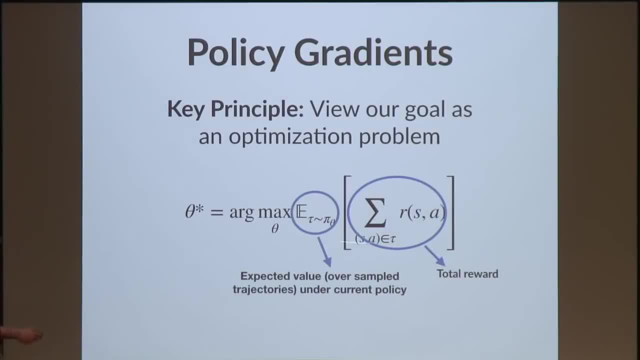 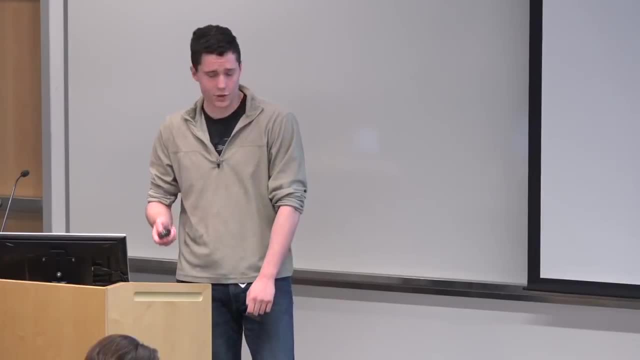 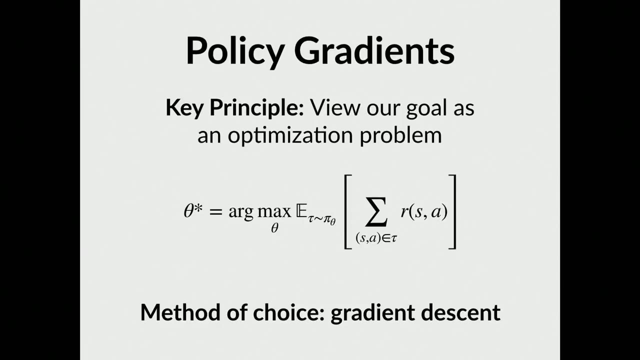 is just the total reward that you get throughout your trajectory, and your goal is to maximize the expectation of the reward that you get while playing the single round of the trajectory, and you want to find the optimal parameters for maximizing this reward, The method of choice that we're going to use throughout. 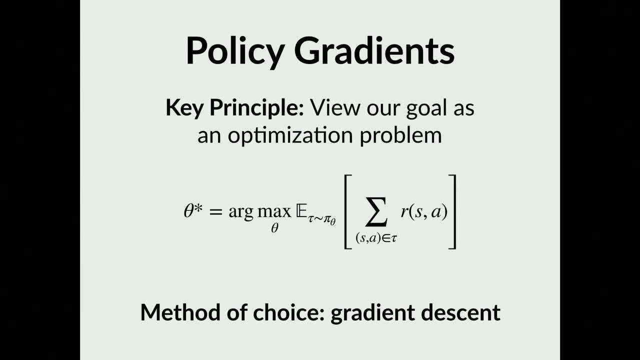 this presentation is just first-order methods to maximize this reward, But the problem is that we don't have any gradient access, and it's unclear exactly how we're going to get the gradient from this expectation, and so what we're going to do instead is we're. 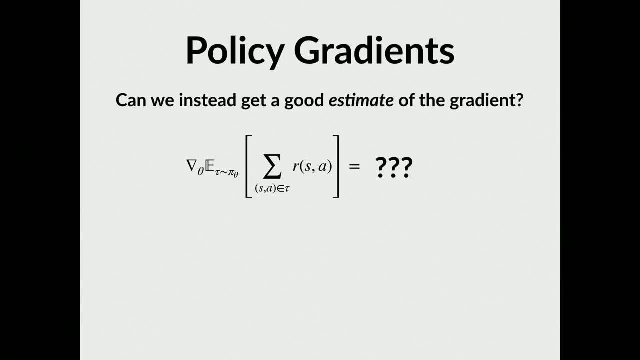 going to try to find an estimate of the gradient It turns out- I'm not going to go into the details here, but it's pretty common in literature- You can basically model this expectation as the expected value of a variable that's easily computable given a trajectory. 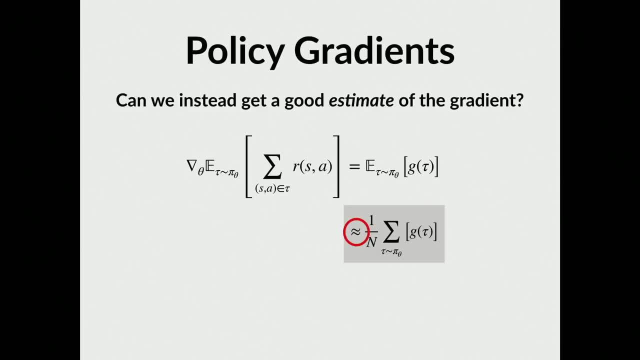 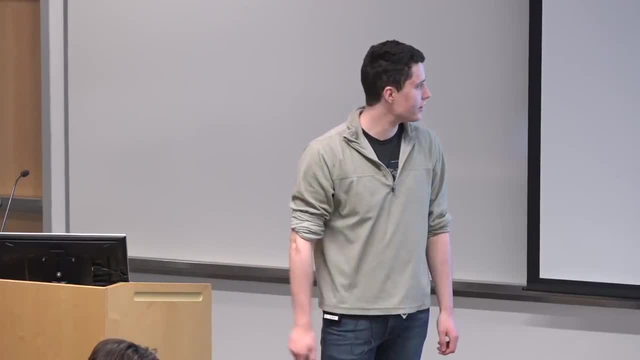 So what you can do here is you can just take a finite sample approximation and you can take a bunch of these gradient estimates, average them together and hopefully get something that looks like the actual gradient which we're going to analyze later. Then, once we get this gradient estimate, 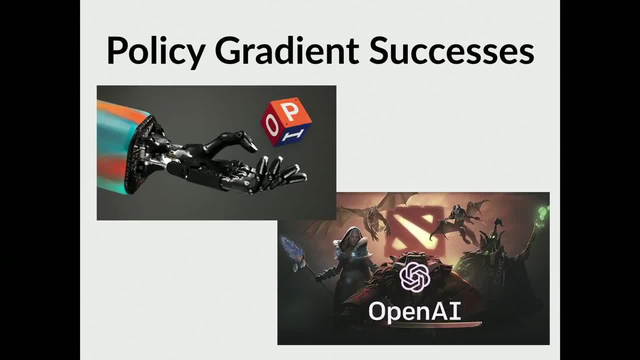 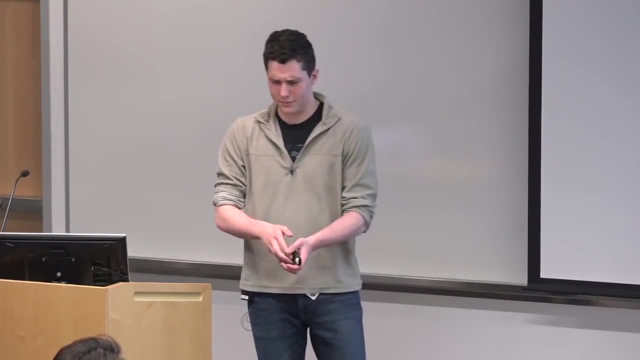 we're going to use it in the gradient descent. People have been really successful at using these in practice. There's OpenAI, who has done both, OpenAI 5, which can be professional humans at Dota using policy gradient algorithms, and they have some robot where you can put a cube in it. 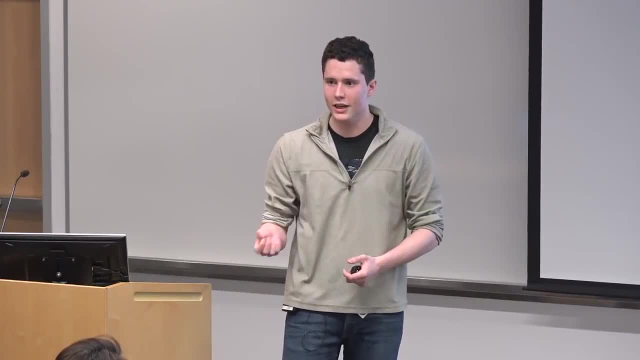 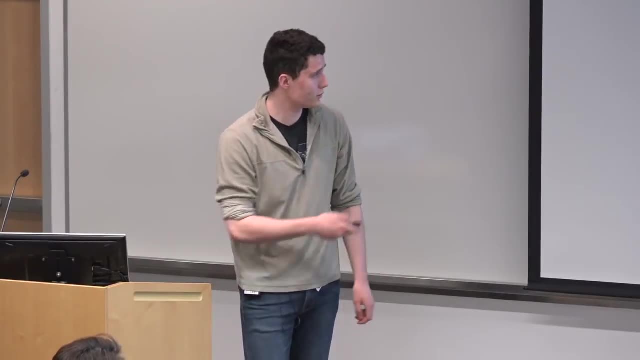 and then you can say, oh, I have a cube in one orientation but I want to move it to another orientation, and then it'll handle it a little bit to be able to shift the cube's orientation, and this works pretty well in practice. 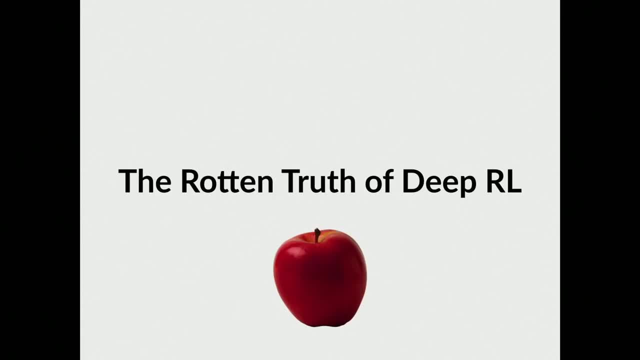 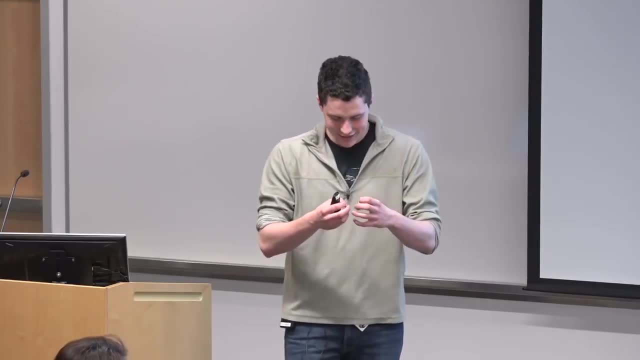 But it turns out that, just like a rotten apple, it might look great on the outside, but there's all these underlying problems. So when you bite into an apple that's rotten, it looks good, but then you bite into it, it's a little moist and juicy, maybe a little brown. 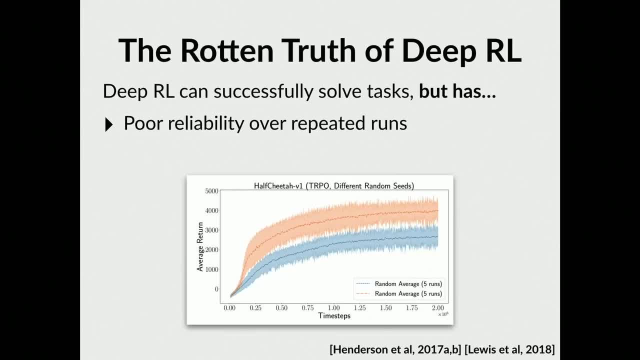 You don't want to eat that Just like that. you probably also don't want to do deep reinforcement learning, because it's really annoying, and I'll tell you why. So one reason why it's pretty annoying is because there is super poor reliability over a repeated run. 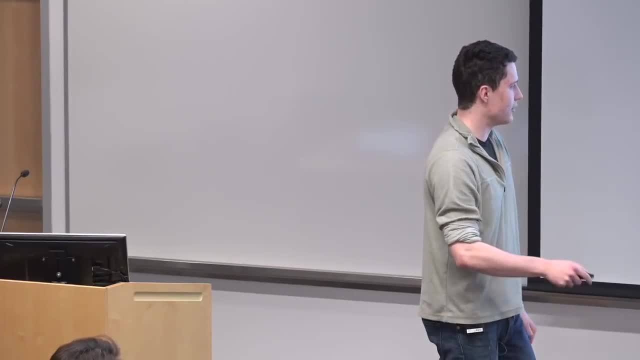 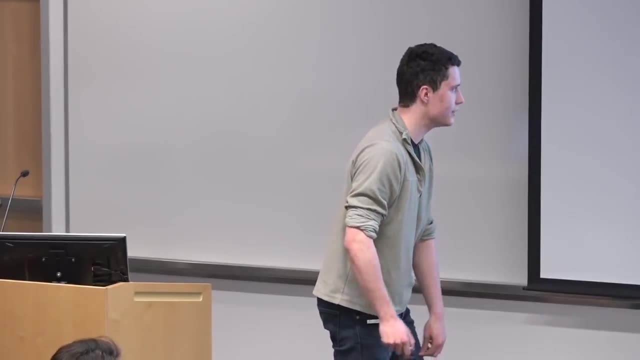 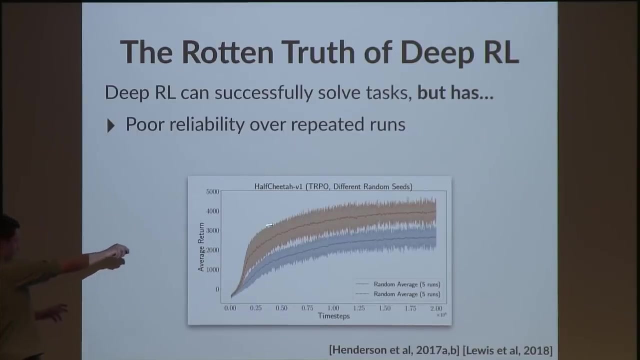 So this is the same game with the same algorithm, and this corresponds to time steps, This corresponds to the return that you get at each step of the time step, and the only difference between these two clusters is that. so this line represents five random seeds. 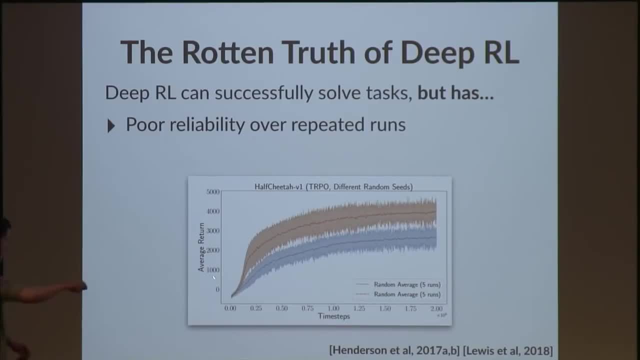 You start at a random seed, then you play the algorithm. So this represents five, this represents another five. They look like totally different algorithms, even though it's the exact same algorithm. The only difference between these two clusters is the choice of five random seeds. 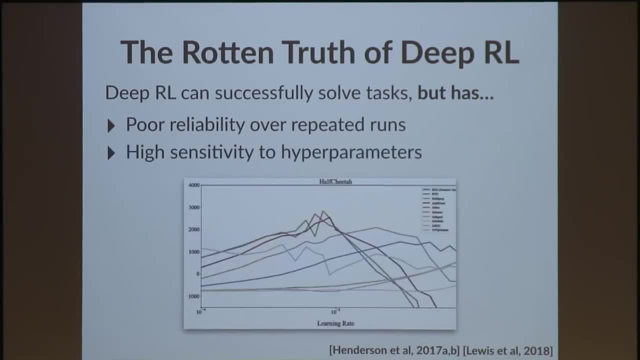 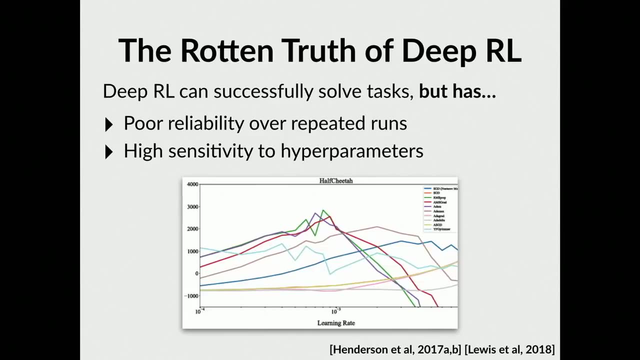 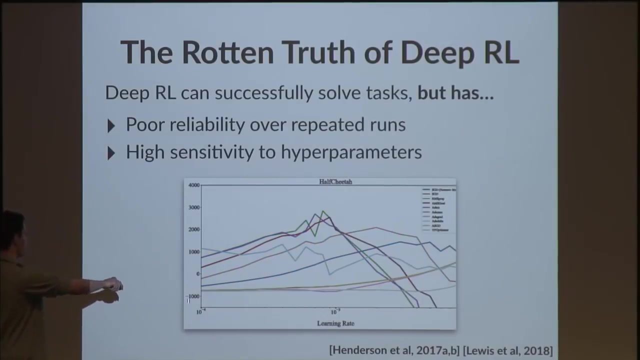 So we clearly have pretty bad reliability over repeated runs. Oh, okay, No, we are good, We're good, Okay. Another problem is super high sensitivity hyperparameters. So this is: the x-axis is going to be learning rate, it's logarithmic- and the y-axis is the total word that you get. 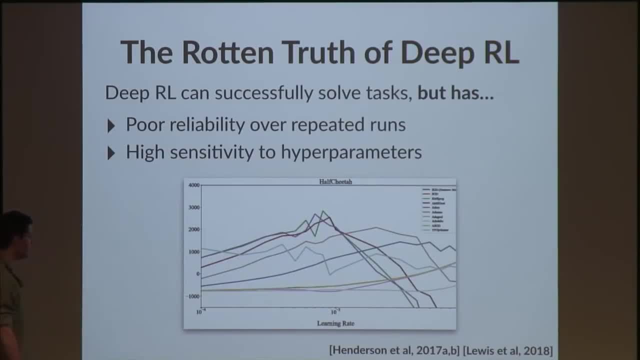 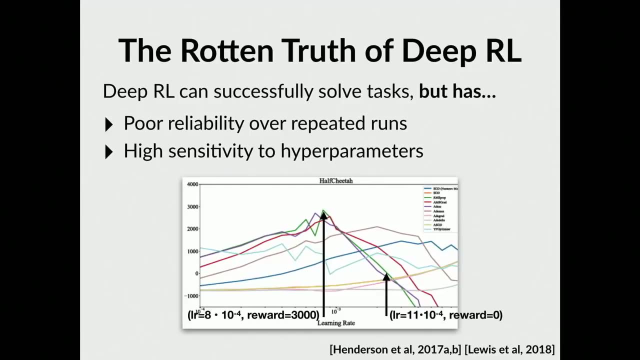 Each one of these lines represents a different algorithm that you use to train the agent, but we're just going to look at this green one, which ultimately achieves the highest reward possible. So you can see that, at learning rate 11 times 10 to negative four. 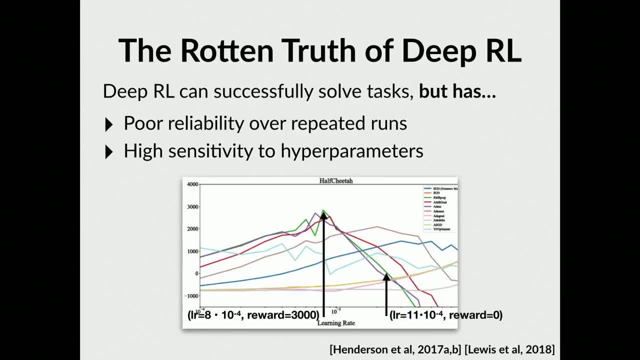 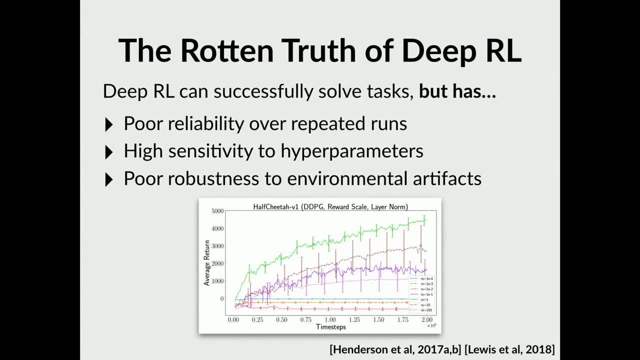 you get reward zero At learning rate. eight times 10 to negative four, you get reward 3,000.. That's crazy, isn't it? It's super high variance just based on this tiny little change in learning rate. Then the final issue that we have: 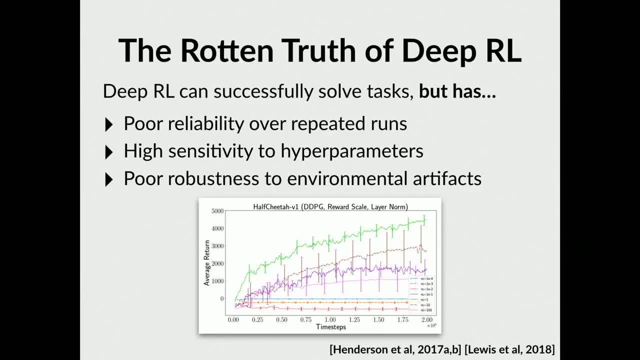 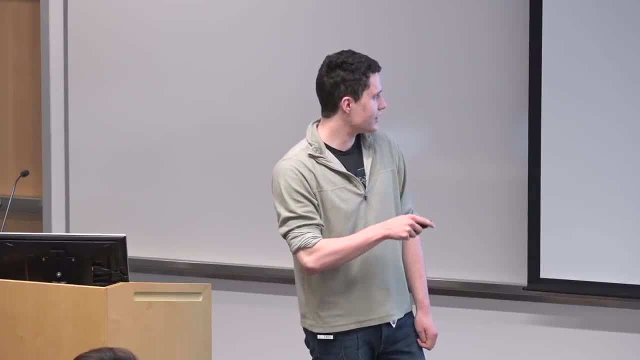 well, there's a lot of issues, but the final issues that we have been discussing in this slide is the poor robustness to artifacts. so one example is that you have the same game again and we're just going to scale the rewards at the very end by a constant factor. 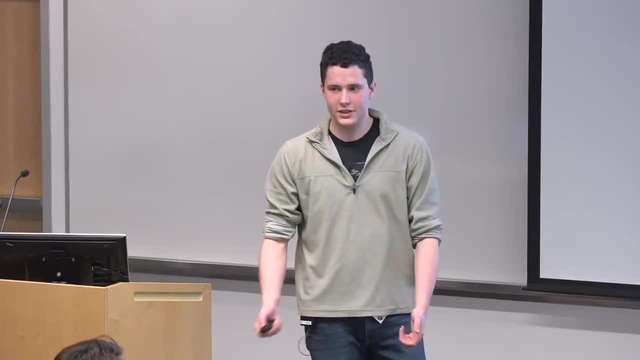 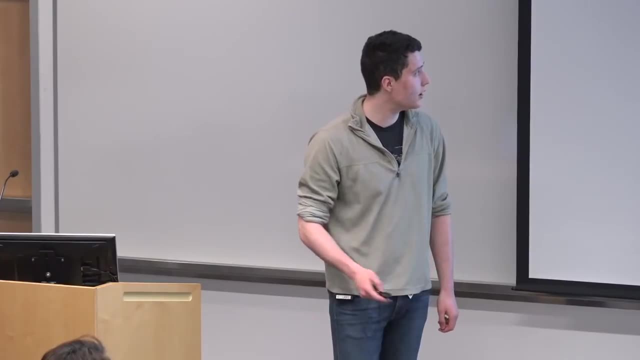 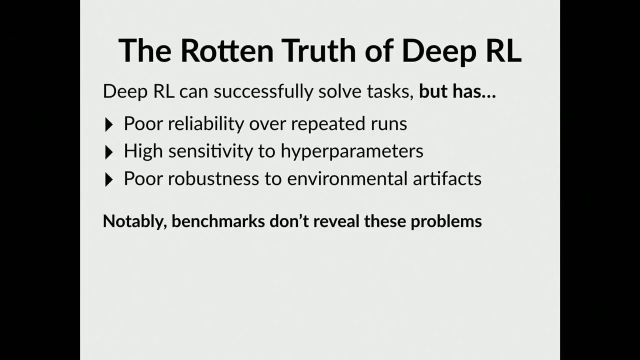 Each one of these represents a different constant factor. They should all have the same ultimate reward, but because of the reward scaling, they do significantly worse. So it's pretty weird, and so that's another issue with deep reinforcement learning Notably so. the benchmarks that everyone looks at is 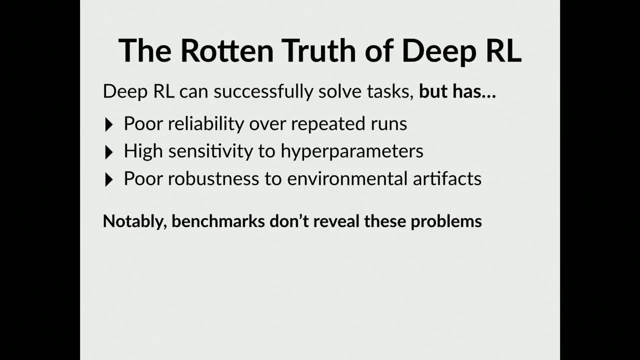 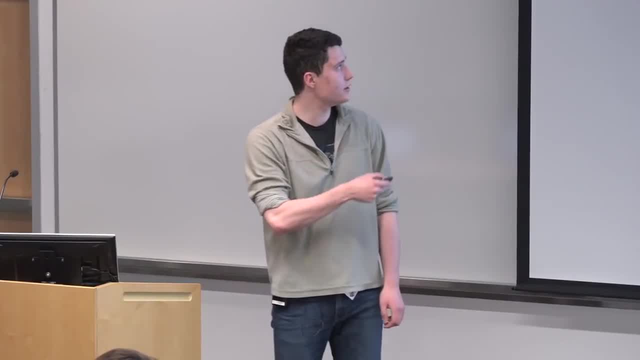 basically, we're going to take the algorithm and we're going to get the highest expected reward at the very end, and that's the benchmarks that people care about. That's the benchmark that people care about in reinforcement learning, and none of these problems are revealed by these benchmarks. 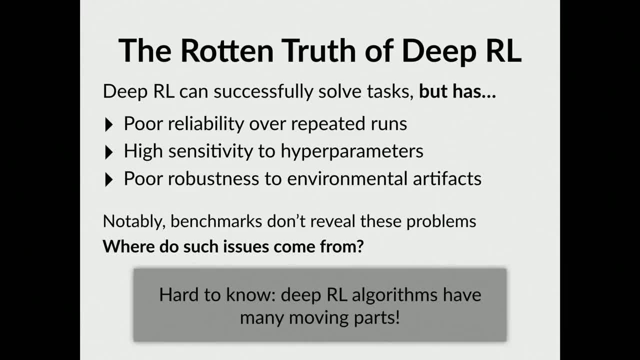 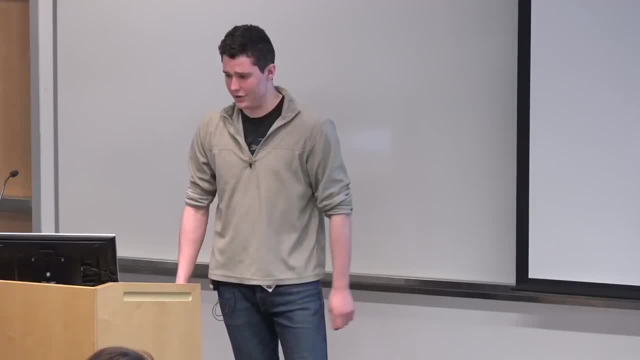 So the question is, where do these issues come from? But it's unclear, because deep reinforcement learning algorithms are super complicated, They have tons of moving parts and it's just very unclear how to implement them, often from just the papers. So one example here is the OpenAI baselines repository. 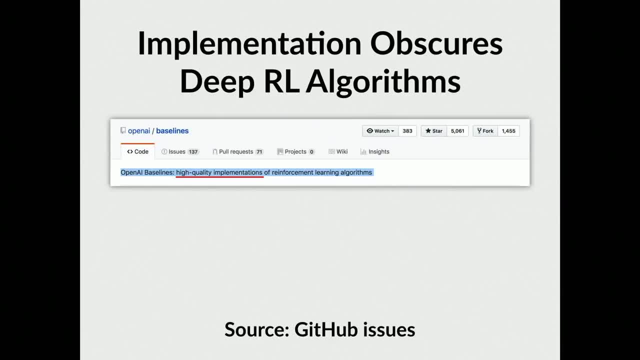 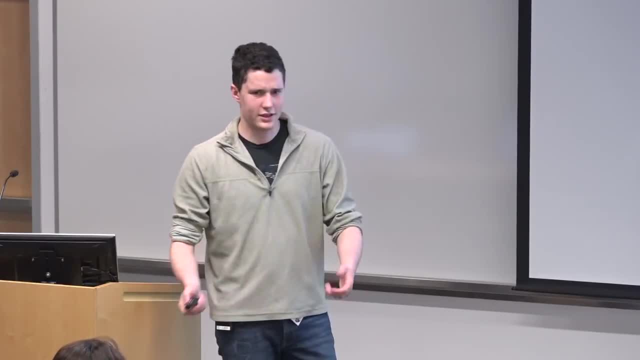 It has high-quality implementations of reinforcement learning algorithms and so, in particular, we're going to look at the PPO1 and PPO2 algorithms, which are from the paper that they have about PPO, which is just an algorithm in deep RL. 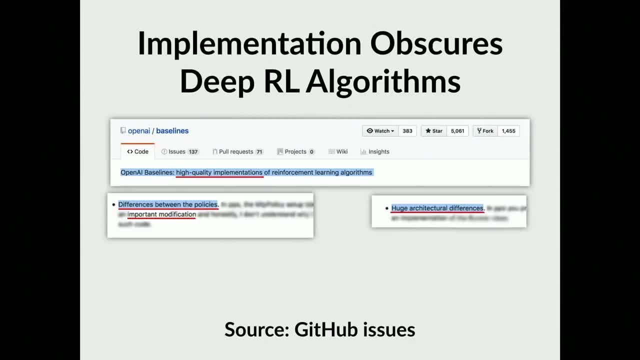 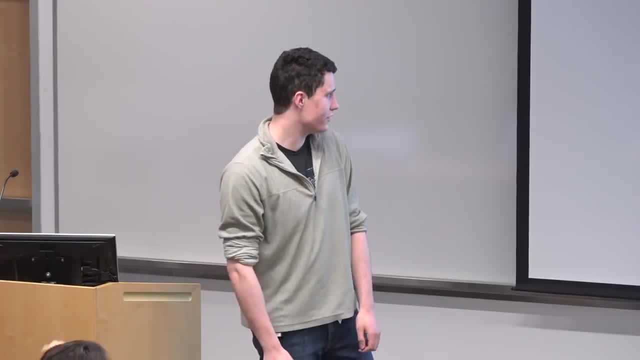 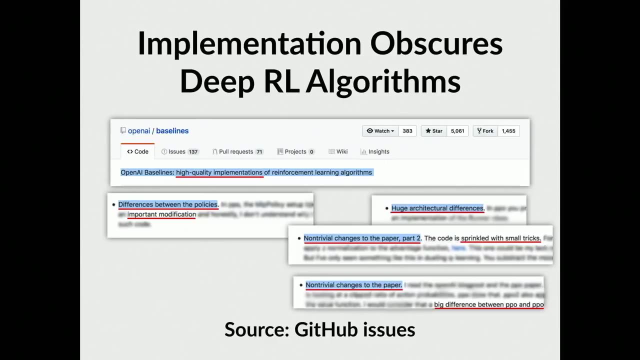 So these are all GitHub issues of people complaining about the differences from the paper and between these two implementations. So between the two implementations there's huge architectural differences. There's huge differences between the policies. They have all these different optimizations on top of the algorithm that they use that they don't mention in the paper at all. 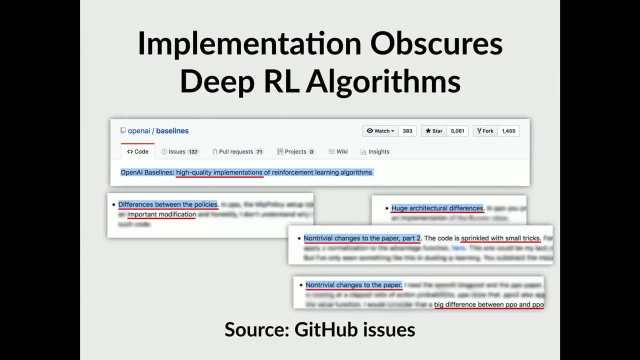 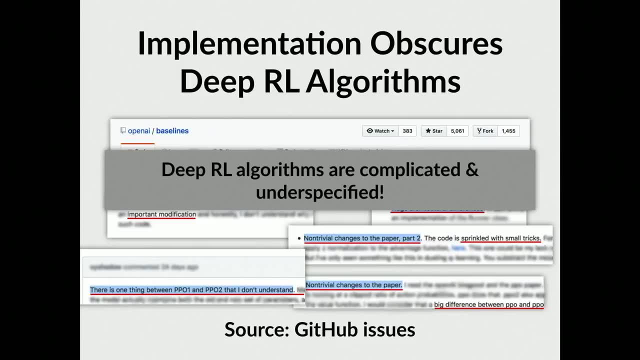 There's like super non-trivial real changes in the repository compared to the paper and so on. So what? the overall message of this slide is that deep RL algorithms are really complicated and they're really under-specified when you just look at the papers. 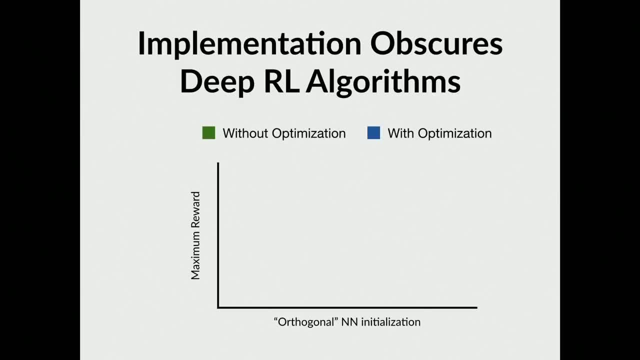 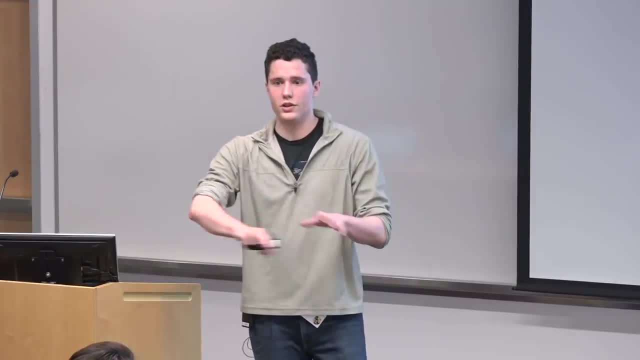 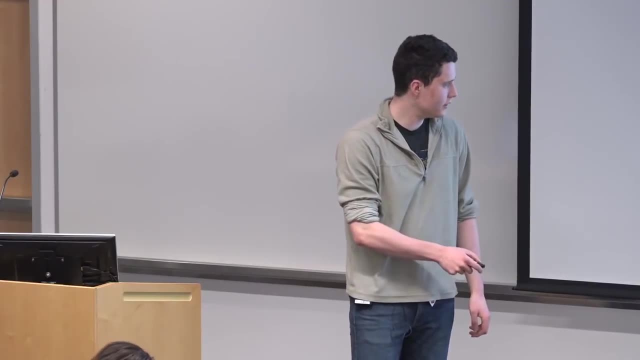 So basically, in PPO at least they have the actual algorithm, they have in the paper, and then they have the implementations, and the implementations have all these different kinds of optimizations on top. One example is orthogonal. oh no, there we go. 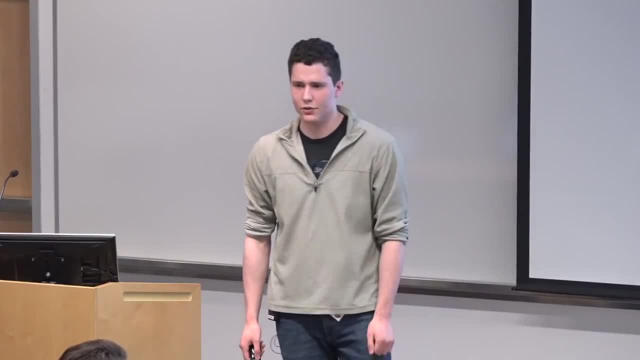 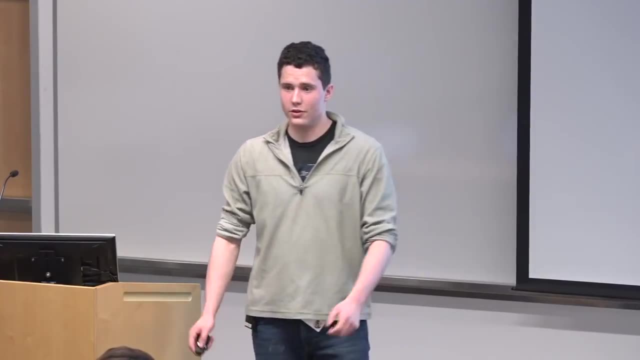 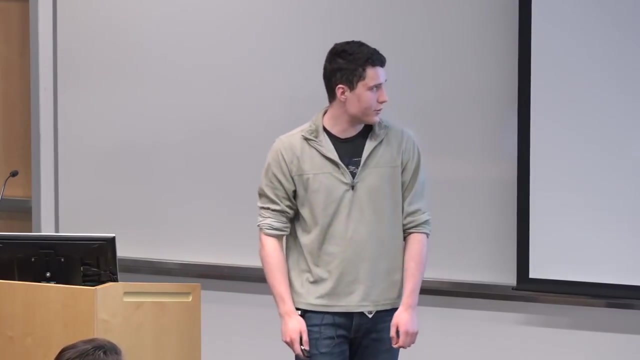 One example is orthogonal neural network initialization, So it's just a different way of initializing the weights. So normally in PyTorch you use like Xavier initialization, which works really well for image classification tasks, But they suggest using orthogonal neural network initialization. 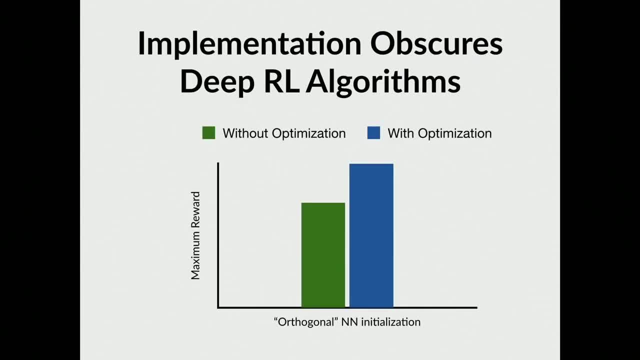 So it turns out that when you run the algorithm using orthogonal initialization, you do way better than Xavier, and it's a little unclear why Even you wouldn't think a priority of this would be a big deal. What task is this? Yeah? 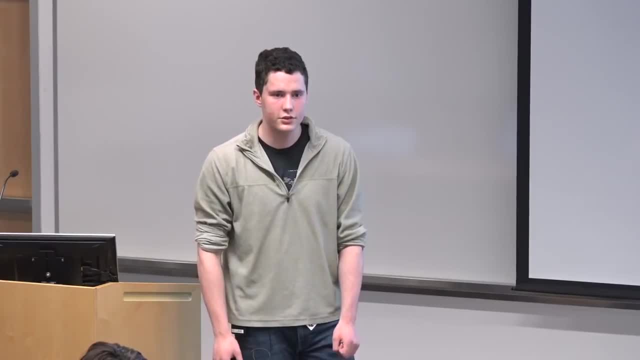 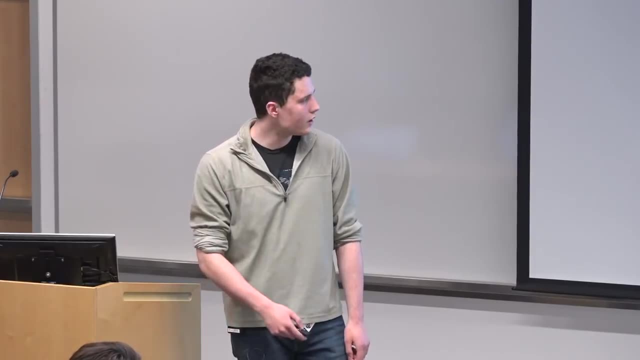 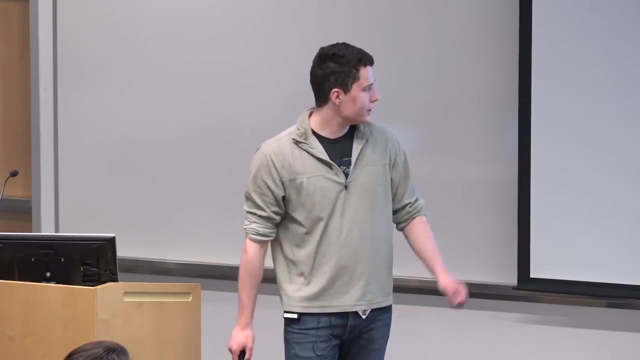 This is Humanoid, Yeah, humanoid, using PPO. So is this stable across different tasks? Yeah, you see the same kind of effects over different tasks. It's definitely more accentuated with harder tasks. So this experiment is essentially that we took all the different optimizations. 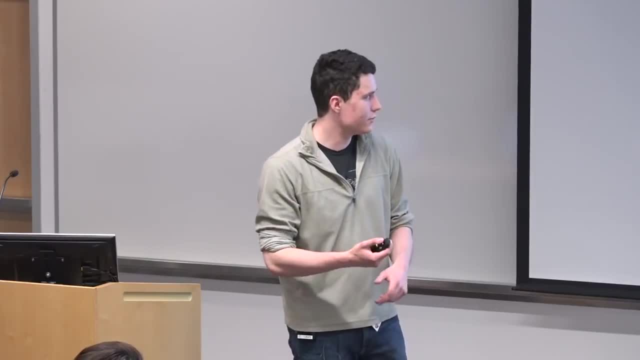 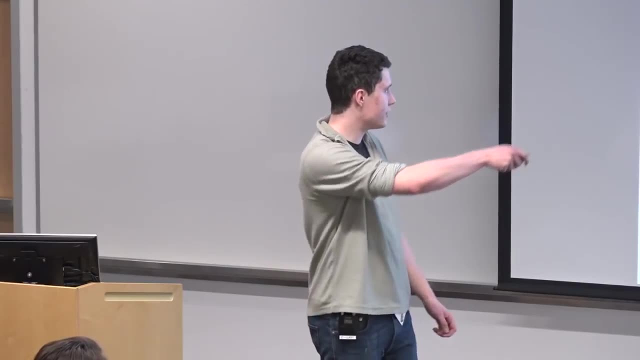 and we did the Cartesian product of all of them and then we plotted the maximum reward for the half of the Cartesian product with this optimization, without the optimization. So it turns out that when you use the optimization, you do way better in terms of the maximum reward. 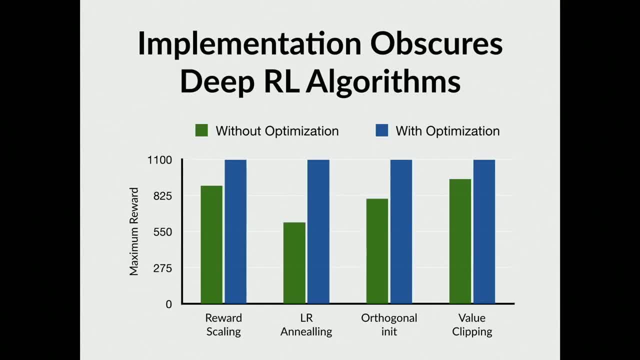 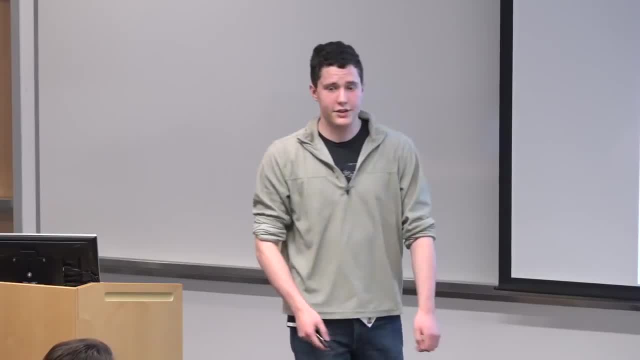 This is true over a bunch of the different optimizations. I'm not going to go into what all these optimizations actually are, But when you look at the maximum reward for all these different optimizations, with and without, they're drastically different. By the way, these are not even listed in the paper. 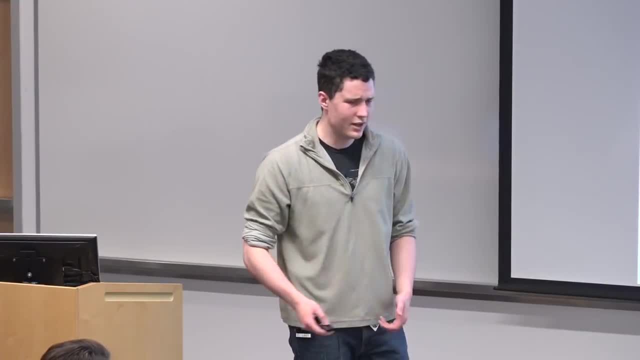 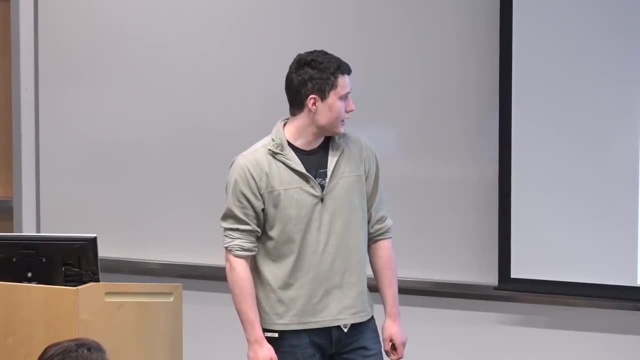 because that's how unimportant the authors originally thought that they were, that they're very common, But people clearly have a very hard time in re-implementing these algorithms because it's often unclear what's exactly part of the deep RL algorithm that they present. 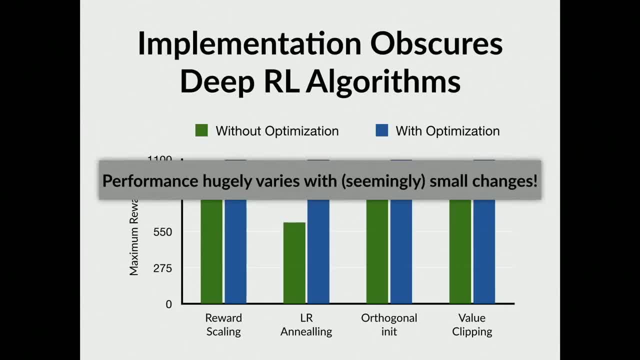 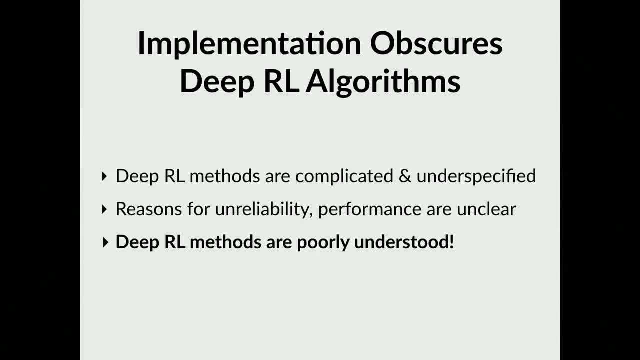 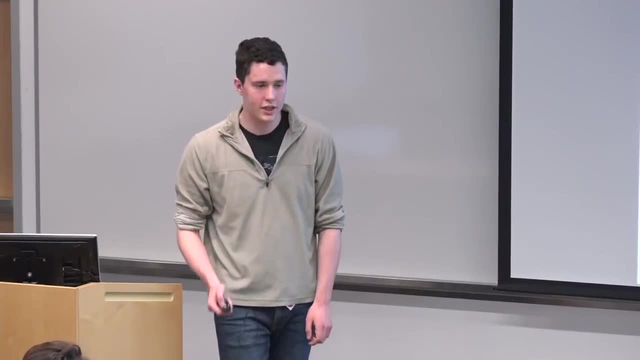 and what's just another optimization on top. So even with these seemingly small changes, performance can super widely vary. So the overall takeaway here is that these deep RL methods are underspecified and they're really complicated, and the reasons for unreliability and performance are somewhat unclear. 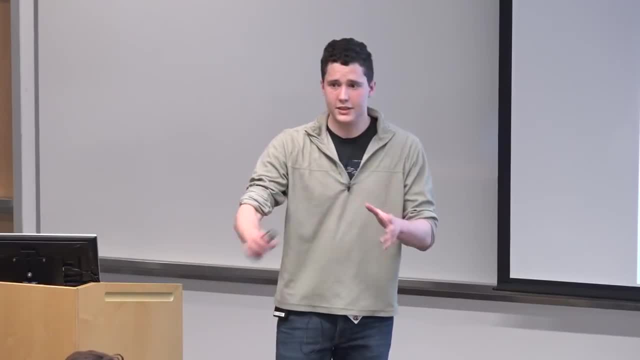 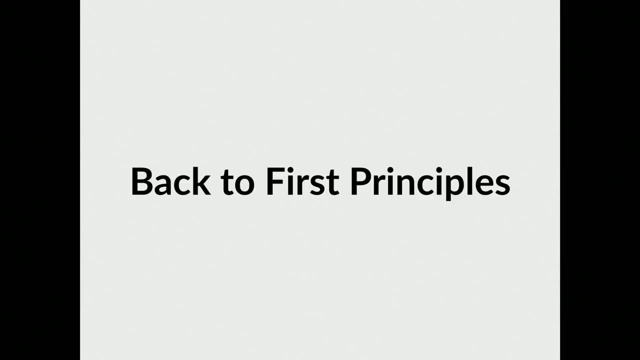 It's not sure if it's the algorithms or if it's all the little optimizations that they put on top of them. So this calls for us to go back to a first principles: look at what these algorithms are really doing. To do that, we're going to look at a bunch of 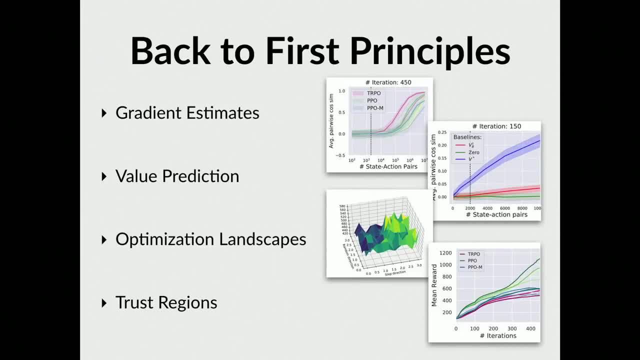 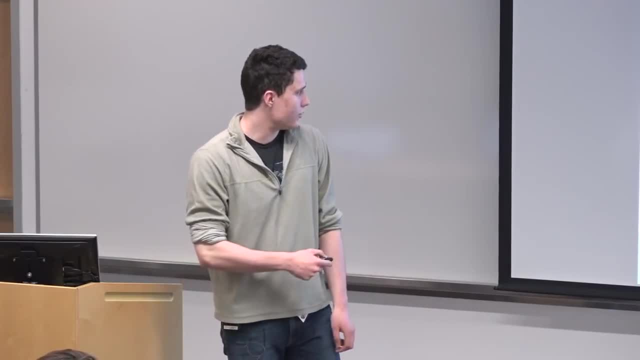 different tenants of the policy gradient framework, One of which is gradient estimates. I'm going to explain all of these as we go, So I'm just going to go quickly through them. Another one is value prediction. We're also going to look at optimization landscapes. 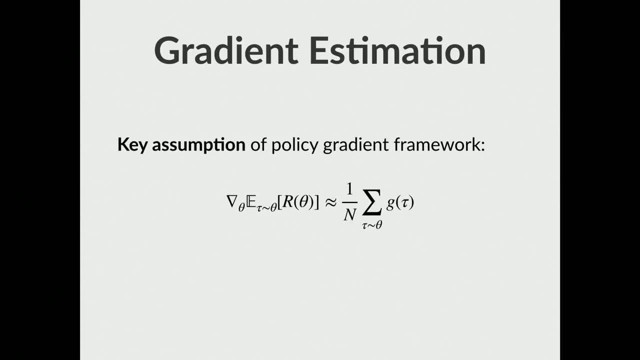 and finally, we're going to look at trust regions at the very end. So the first thing we're going to look at is gradient estimation. So, if you recall, in our policy gradient framework, one of the key assumptions that we have is that the gradient that we actually take is pretty correlated. 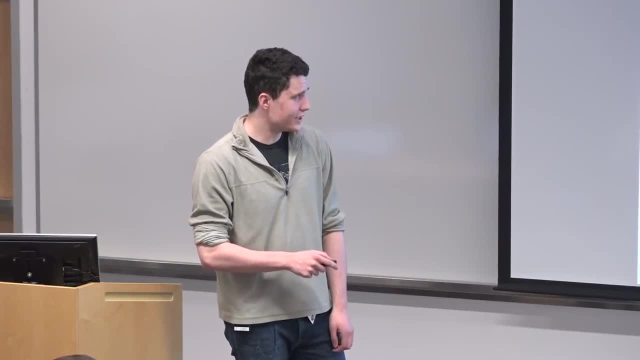 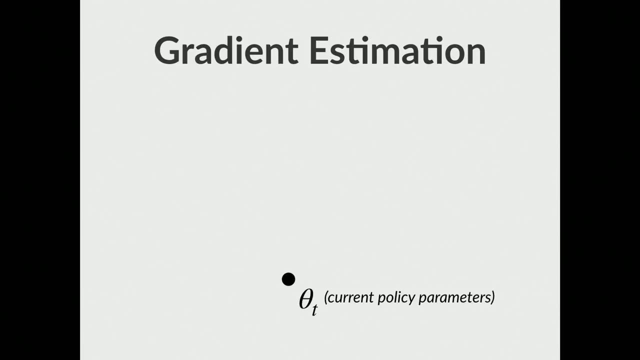 or at least correlated with the finance sample approximation that we get. We want to look at how valid this is in practice. So the experiment that we're going to do is that we're going to fix a single policy and then we're going to take a bunch of steps. 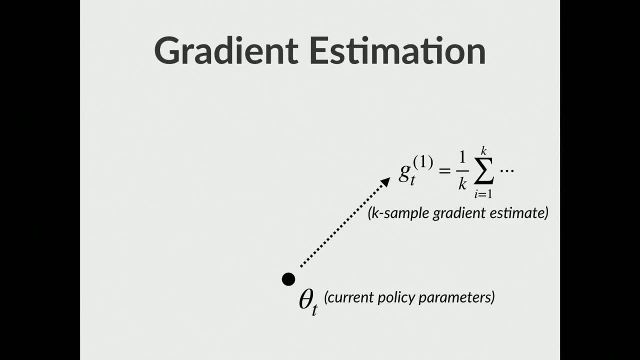 each of which uses this case sample gradient estimate. So we're going to take a bunch of samples and then we're going to make a step based off of the sample. So you should expect that if you have more samples, your gradient estimates are going to get better. 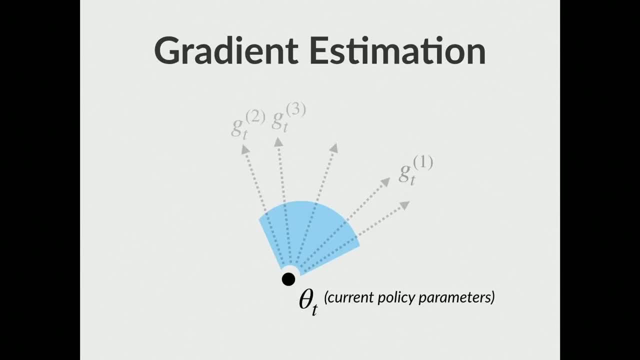 We're going to do this a bunch of times and what we want to be able to do is measure their concentration and see how well these actually concentrate to the true gradient. The way we're going to do that is we're going to measure. 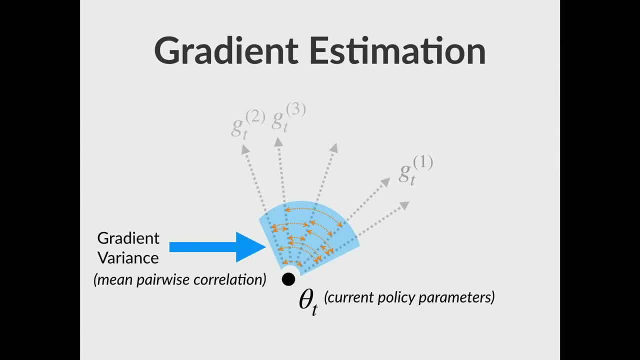 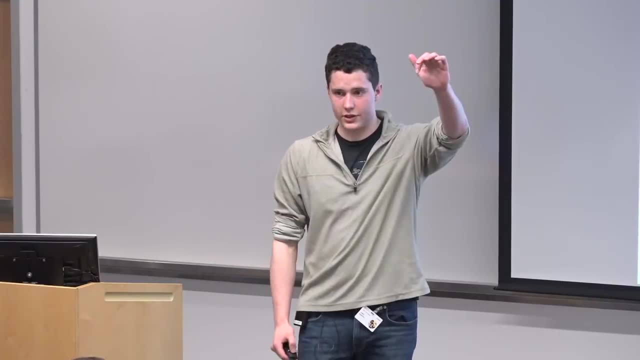 the mean pairwise correlation between all the different gradients, between all the different gradient estimates that we collect. So you can think of this as if you have higher pairwise gradient correlation, you're going to have better concentration. If you have lower mean pairwise correlation. 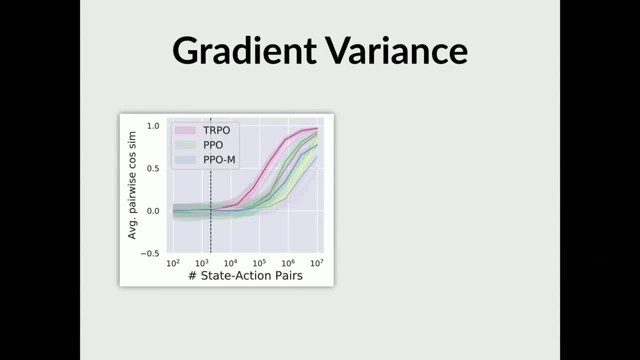 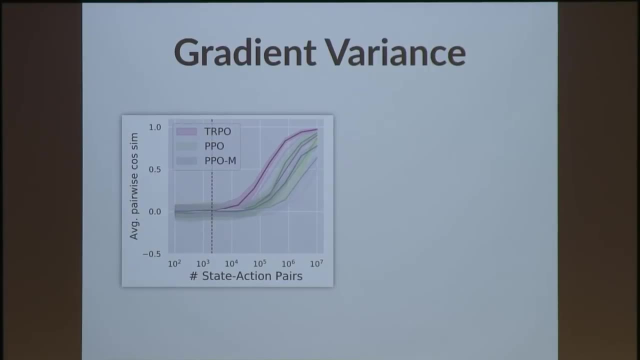 you're going to have worse concentration. So this is a plot where on the x-axis you have the number of samples that we use and on the y-axis we have the average. basically just the correlation- sorry, the concentration in that regime. 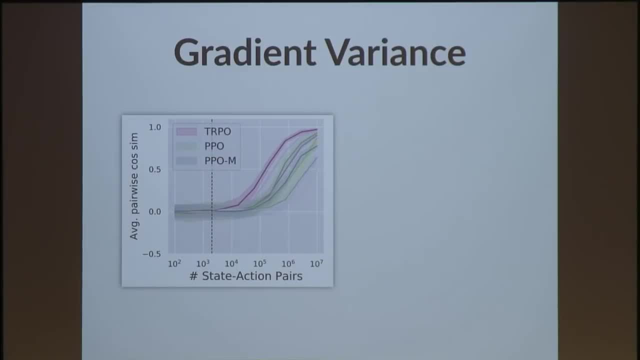 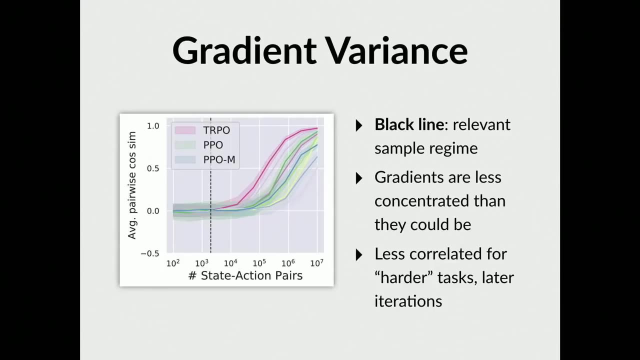 So higher means that you're basically concentrating to get the actual gradient and lower means that you're not as much. So this black line is what the algorithms actually use in practice. So you can see that roughly- I don't want to say half, but like about half the time. 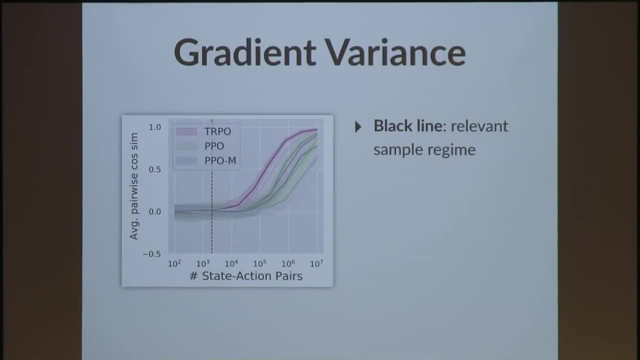 a little less than half the time. the steps that you take are actually in opposite directions from one another and the gradients are much less concentrated than they should be. But that's not necessarily as big of a problem as you might think, because in high dimensions 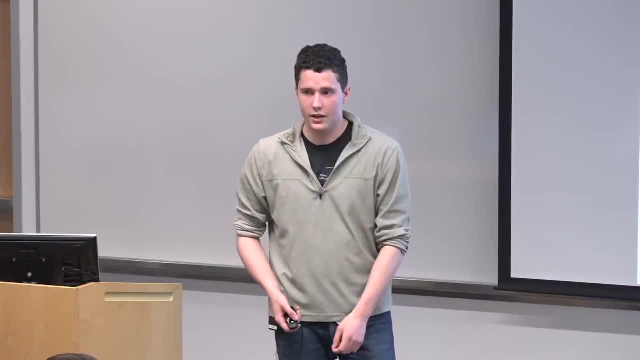 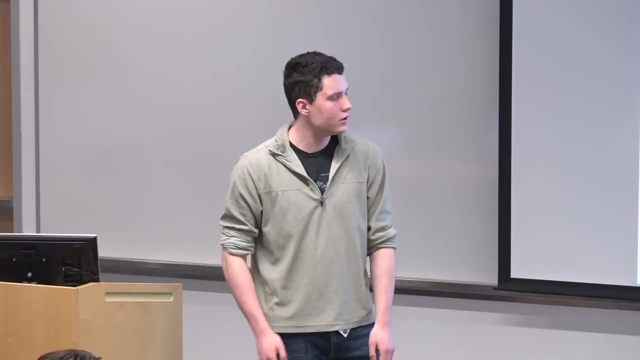 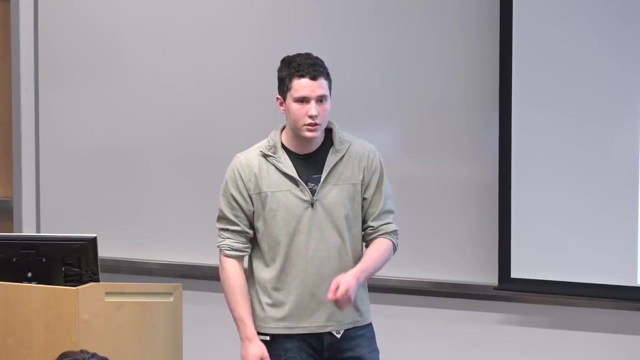 if you have very low cosine similarity, it's still pretty significant because you're in high dimensions. The x-axis is like you're changing the state, action space, So the x-axis is the number of samples that we use. Oh, okay, So you would expect yeah. 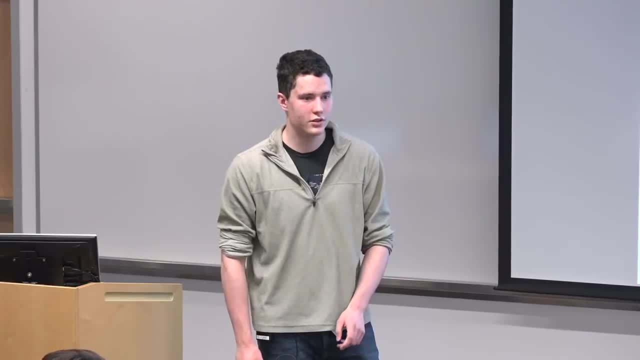 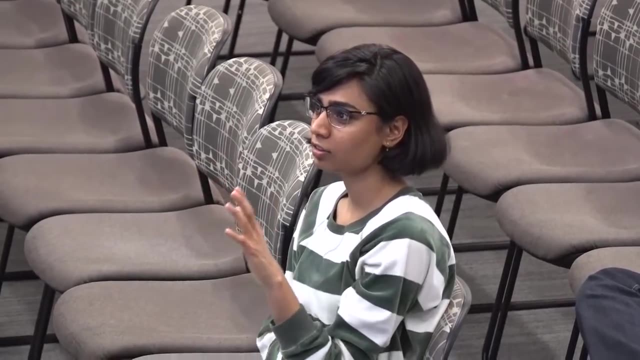 You can finish your sentence. Oh, no, no, no, Okay Is this- You can just ask. if you guys are confused, just ask a question: Is this consistent? Is it across different architectures of the policy? So we only tested one architecture of the policy. 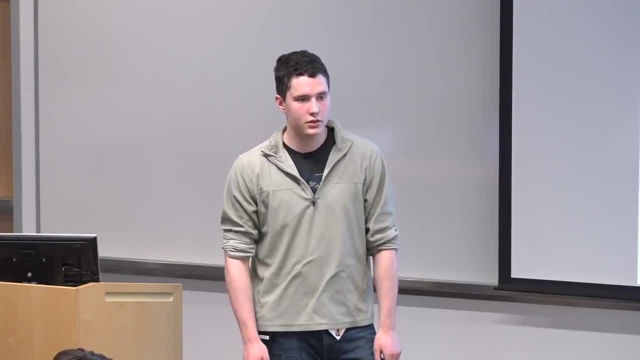 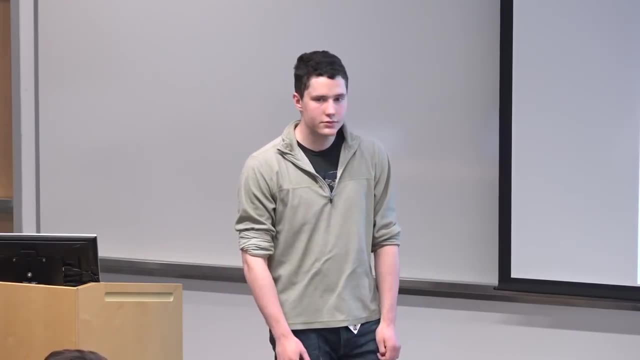 But if I had to guess it, I think it would be: It's consistent across tasks, for instance. Yeah, it is very consistent across tasks, across different iterations, yeah, So in this case, what's the dimension of the parameter? 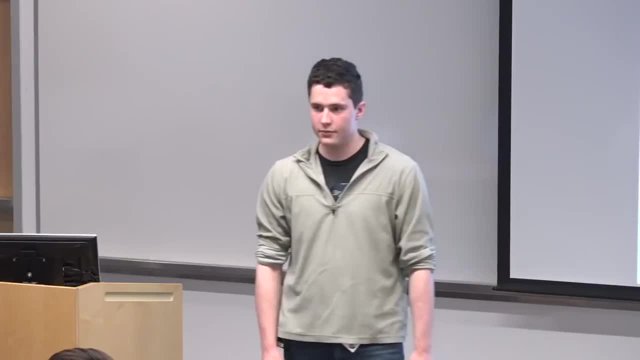 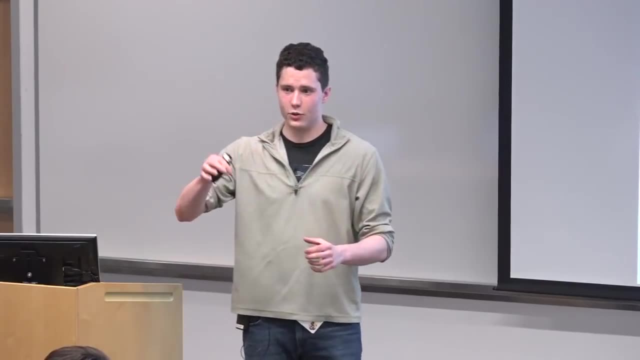 What's the dimension of the parameter? About 5,000.. So if you consider like random Gaussians and then you have correlation between the random Gaussians, it was like you get roughly like one over square root D correlation like cosine similarity, I guess. 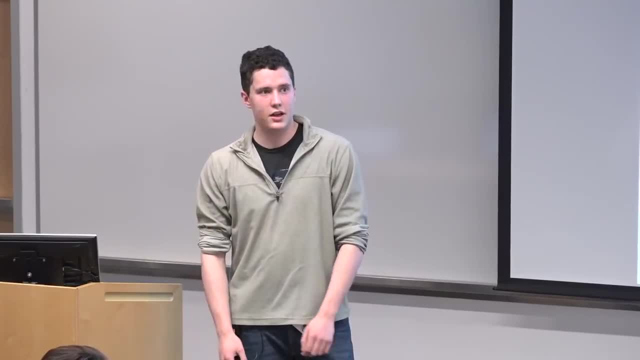 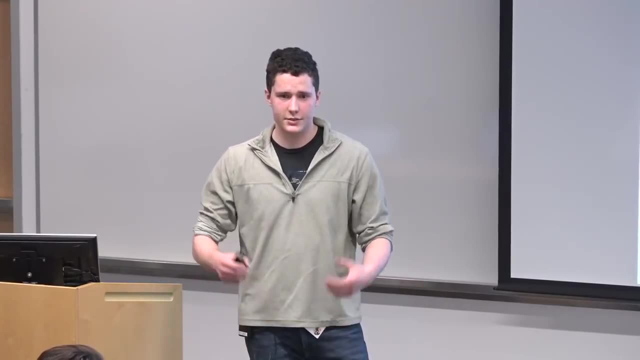 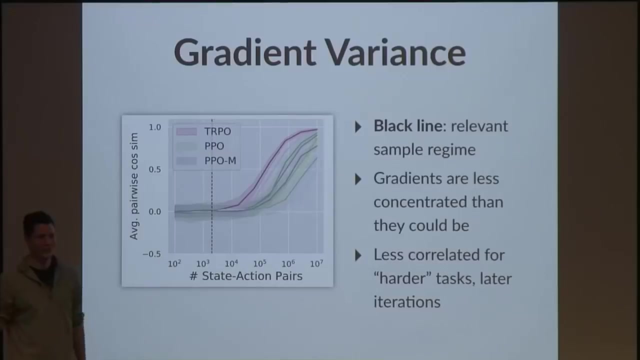 between two random Gaussians. So you get like, I don't know, maybe 0.01 or less than that in terms of correlation, if you just drew Gaussians and 5,000 dimensions. So this is non-trivial and Alec pointed this out. 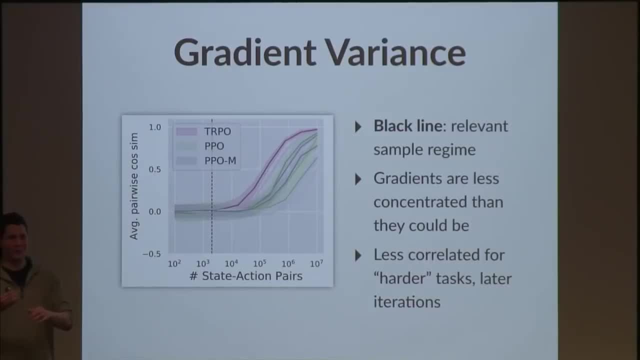 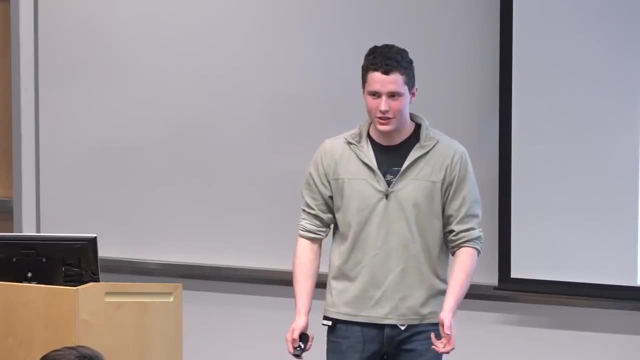 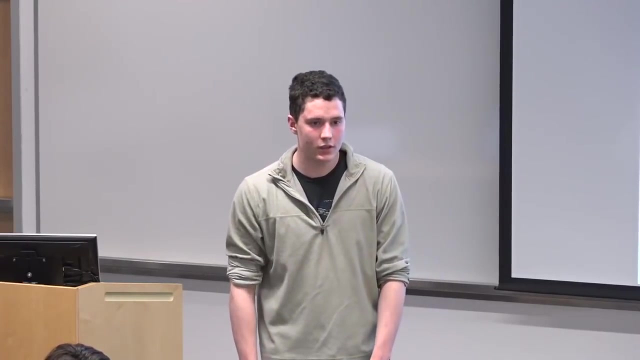 Well, Alec, multiple people pointed out similar veins. Never mind, But anyway, Yeah. Yeah. So it's not quite as bad as it looks, but there's clearly a lot of room for improvement here. How does it vary across the equations of the optimization algorithm? 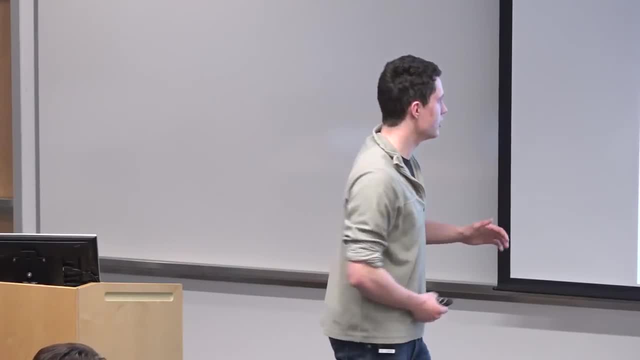 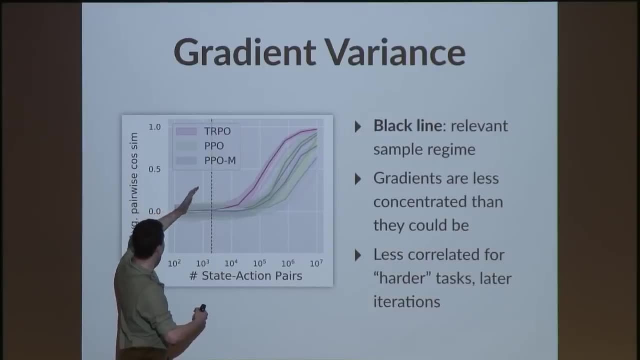 Yeah, So at earlier iterations this looks much better. So if you're at the very start, this graph basically just shifted left, and so you get actually pretty reasonable correlation at the very first iteration. Then I think there's like iteration 150 or so out of. 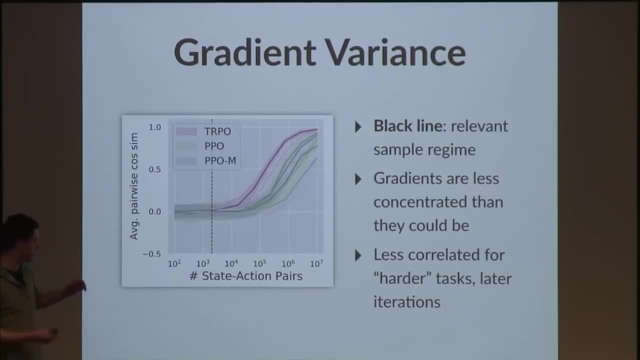 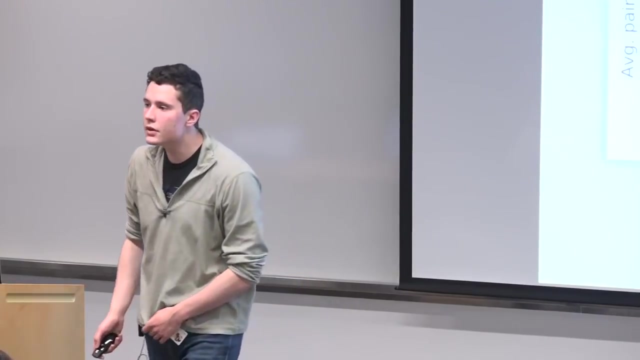 500 or 300,, but it very quickly drops off. So as you go further in the iteration process, this graph shifts to the right and you get much worse estimates in terms of concentrating Any other questions by this way. What do you mean? harder tasks? 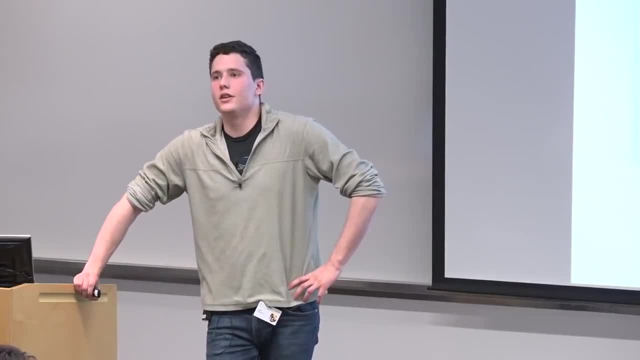 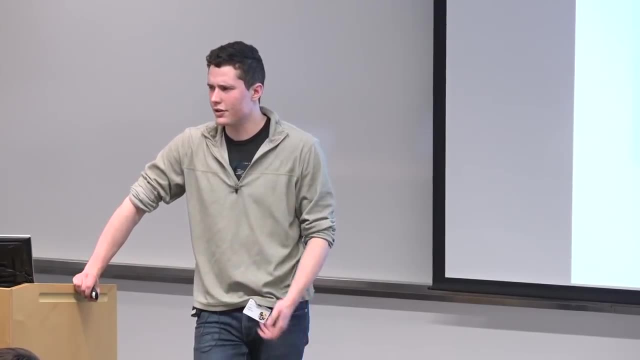 Harder tasks. Yeah, So there's an informal hierarchy of how hard all these different tasks are. I guess you can make it more fun, Typically in terms of sample complexity- how many samples you need to be able to learn this task. 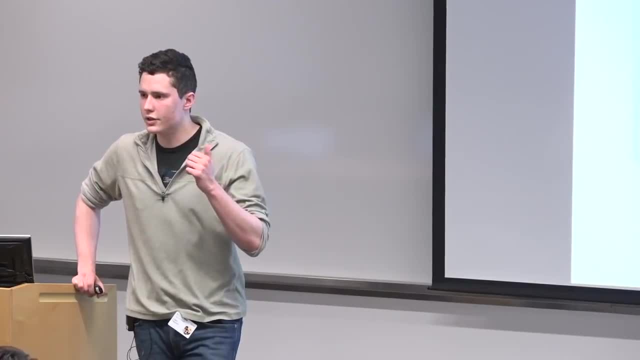 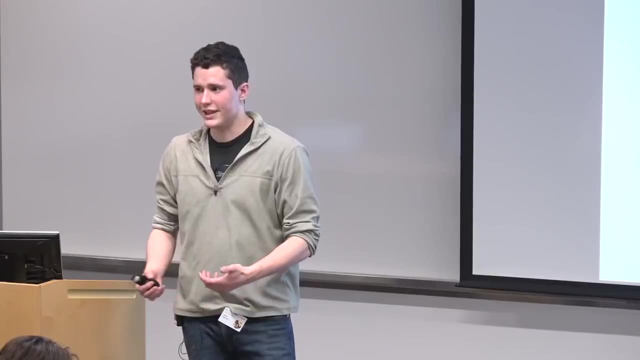 So this is for a humanoid or this is for- sorry, for Walker2D, which is considered one of the harder tasks on MuJoCo. Then there's easier ones, like Hopper, where it's like it's going around like this: 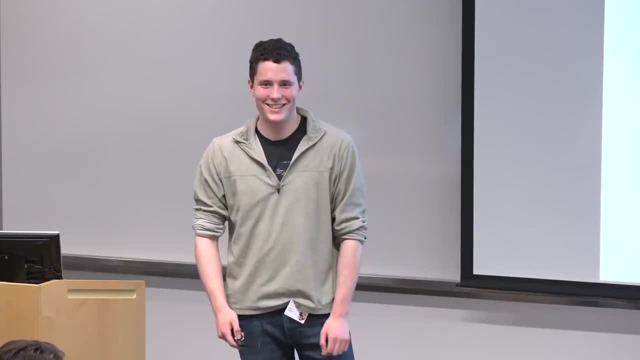 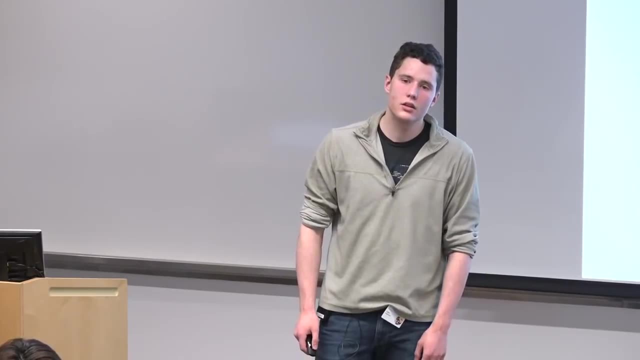 For some reason, that's easier. Yeah, Can you give some sense of how bad this could be? Are these doing much better than the worst case scenario, or Yeah, Actually, we're going to get to that in the next section. Okay, 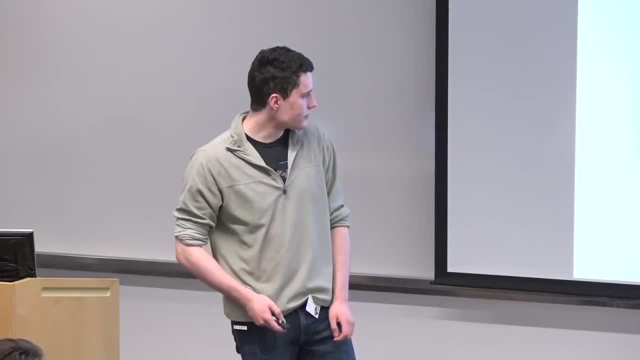 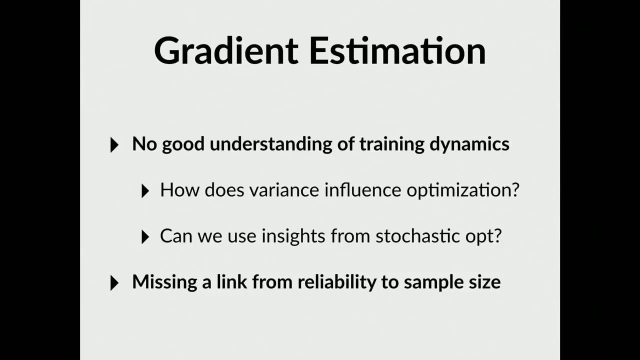 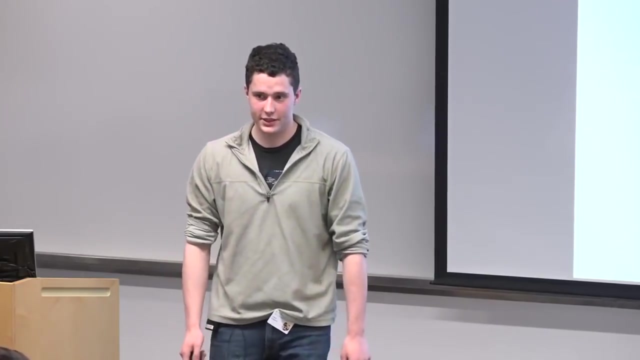 Yeah, We're going to look at value estimation. So I guess the key takeaway here is that we don't have a great understanding of the training dynamics for how this variance really impacts our optimization process. But it would be great if we could use insights from stochastic optimization to be able to look at this. 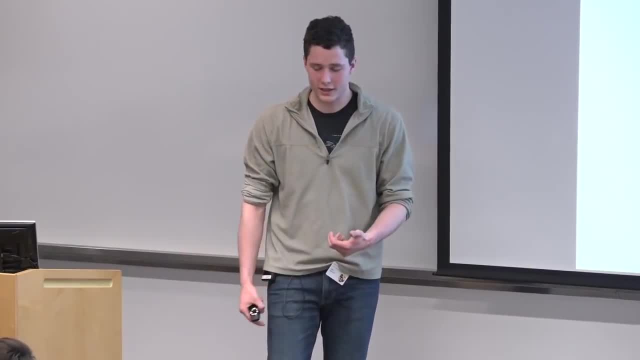 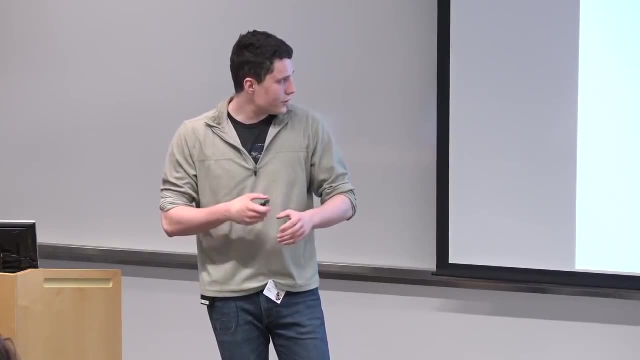 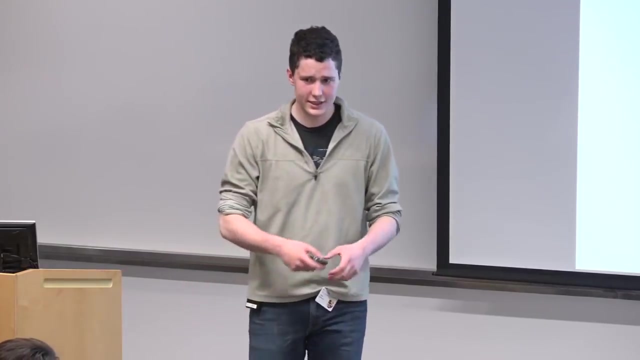 It's not exactly the same regime because the samples that we get are not exactly. they aren't independent. and not only that, but the actual objective, because of the way that the deep policy gradient methods are organized, is non-stationary, So you can't exactly apply SGD. 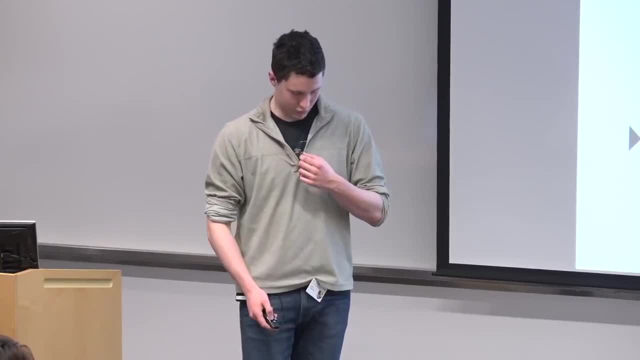 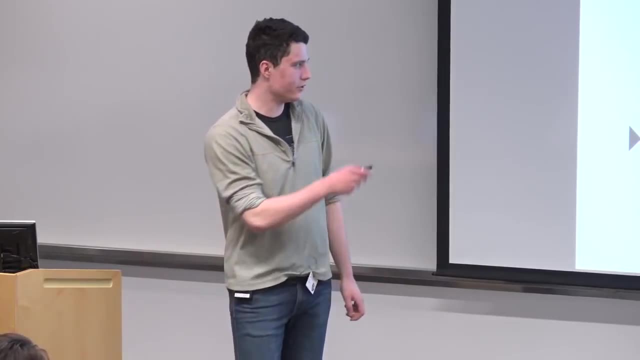 but it would be great to use insights from it. Okay, No, So yeah. and another key thing here is that we're really missing a link between reliability and sample size. So it turns out that when you really scale up these algorithms and use many more and more samples, 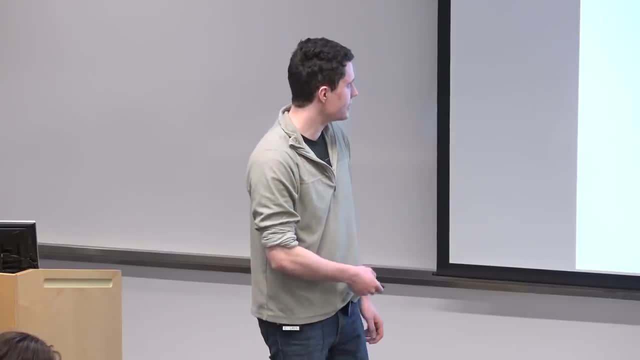 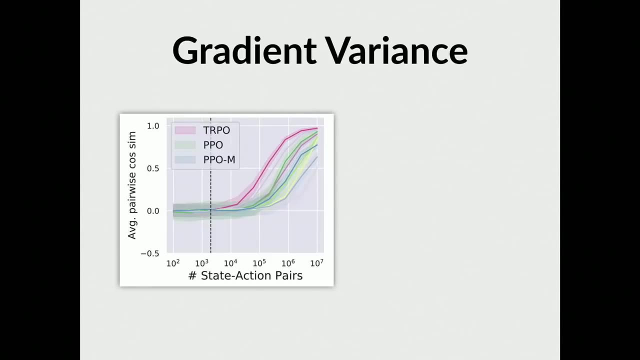 these algorithms become much more reliable. It hints at this in this plot because, you can see, the gradient estimation is much better when you use many more samples, So it'd be great to get a better understanding of what that's like. There's actually an open eye paper about that. 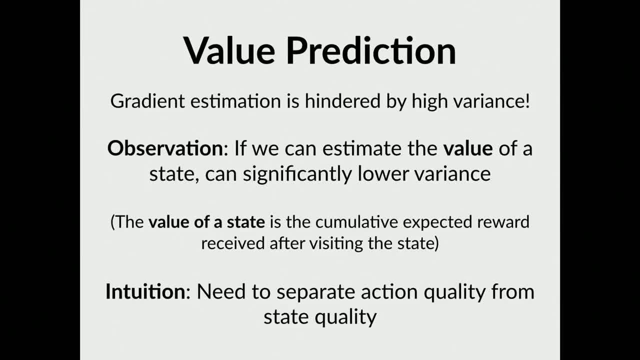 but it would be great to look into it even more. So the next aspect of policy gradient methods that we're going to look into is value prediction. So, as we just saw, the gradient estimation that we get is really hindered by in terms of concentration. 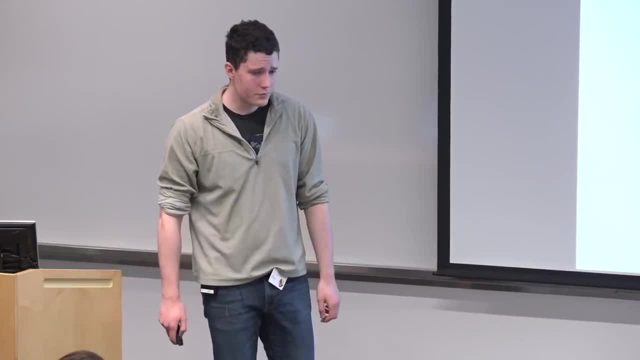 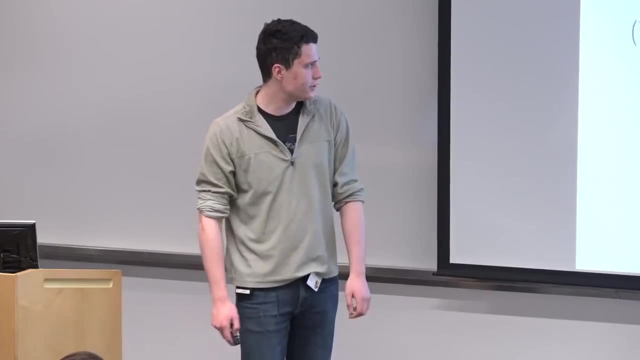 the concentration that we get is really hindered by poor variance, So it'd be great if we could lower this variance. It turns out that one way to do that is to estimate the values and then use that in our policy gradient method. So the value of the state is 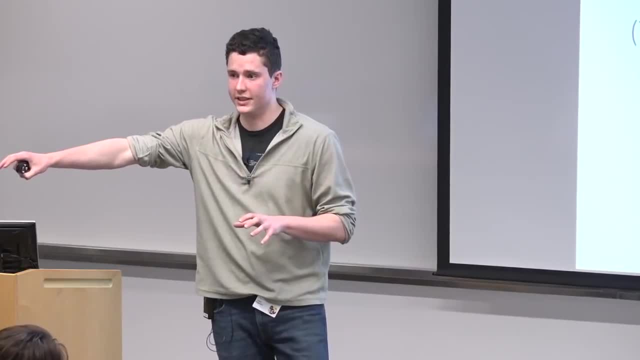 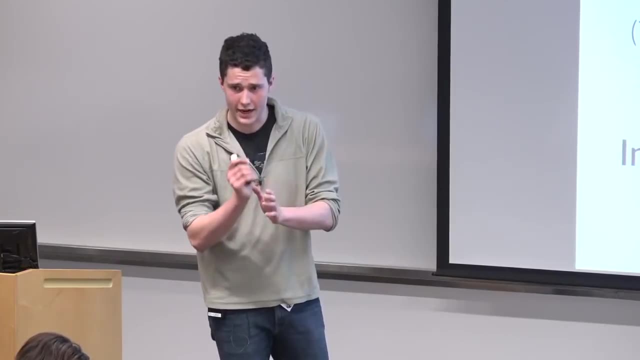 if you have a given state, the value is the expected reward that you get after visiting that state. So the idea is that if you can estimate these states well, then you can better separate out the action quality- what action you take from the action that you take versus what the state quality is. 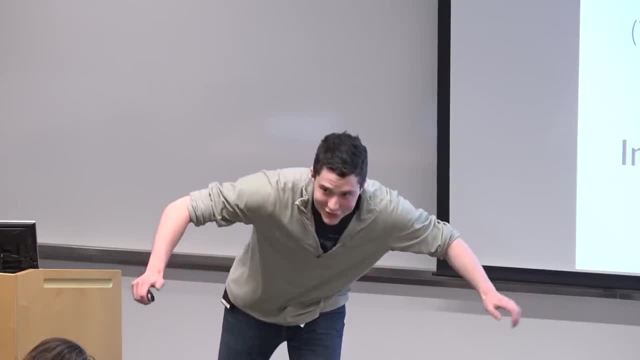 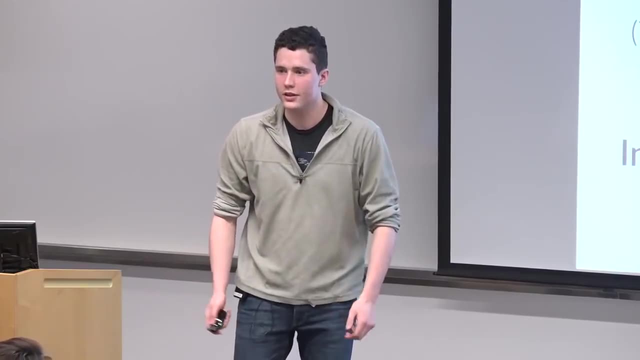 So, for example, if you have a robot and it's about to fall over or something, then you take an action. you don't want to say the action is bad because you're about to fall over anyway. So the idea here is that if you can understand what the state contribution. 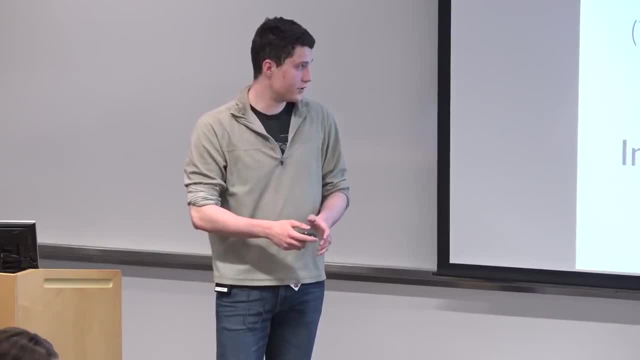 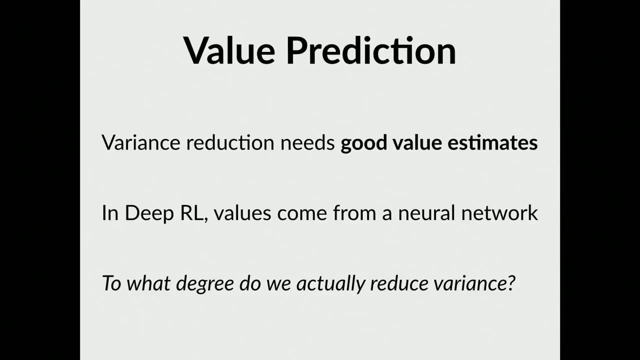 to how good the algorithm does versus what the action contribution is, then you can significantly lower the variance. To reduce the variance you need good value estimates. The way that we get value estimates is during training. we collect all these different samples of states and rewards. 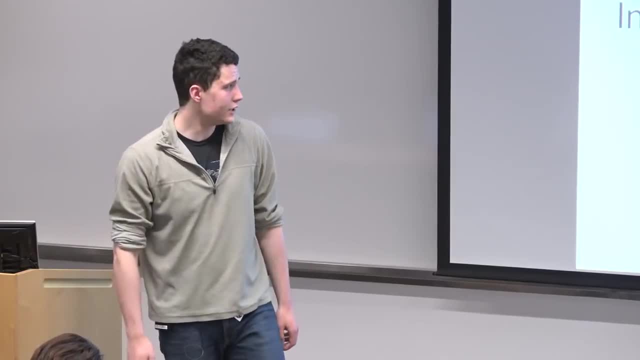 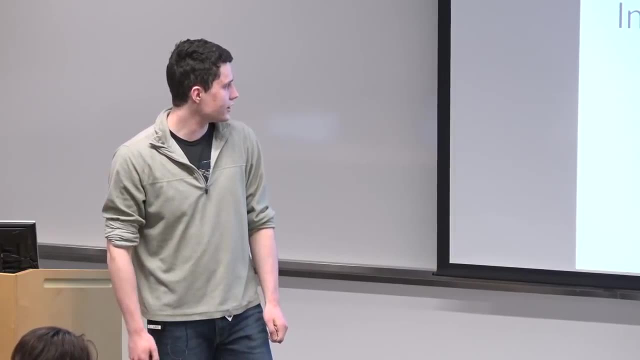 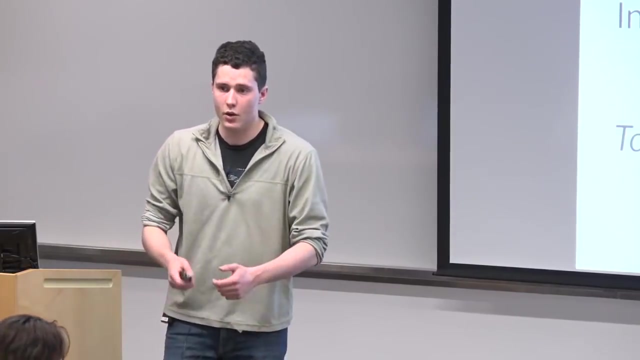 and you can calculate what the values are from that. So we basically just perform a supervised regression task at every point in the training process using the data that we collect. So we really want to understand here: what does the value, what do the value estimates do? 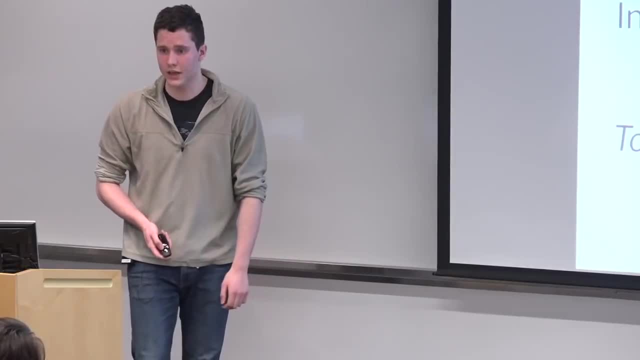 What do the value estimates we get do in terms of reducing our variance, and how well could we actually do? Also, how bad is it in terms of the baseline if you don't do anything? So the way we're going to do, that is we're going to do. 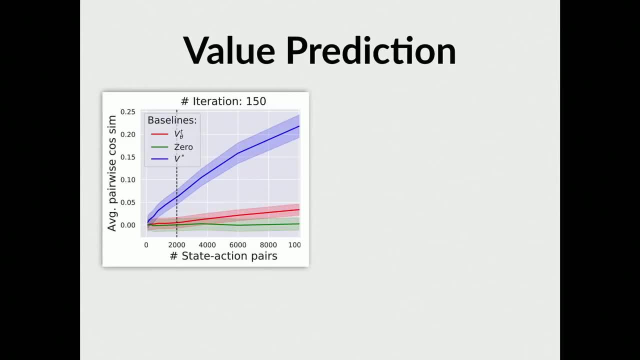 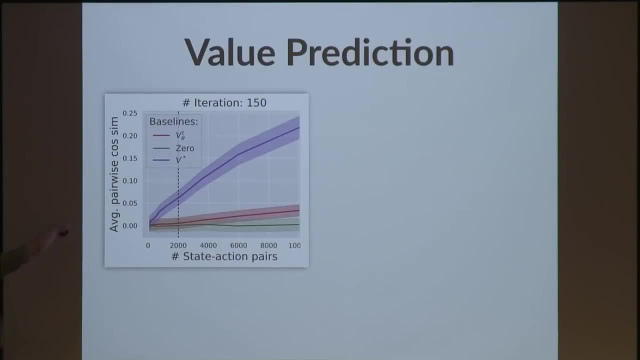 a similar experiment to last time, where we vary the number of samples on the x-axis and we vary the concentration on the y-axis. It's the same exact plot as previously, But now we're going to look at three different kinds of agents. 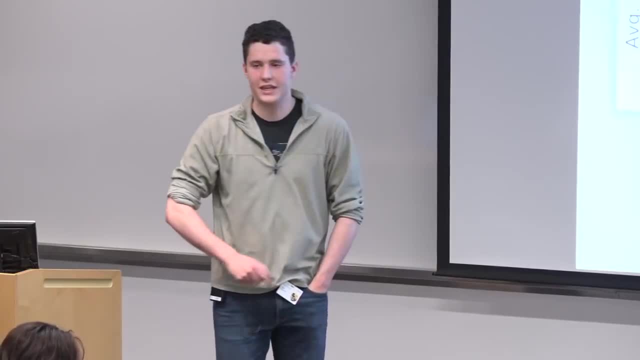 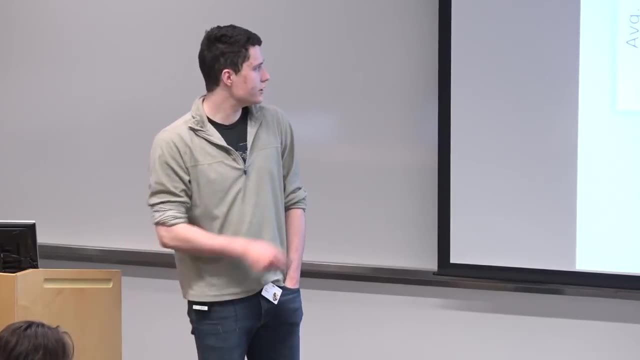 So the first agent is when you don't use any baseline at all, So you don't use any value estimation. So then the red line here represents what happens when you use the standard value estimation from the algorithm. Then this blue line represents what would. 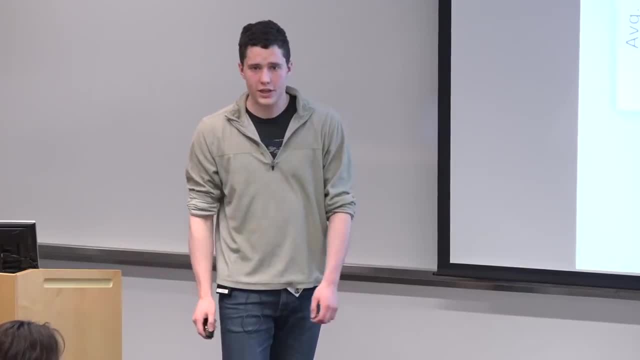 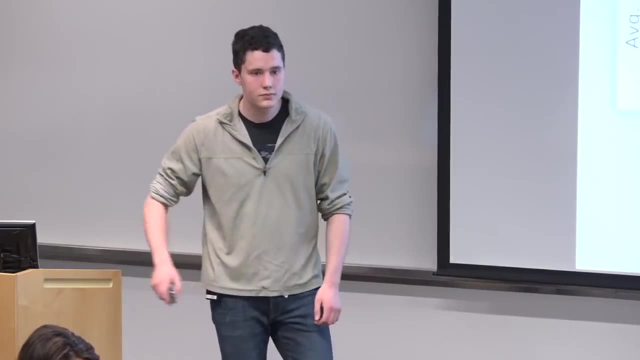 happen if you got a near ideal value function. The way that we calculate that is: we basically just take a ton of samples and we very well approximate what the value function is. So just to be clear, the star here actually refers to the value function of the current policy, not the optimal value function. 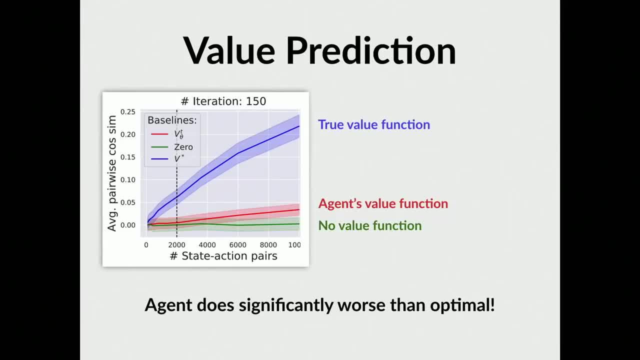 Yes, Okay, The value function of the current policy. So this is no value function. This is the agent's value function and that's a true value function. So it turns out that the agent does significantly worse than what it could be doing if it had the true value function. 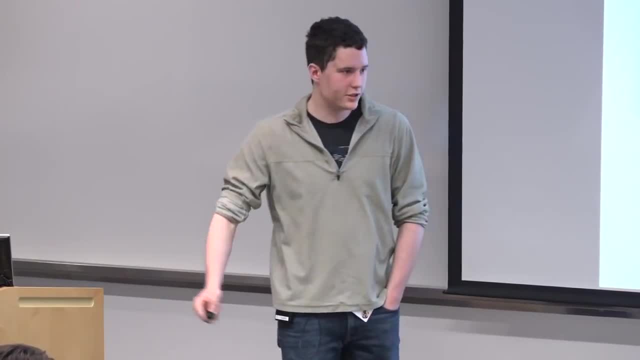 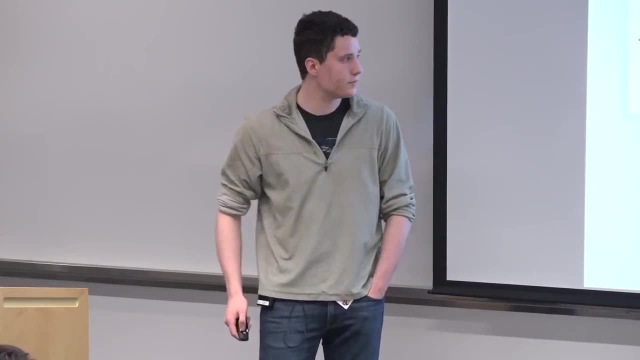 But it's still doing significantly better because, again, remember that we're in high dimensions, so this is actually pretty good. It's actually doing quite better than no value function, But there's clearly significant room for improvement. here You can see that the concentration gets. 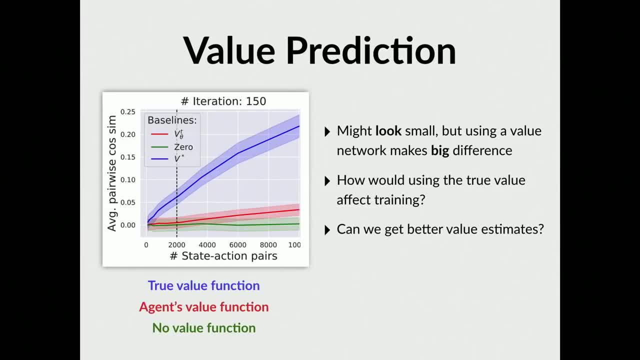 much better for the true value function. So one of the key questions here is: if we were able to get better value functions, how would that affect training? How much better would we be able to do? How much more reliable would it be able to be? 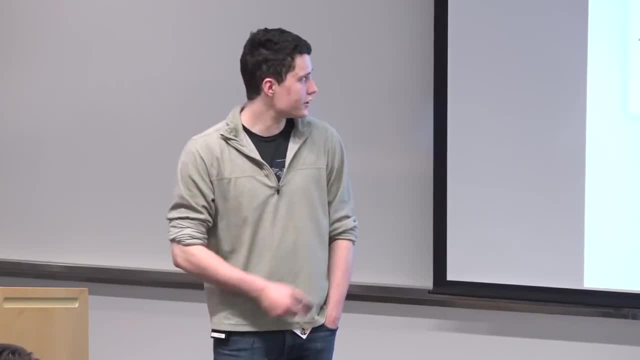 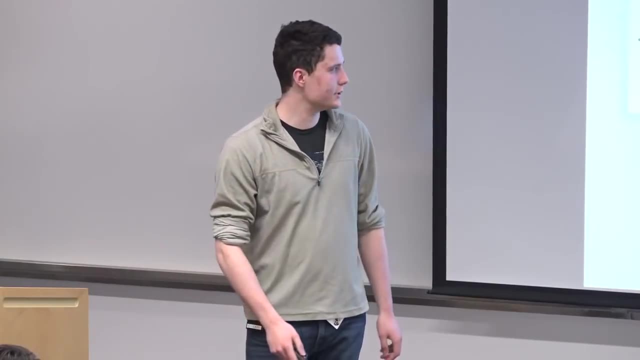 Not only that, but how can we actually get better value functions? Because it's clear that there's a big benefit here. What's unclear is how well that would really translate to our optimization in general. So now the third tenet that we're. 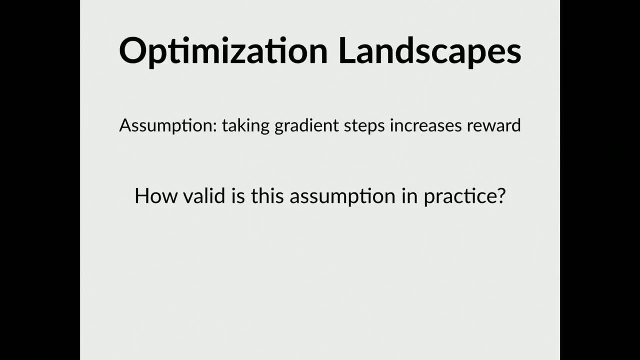 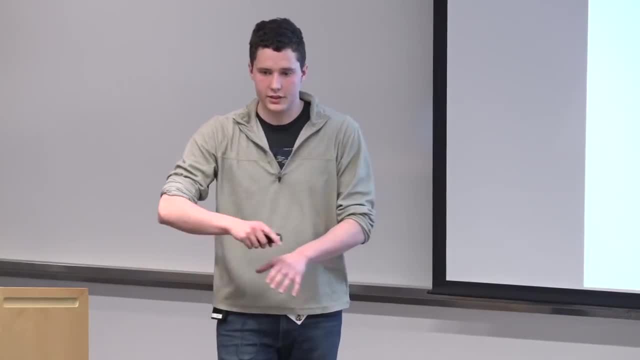 going to look at is of optimization landscapes. So a key assumption again in our policy gradient framework is that when we take these gradient steps we increase the overall reward that we're going to get from that policy. So what we want to see is how valid this assumption is in practice. 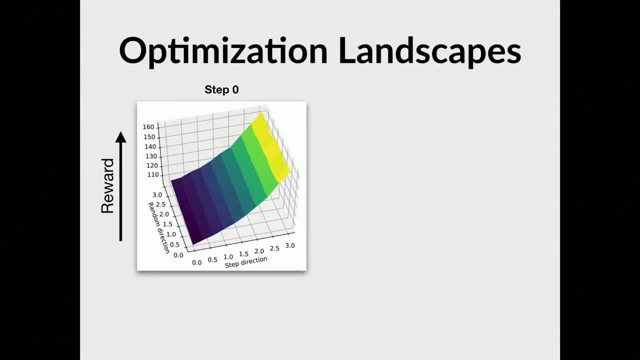 So we're going to look at a lot of plots of this form in the next few slides. So we're going to make it very clear what these plots are. So this is essentially in this direction: we're going to fix a policy and then in this direction represents moving. 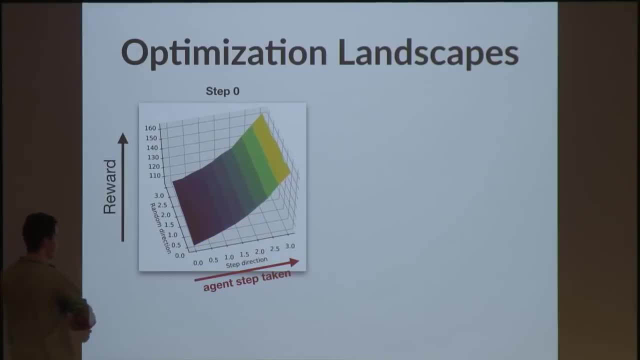 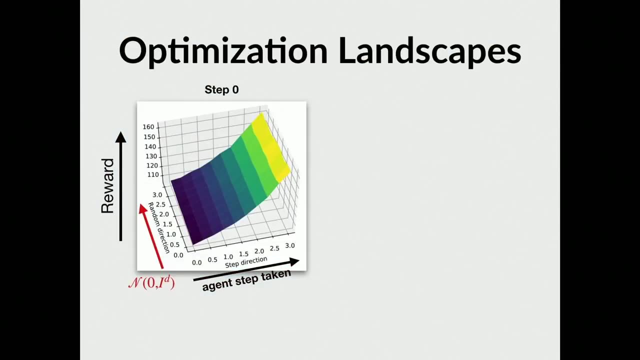 in the actual step direction that we get. So this point represents what the actual step would be in the next step. Then this direction represents going in a random direction, chosen from a Gaussian. Then what the actual plots here represent are the reward that you get at that new policy. 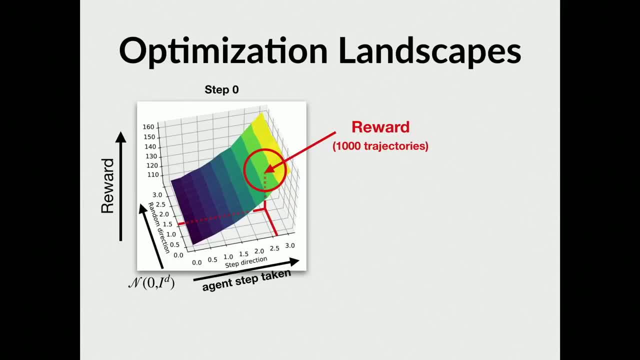 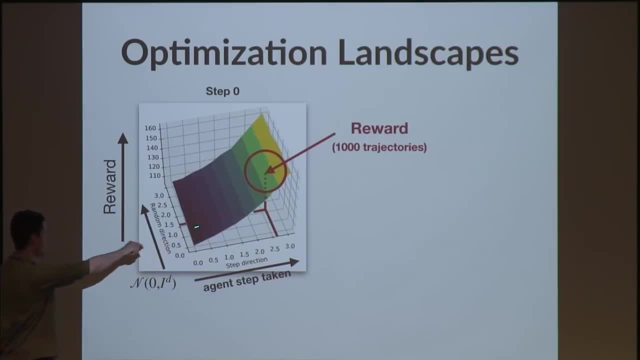 So you fix a policy, then you move this much in the agent step direction and you move this much in the random direction. So one example here is this red stuff right here represents you move 2.5 times in the step direction and you move 1.5 times in a random direction. 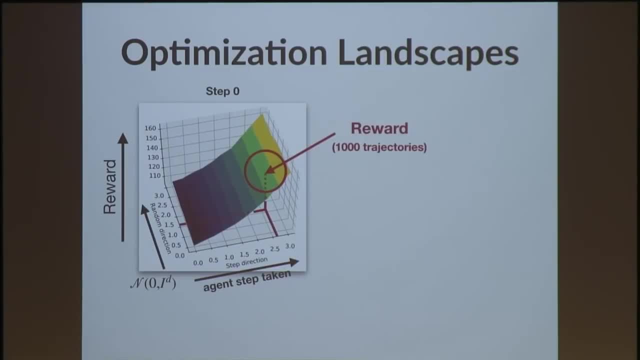 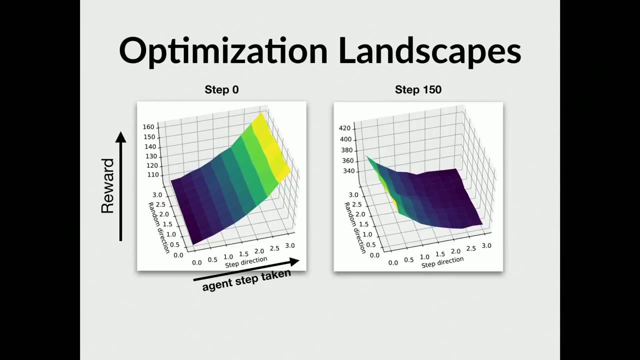 and then this is the ultimate reward that you get from that policy. So this is step 0.. You can see that we're doing pretty well here. You move in the step direction. you get increasing rewards, which is great, But then by step 150,. 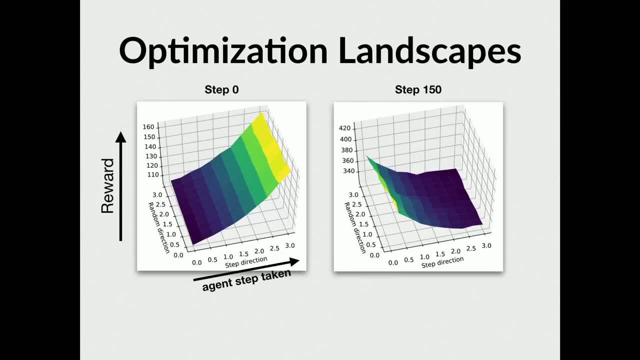 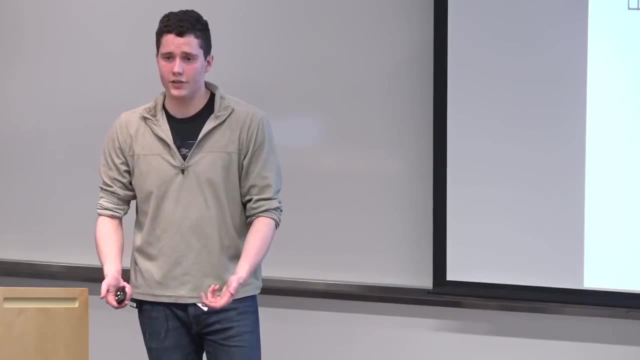 you can see that this really degrades quite a lot. But just moving in the step direction this actually lowers your reward. That stays true at step 300.. We looked at a lot of these kinds of plots and essentially shows that oftentimes the steps 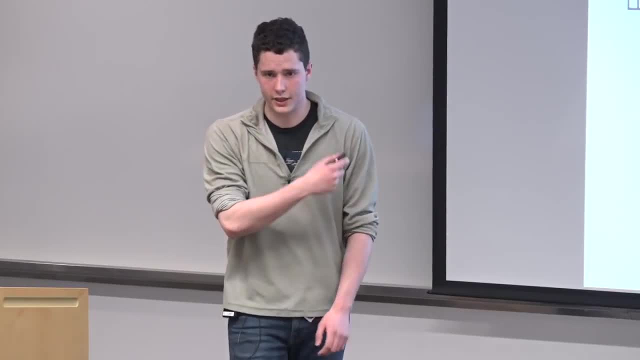 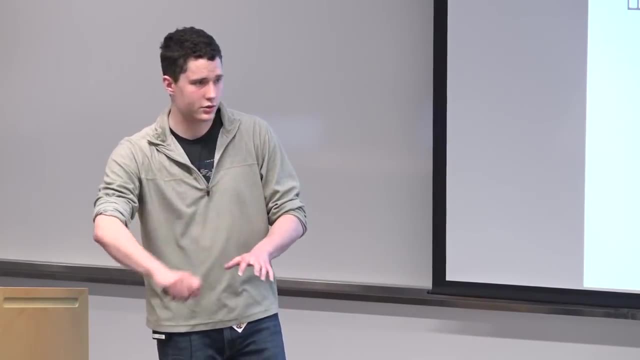 are not predictive. later in the optimization process This looks even worse again for harder tasks. So for easier tasks it looks a little better, But for these harder tasks it looks much worse. So natural question to ask here is: what's going on? 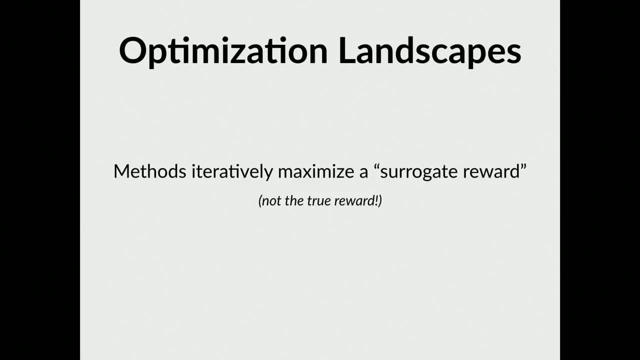 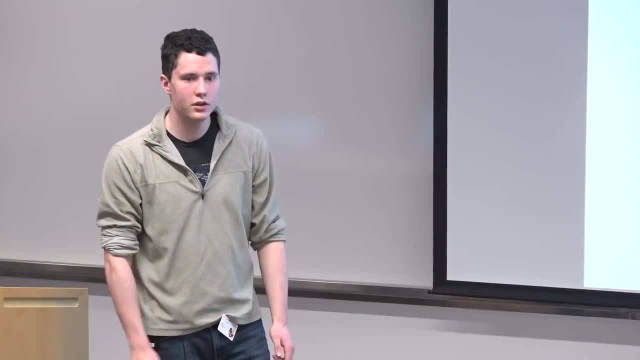 It turns out that when you look at what the algorithms are actually doing, they're not maximizing the actual true rewards. What, instead, they're maximizing is some surrogate reward. Sorry, I have a question on the previous one. The x-axis is the step taken by the agent. 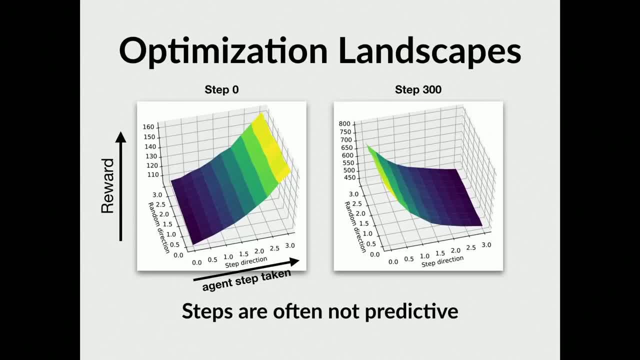 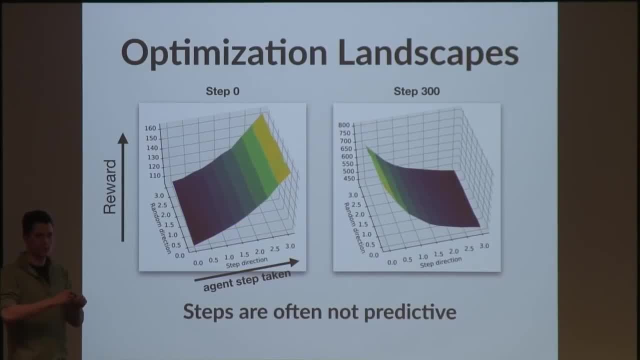 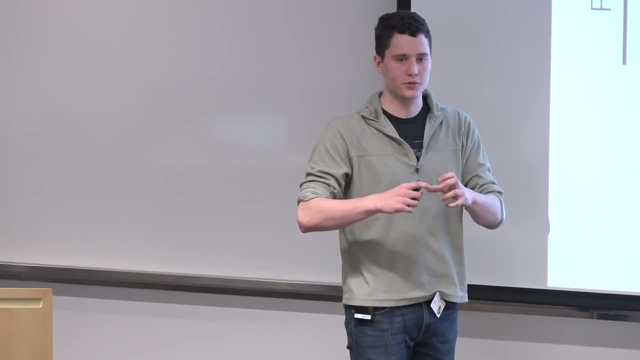 Yes, So you're talking about this one, right? Yeah, So I fix a policy and then I move x times, step in policy space and then I evaluate how that agent does in terms of reward. Does that make sense? So it's moving optimization like parameters space. 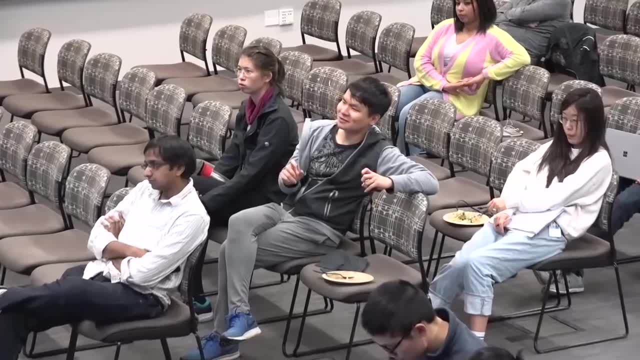 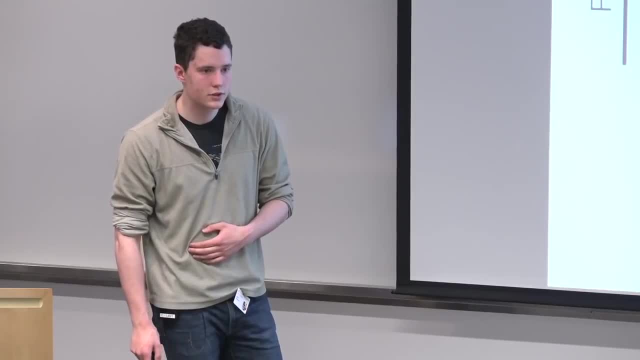 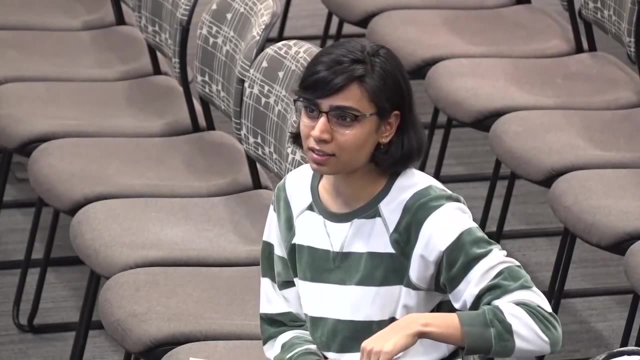 Yes, Okay, Because agent step taken sounds like it's agent taken step Right. The random detection would be like adding noise to the gradient. Yes, But aren't there results that show that adding noise to policy gradients actually helps? I'm not aware of any. 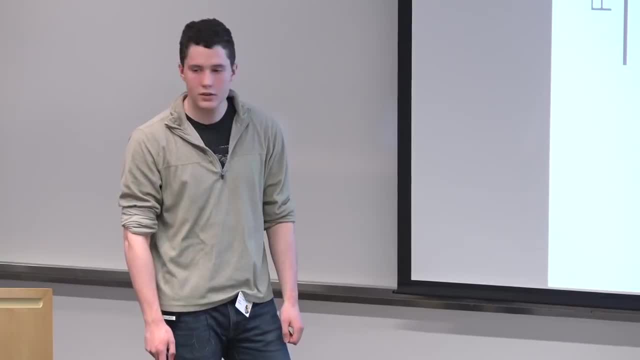 but it would be. I'm happy to talk. Okay, I'm fine about that. Sure, You're also adding noise to the policy parameters. Yeah, It's also adding noise to the policy parameters. I'm not sure if that's-. 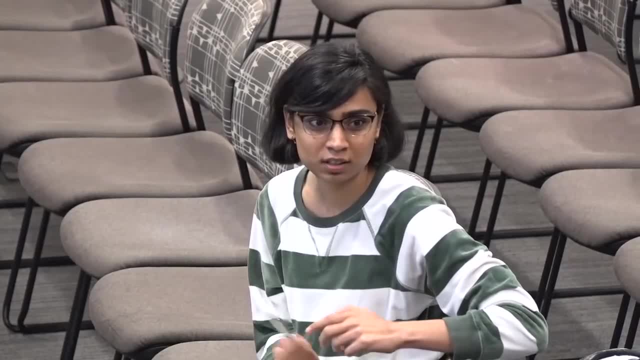 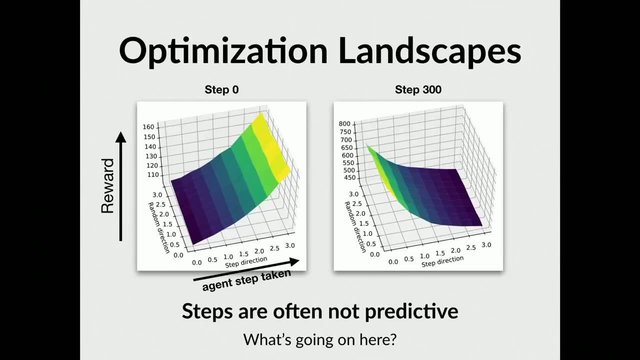 Yeah, There's a paper from OpenAI called Parameter Space Exploration. Yeah, yeah, yeah, yeah, You can Sure. Yeah, Any other questions about these slides? Is everyone clear about what's going on here? Move in the parameter space in the step direction. 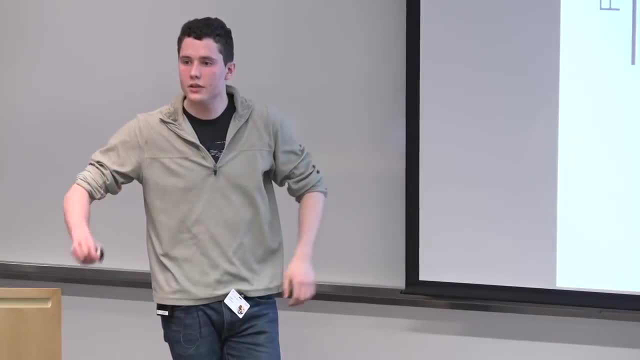 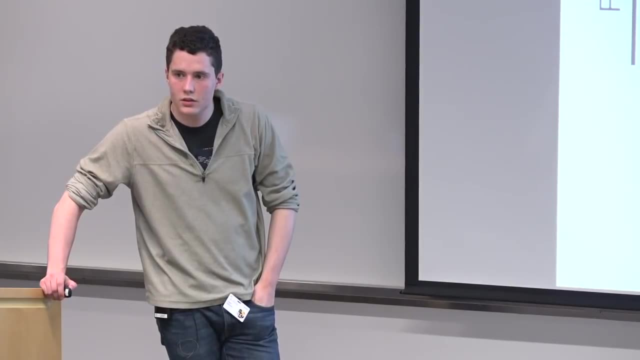 and you can move in a random direction. This is the kind of plots you get, Yeah, Well, this is a good question, Because we are following the gradient direction. why the reward is going down This part? I- We're going to explain that in the next slide. 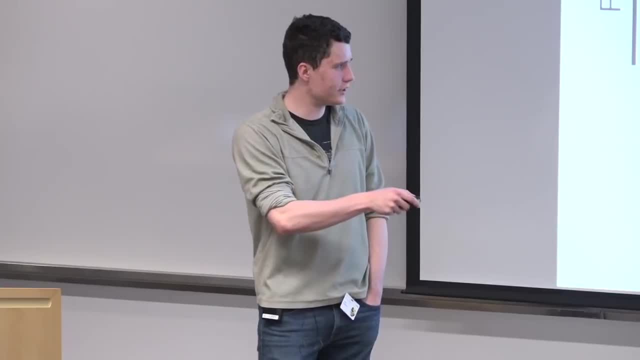 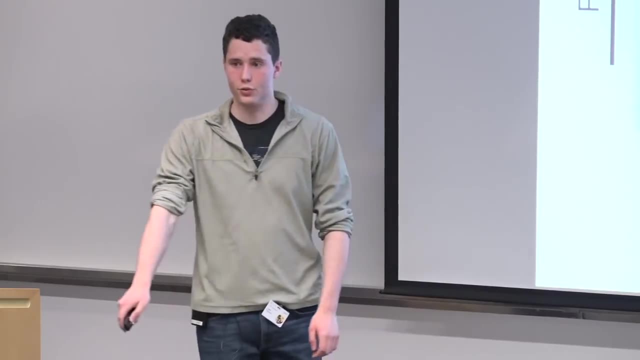 Yeah, So that's. the key question here is: why is it that we go in the direction of the actual step that we take? why is it that the true reward is going down? It turns out that these methods actually don't optimize the true reward. 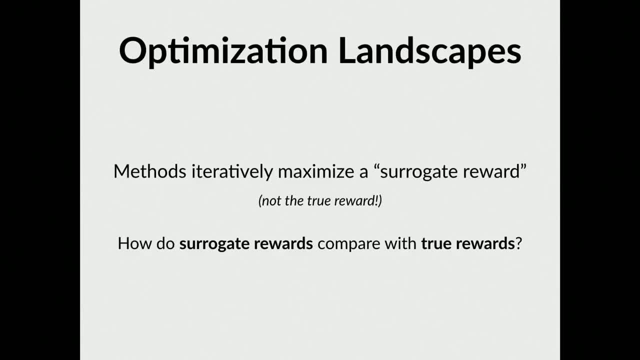 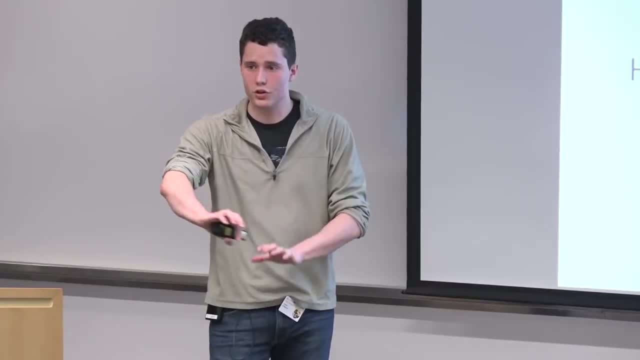 What they instead optimize is something called a surrogate reward. I'm not going to go into detail about it, but we can talk afterwards. But what this actually is, What we want to check here is how the landscape of surrogate rewards compared to landscapes of true rewards. 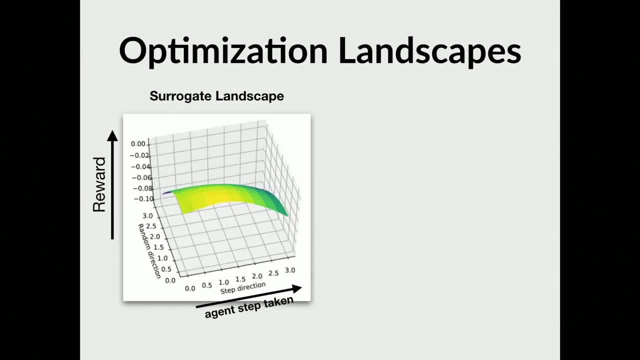 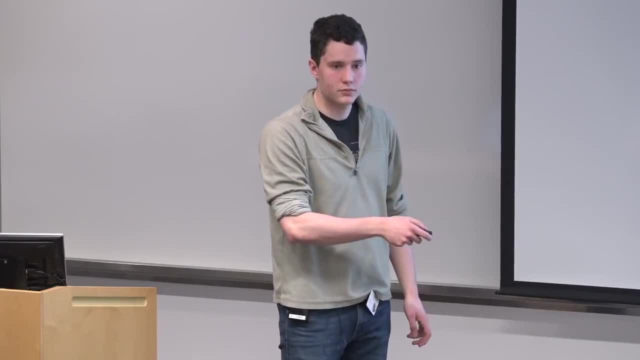 So this is a surrogate reward. landscape is the exact same format as our previous landscape, except that now it's a surrogate rewards instead of the true rewards. So surrogate is coming in because of the proximity stuff in the NTP, or Yeah, Okay? 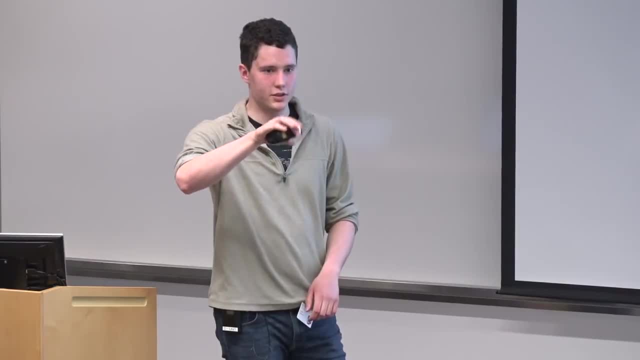 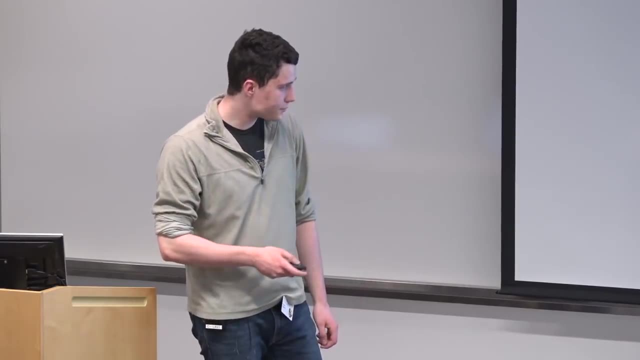 Yeah, So they look at basically the policy ratio, times. the policy ratio always gives you times, the advantage, and that's what they're optimizing instead of the true rewards. So this is what the agent is actually optimizing, So you can see that it has a maximum rate where 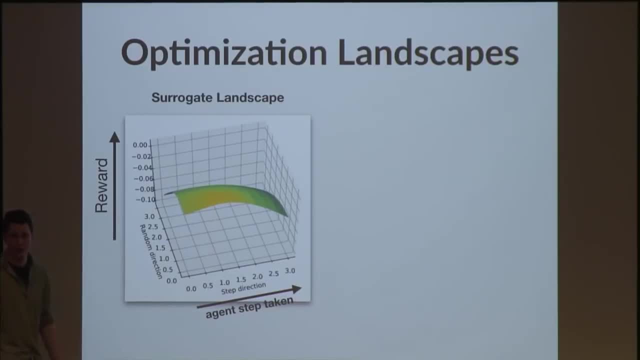 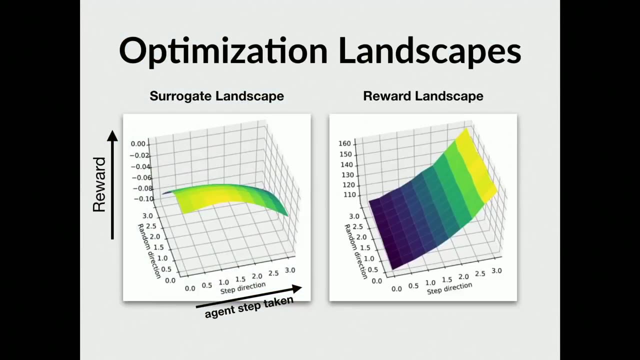 the step direction is, so it's actually maximizing the surrogate reward really well. That makes sense because it has full access to the surrogate reward, So it should be able to optimize it really well. It should be clear that the surrogate reward is based off of what it sees in training. 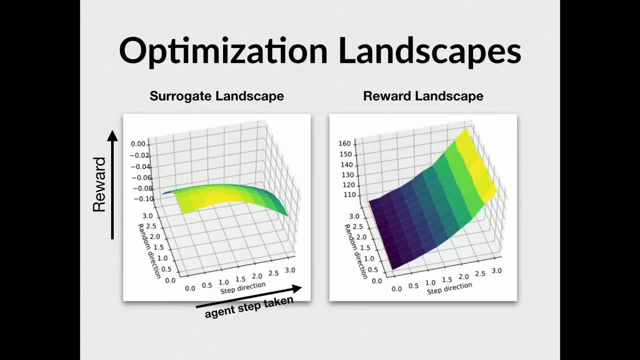 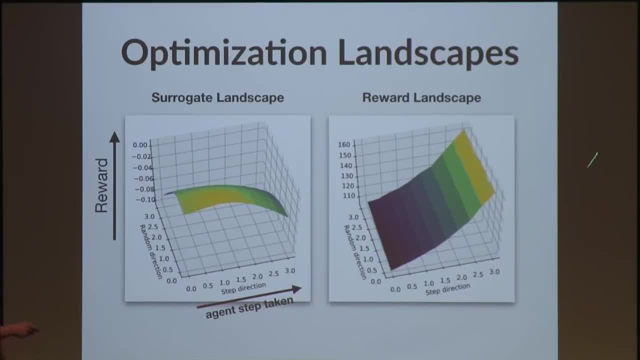 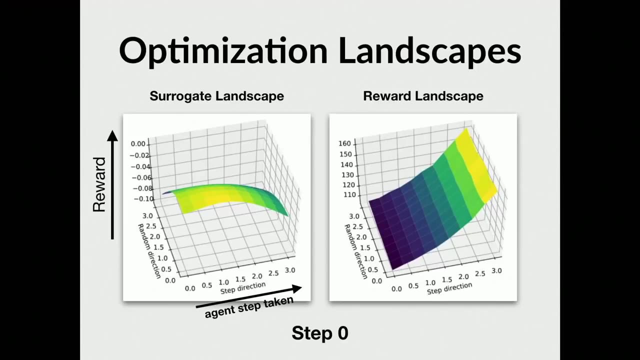 It's just that they have some smooth approximation and it's based on some theory, But what ends up happening here is that these actually work pretty well. This is step zero, and what happens is you move up in the surrogate landscape direction. you also move up in the corresponding reward direction. 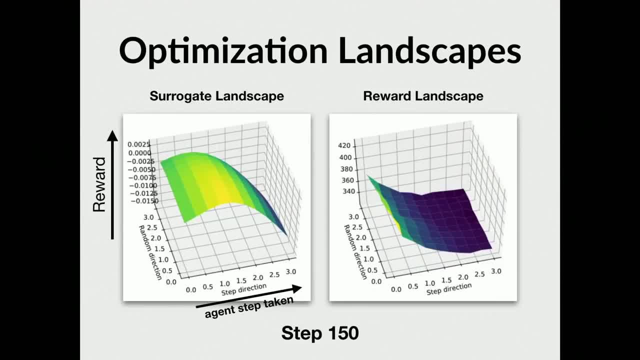 So this step does pretty well, But then by step 150, you run into the same problem that we saw in the last slide, where you move in the surrogate direction. it looks like this is the optimum, But then what actually ends up happening is that in the true reward landscape, 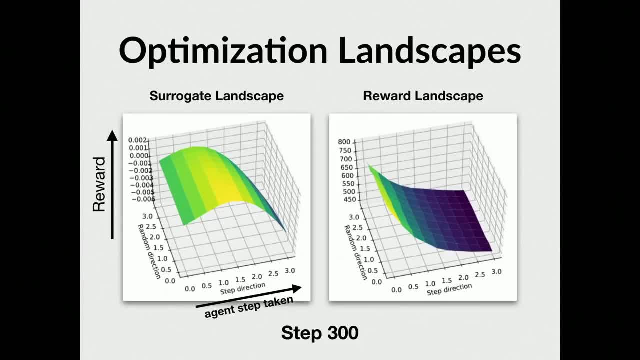 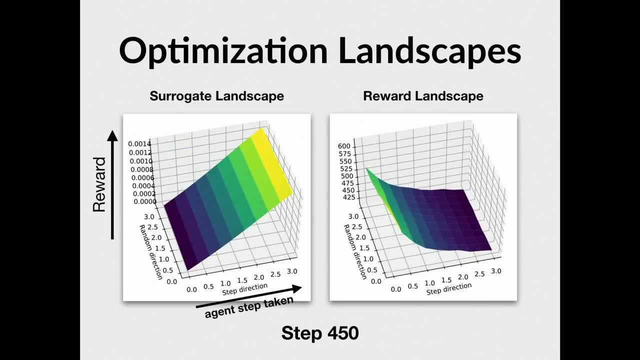 you're going down, you're getting worse rewards. This continues to be true at step 300 and 450.. This looks great, right? You just optimize as much as we want. But it turns out that even when you move in the surrogate direction, 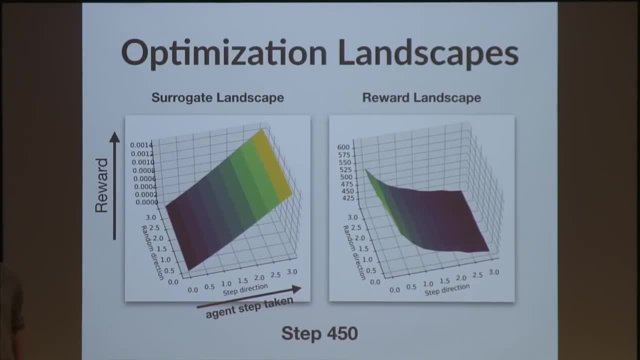 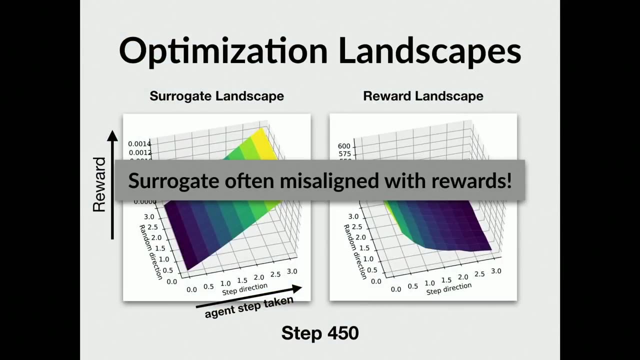 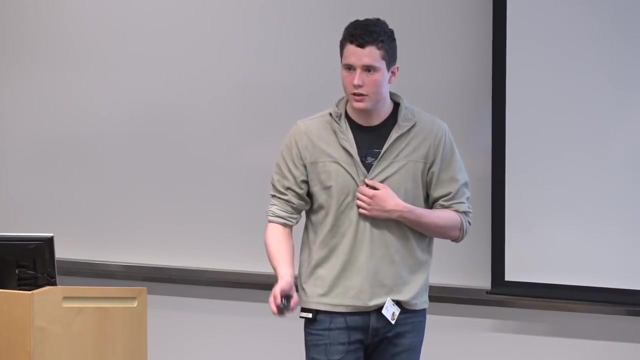 increasing the surrogate rewards. you're seriously not doing very well in the true rewards landscape. So here the surrogate landscape is the landscape for the value network, or how do you get the surrogate landscape? Yeah, So I'm happy to talk offline about it. 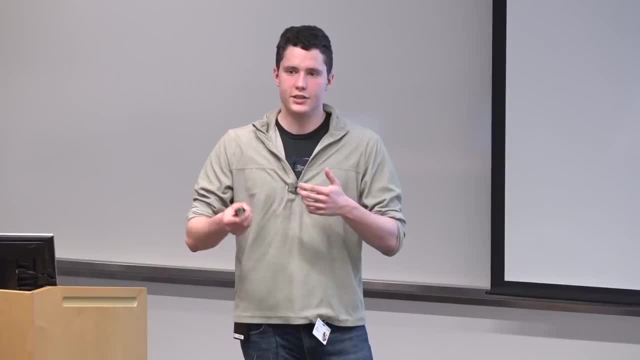 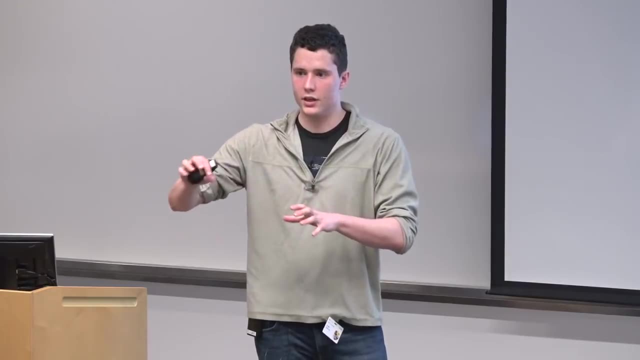 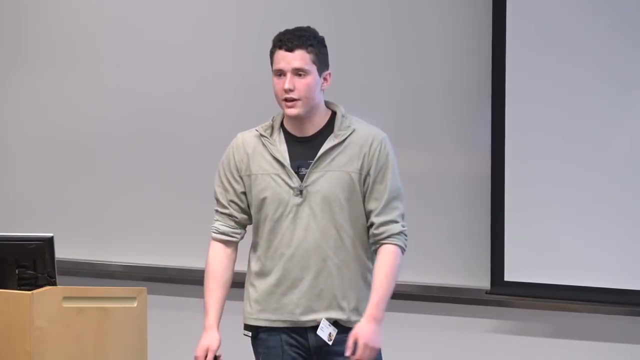 But essentially the surrogate landscape is just a function of the trajectories that you see. So you collect all these different trajectories and training and then you make a surrogate out of it which is motivated by some theory work. Yeah, it uses the value function as well. 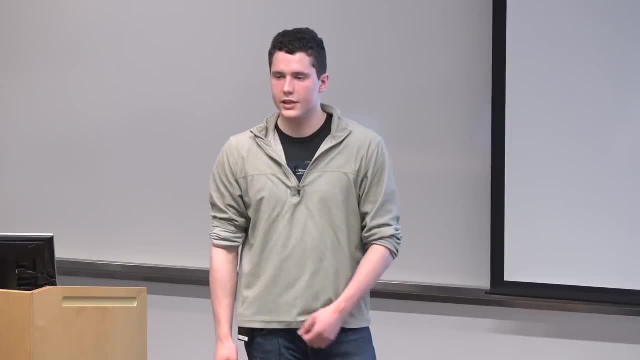 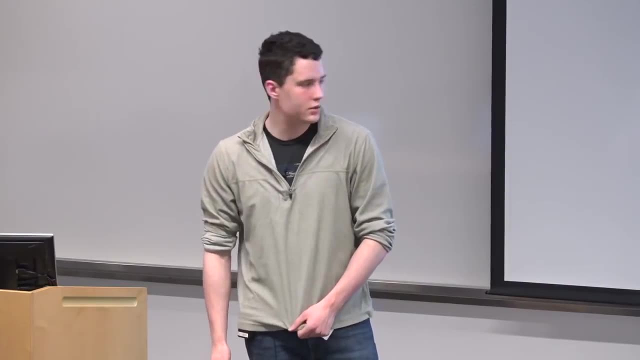 It's the landscape for the policy. Yeah, It's a landscape on the policy, I'm sorry what? It's the landscape for the policy network. This is all the policy parameters. Yes, Yeah, We're again operating a policy space. 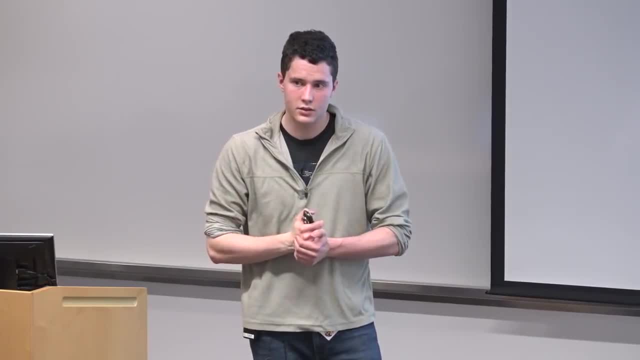 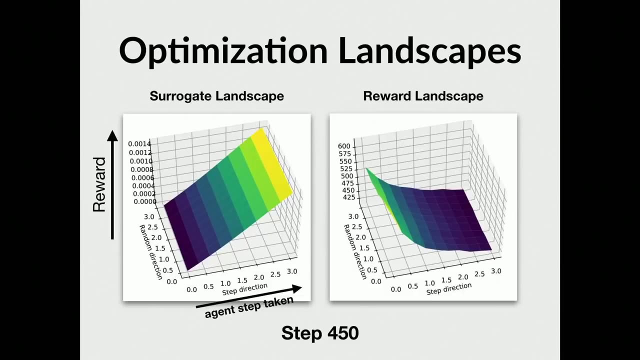 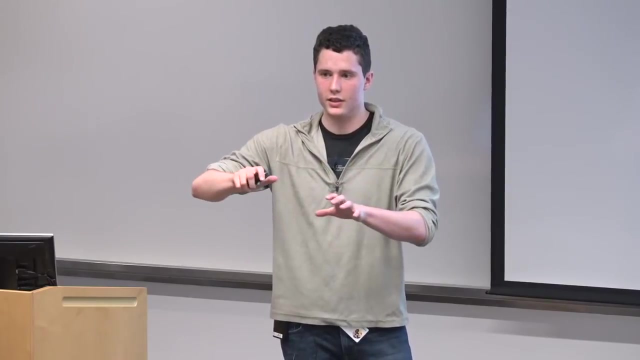 Does that make sense? Yeah, No, Still. So you can think about this just abstractly. You can think about the surrogate reward as something that the algorithm is actually optimizing over. It takes in the trajectories and then it makes a landscape, what it thinks in terms 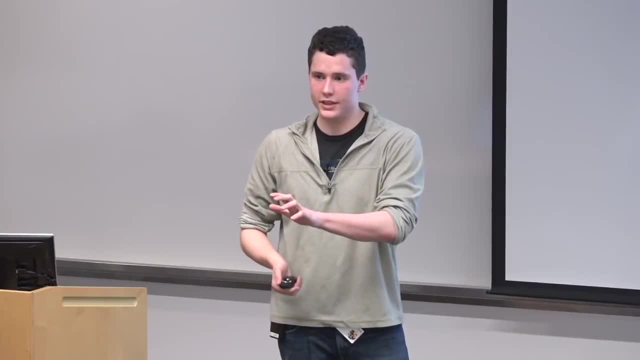 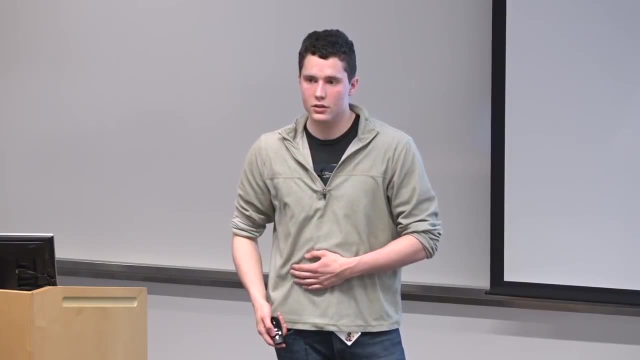 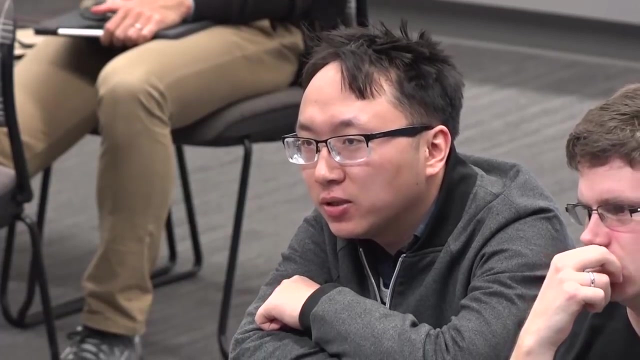 of it makes a landscape that it thinks corresponds to the tree landscape, and then it optimizes that instead of optimizing over this tree landscape. From my side, I think there's two approximations. One is you use a Monte Carlo to sample, to estimate the expectation. 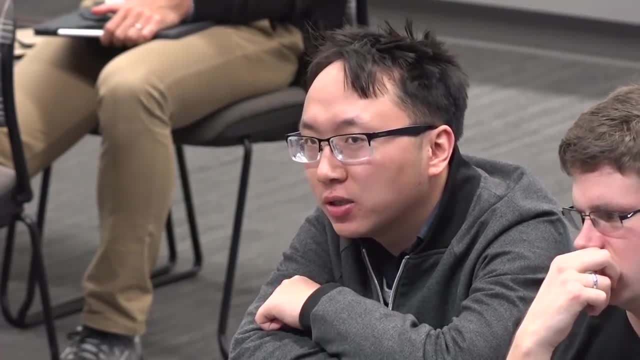 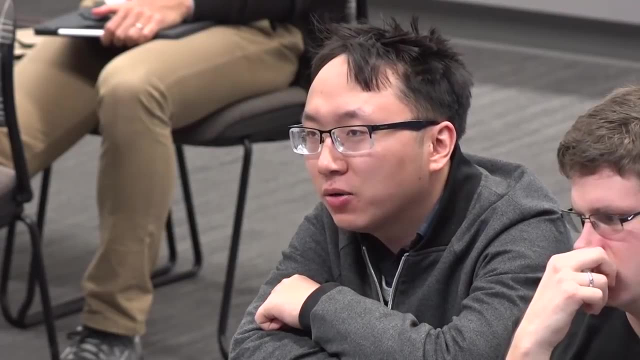 That is one kind of optimization. The other approximation is that I even do not know the true value function, so I need to use some network to optimize that one. So by surrogate here, so which approximation you are really- It uses both of them. 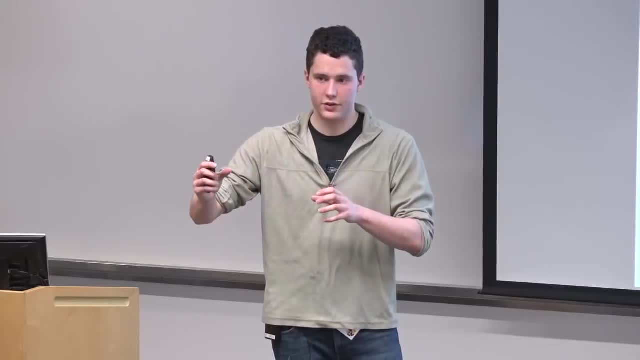 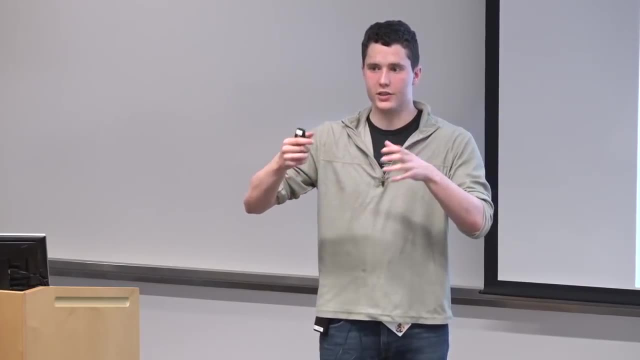 Both of them. Yeah, So it uses the value function and it uses the samples that we get, but it's not looking at the actual rewards you get. it's looking at some function of the actual rewards you get. Yeah, Are you measuring these functions on the same scale? 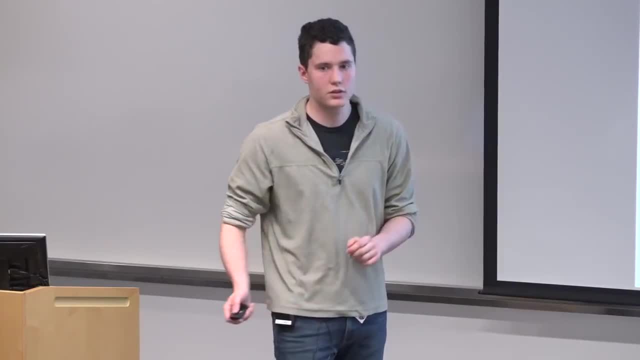 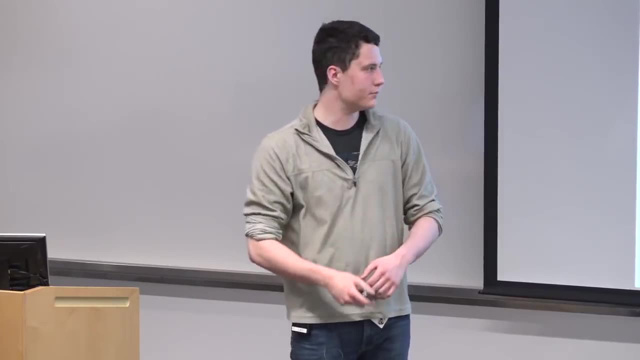 Sorry, are we seeing-? Yeah, So you should- The surrogate reward by a very small amount, it's- Right, So you should ignore the scale in terms. of. the only thing that's important about this is the direction. Like this goes up, this should also go up. 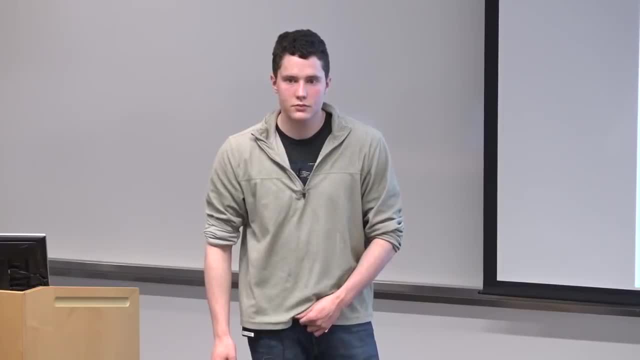 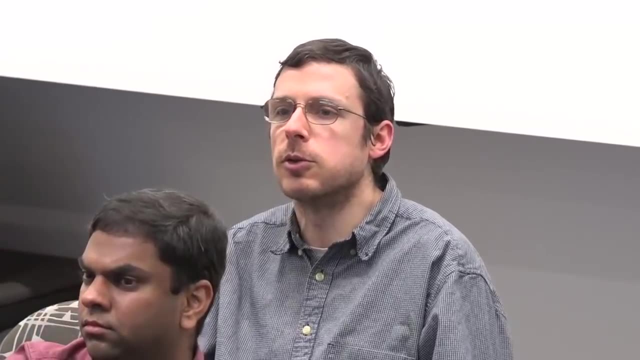 I'm just curious: in trying to take a step to achieve a very small improvement in the surrogate reward, are we seeing a comparatively much larger decrement in the true reward, or are these scales not comparable? Yeah, These scales are not comparable, Okay. 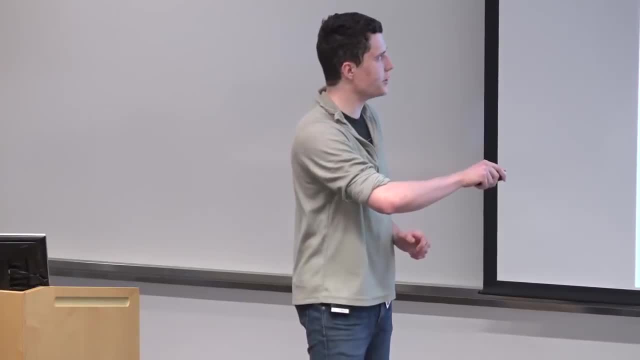 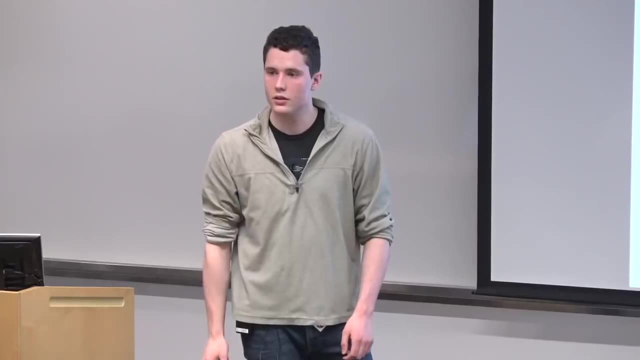 But it's definitely regardless. it is concerning that you move. when you're increasing the surrogate reward, you are decreasing the true reward. Yeah, Does the network, does the agent actually become better? Yes, Yes, it does. Yeah, So that's the key thing. 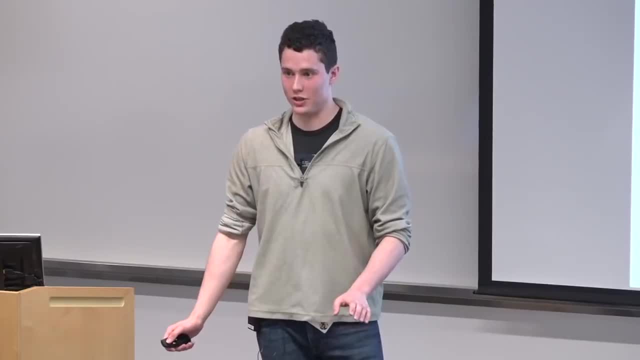 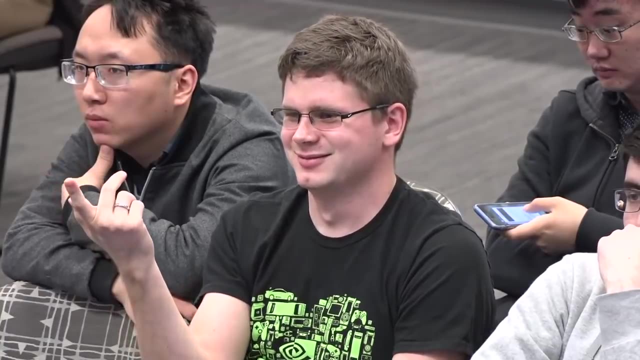 Throughout this whole presentation. I am not saying that these deep RL algorithms do not work, because they do work. But how can it become better if I hold this pretty much, after some point decrease my true reward. That's a great question. That's a great question. 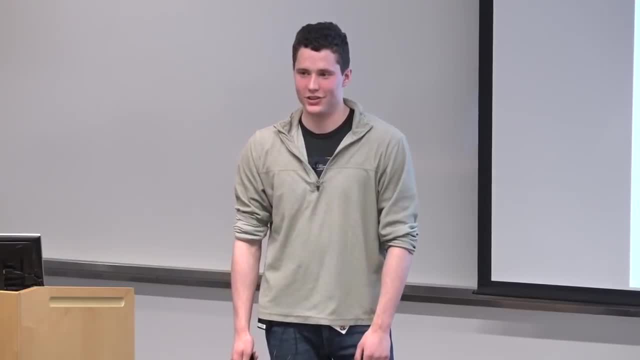 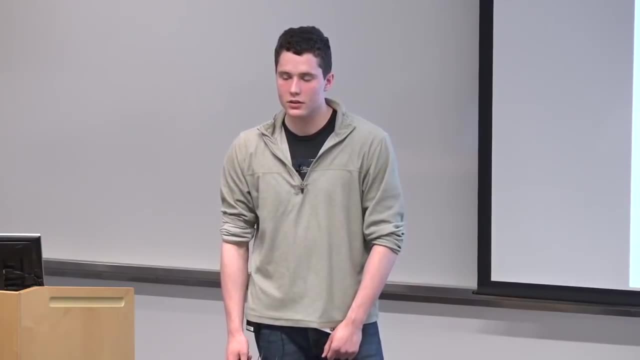 I mean, we have some hypotheses, but it's a little unclear. Yeah, This could be a source of the unreliability issues that we see. So for this slide, do you think that's the kind of the error many of them? 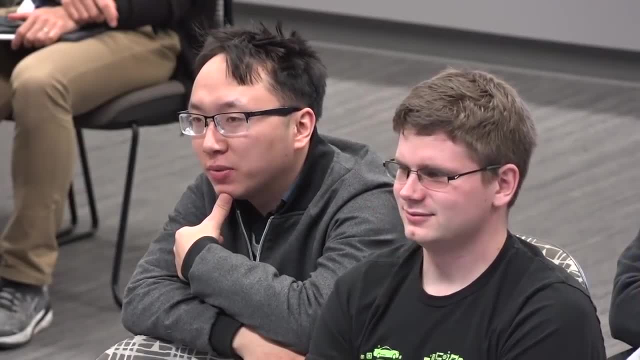 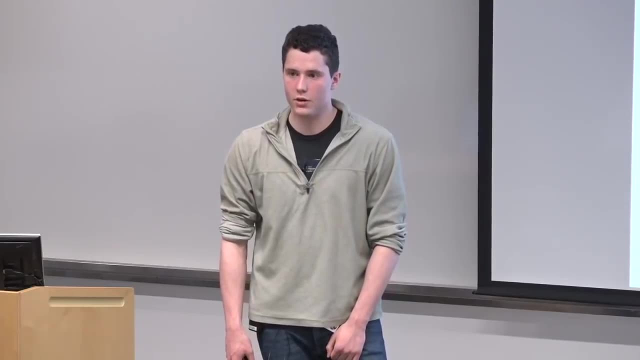 one of the kind of, or many of them from, the value function approximation. I think both of them are probably. I think both probably play a part in this, But it's more about the. I think both of these play a part in it. 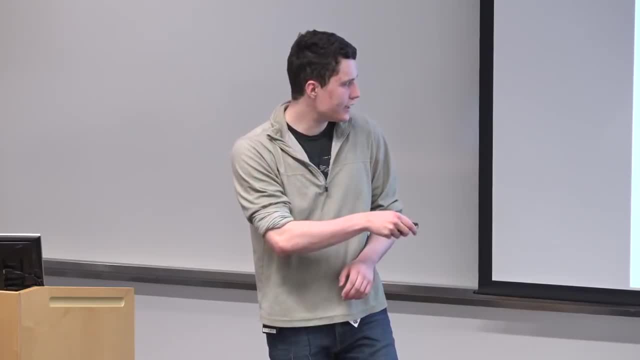 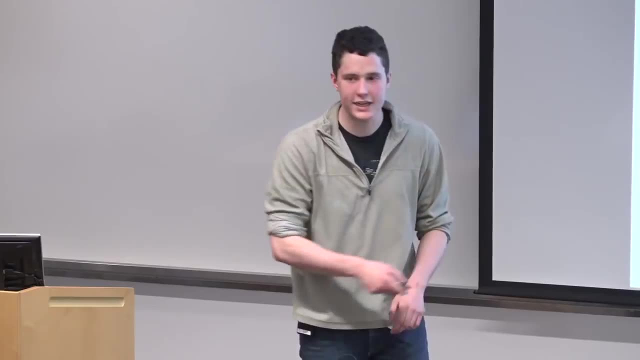 But actually. so when we take this step, we use many, many samples, So these actually should be pretty good, Like when you take the step we're not taking, like the actual agent step. What we're actually doing is we're using many. 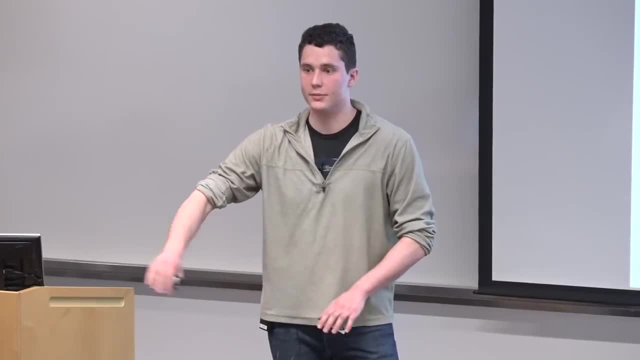 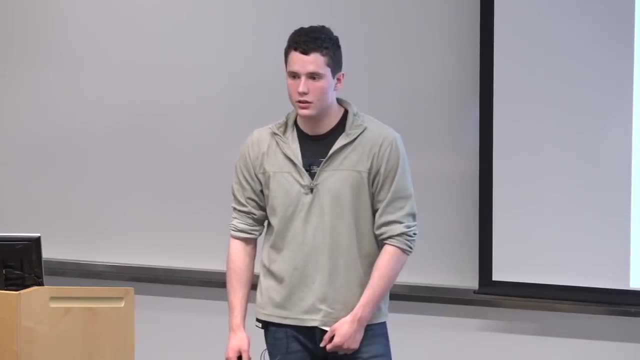 many samples to get like a pretty good approximation of what the agent step should be. So I don't think that those issues are super big. It's like a third source of approximation. Yeah, It's kind of another sort like a third source of approximation. error is like. 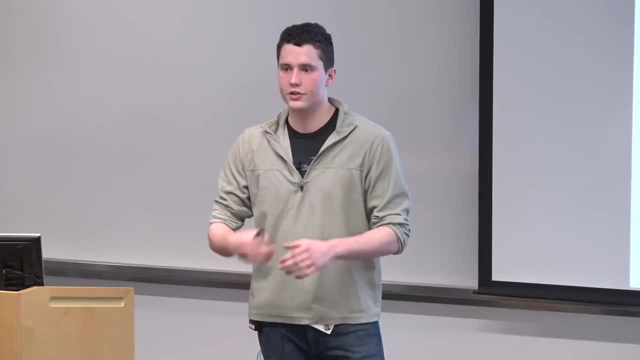 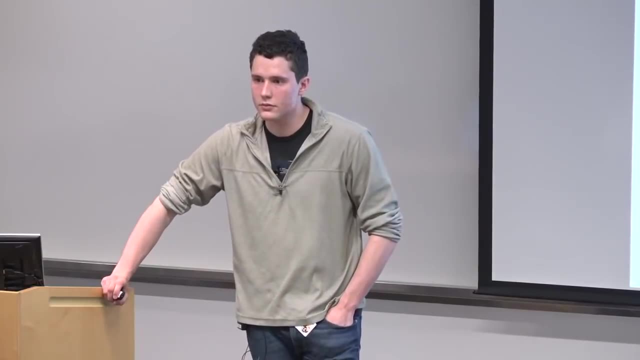 the actual function that they build out of the trajectories and out of the value function in the estimates. So in the same way that you can optimize accuracy where you train in deep networks, you optimize cross-entropy. It's exactly the same. You don't optimize reward, you optimize some surrogate of the reward. 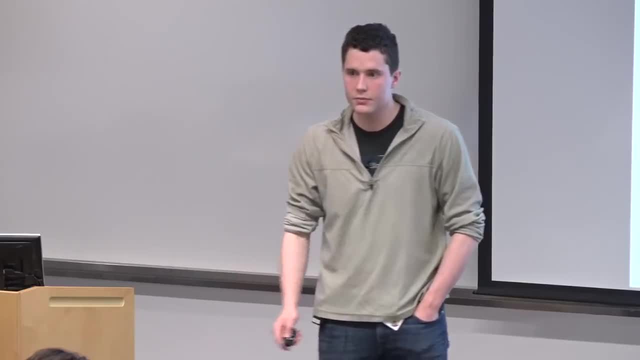 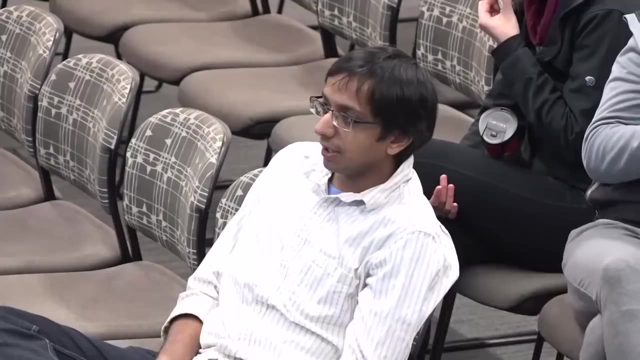 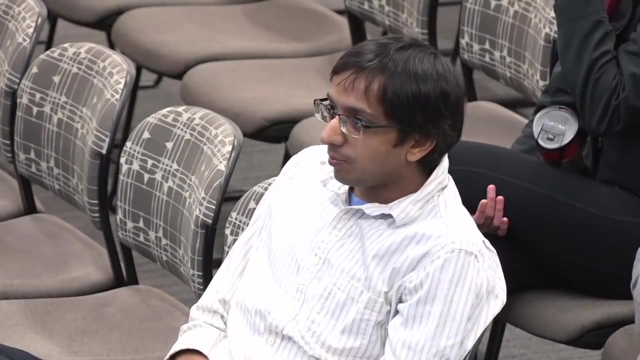 Yeah, That's what we're seeing here. Yeah, That's a great explanation. So I guess the quantity on the x-axis, the way I should think about it, is like the step size in my optimization algorithm, right, Yes, But then presumably the scale at which you're plotting things is. 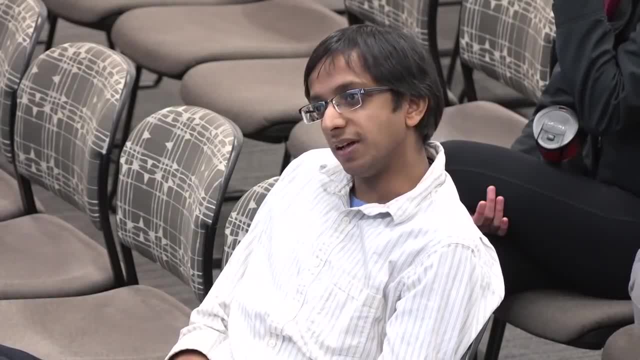 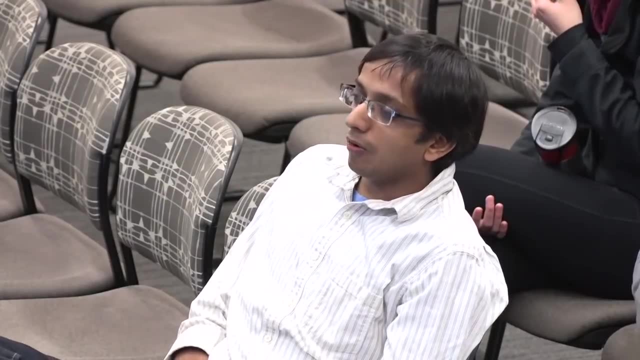 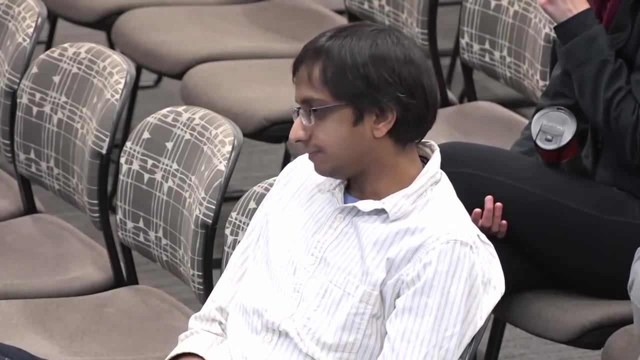 much larger than the regime in which the step sizes are operating and training at least. So one here is the actual step. Yeah, So if you- Oh, I see You're scared with the-. Yeah, I see, Okay, So if you just do early stopping at 150, would you get-. 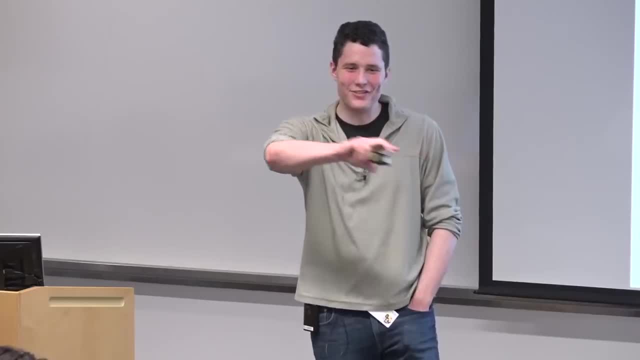 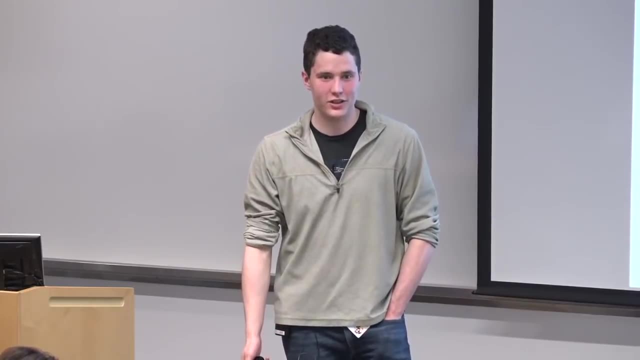 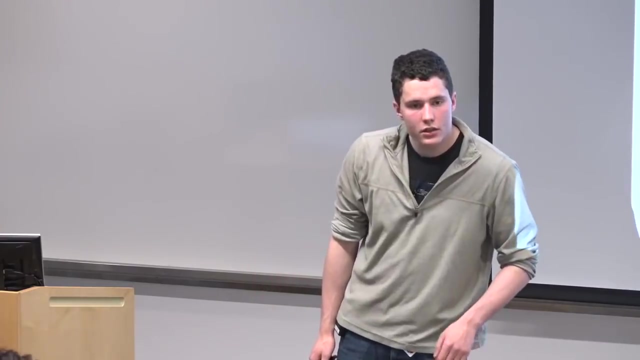 No, Actually, I mean, you definitely improve over time. So it's not like these algorithms are not working. It's just a little unclear what the mechanisms behind them are that are making them work. I'm sorry, what Like? it's a y-axis in the right plot here. 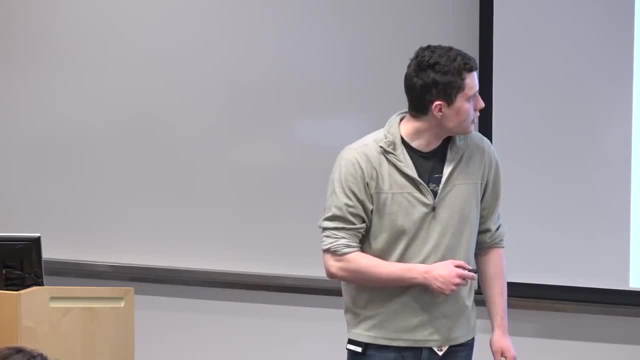 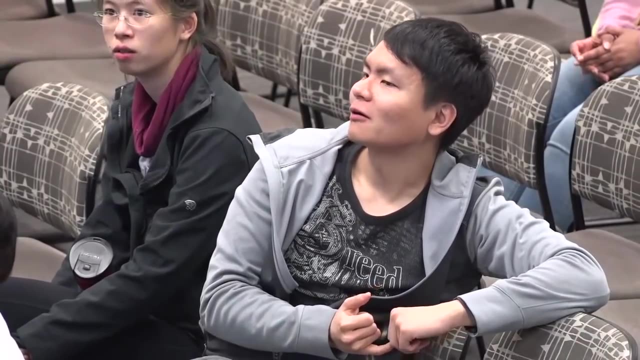 This is the same thing. you're claiming that the total reward will increase over time, Like if you look at the graph. Yes, This quantity exactly corresponds to what should be increasing over time. So how can that be if every step you take decreases? 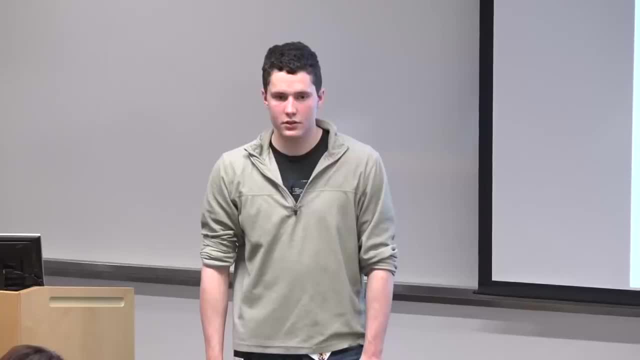 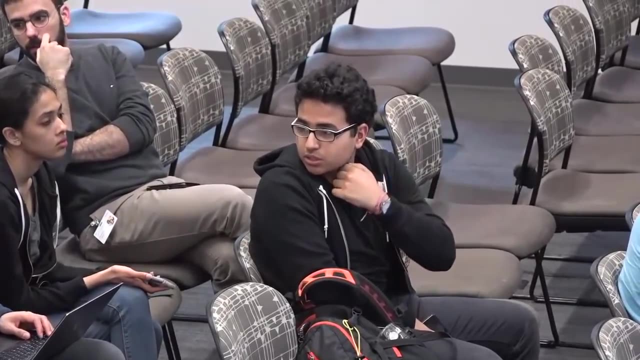 So it's not every step, So we sample a couple of steps. It could be that you take very few high magnitude jumps, but then if you sample at any point you're likely to see some small decrease. So maybe on average, like this doesn't do so well. 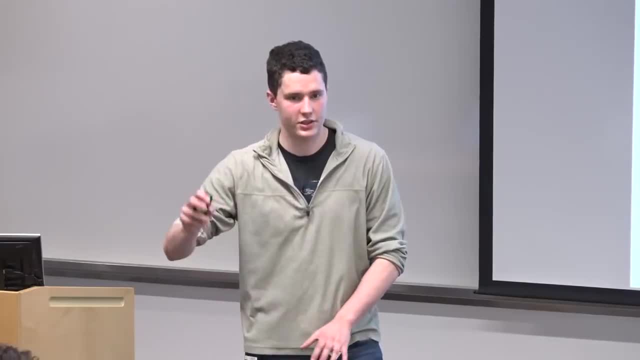 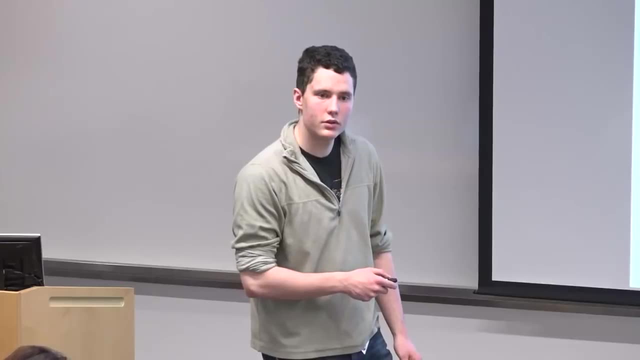 but you might get a few steps that are doing really well and so it kind of bounces out. So is this reward the return, or is it the stepwise reward, The total reward, over-. Yeah, This is the total reward. It's discounted return. 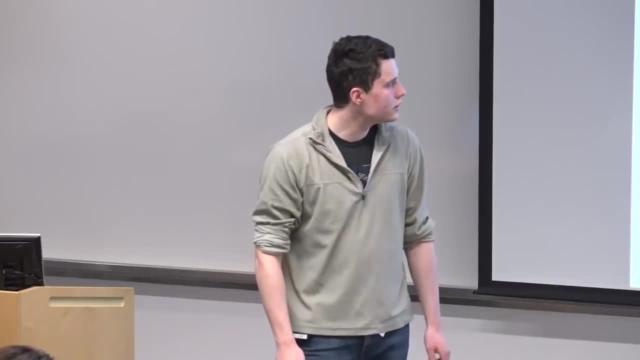 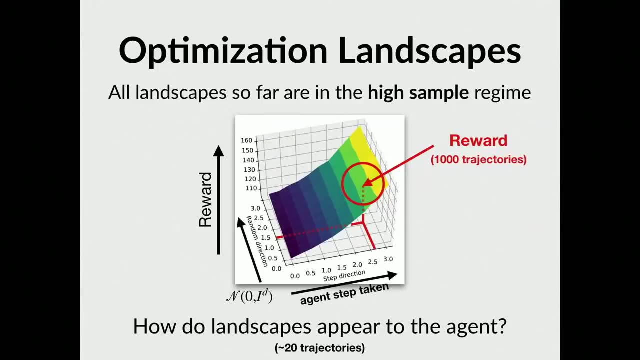 Yeah, It's discounted return actually. So, as we can see here, the surrogate reward is often very misaligned with the true reward landscape. It's important to note that everything we've looked at so far has been in this high sample regime. 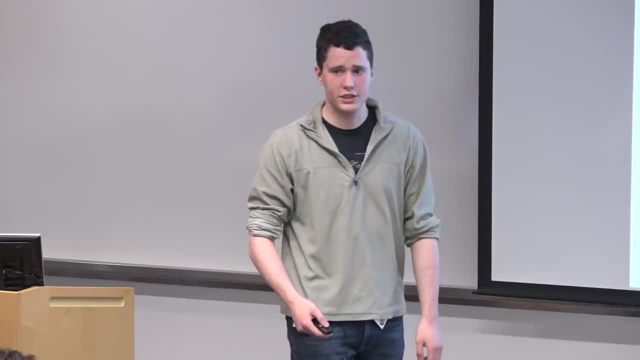 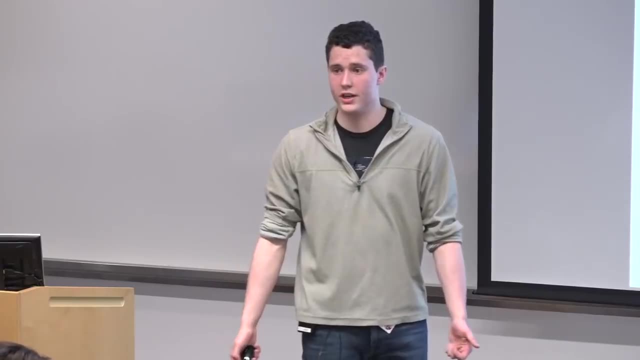 So every time that we try to make an approximation of how good each one of these agents are, we get the discounted reward using 1,000 trajectories, which is pretty good. You can get a pretty good estimate of this. But when the agent is actually learning, 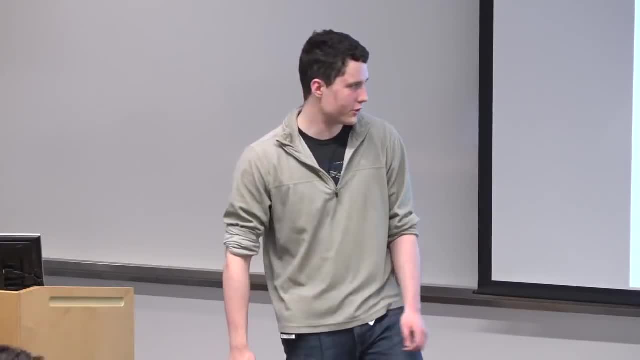 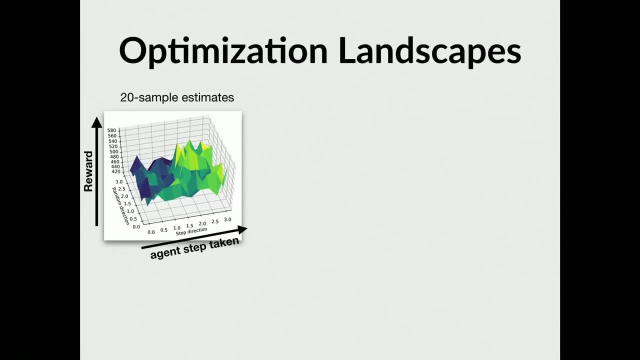 it only uses about 20 trajectories. So what does the agent actually see when we're going throughout this optimization process? So these are 20 sample estimates, which means that each one of these points correspond to taking 20 trajectories per reward estimate. So you take the step. 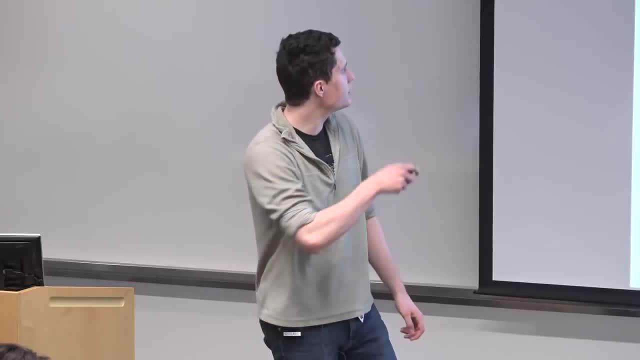 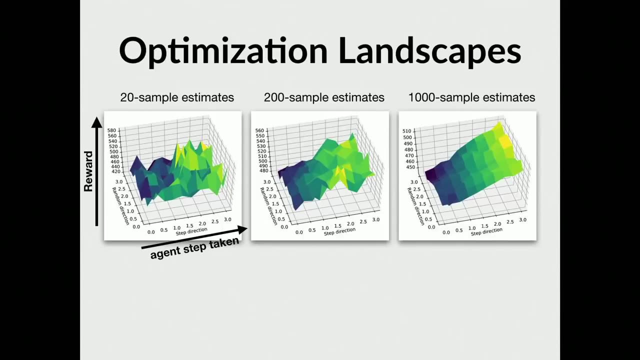 you look at this new agent, then you run through 20 trajectories and then you see what the mean discounted reward was, the mean return. Then this is what happens when you take 200 samples at every point. This is what happens when you take 1,000 samples at every point. 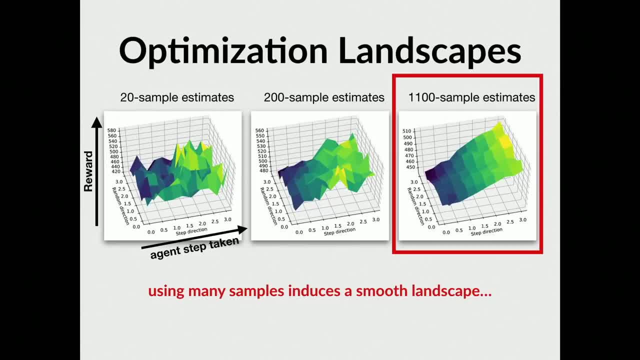 So you can see here that if you use many, many samples, you get a really nice, smooth landscape. But this improvement is so if you move in this direction. even though you're definitely actually improving these rewards, it's a little hard to detect in the agent sample regime. 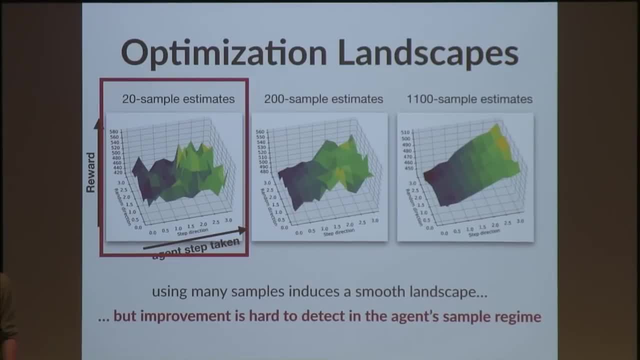 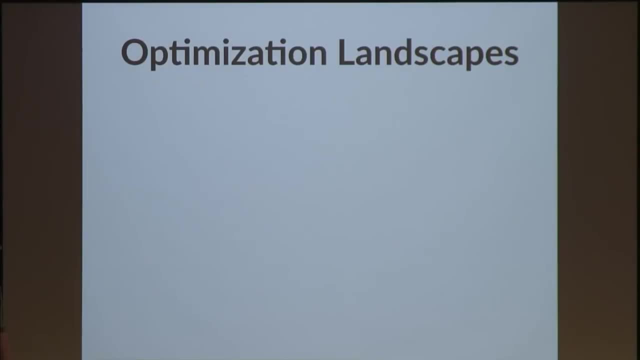 This is concerning because this is what the agent actually uses to make steps. So it's hard for the agent to even know if it's making progress because of how noisy this landscape is. So the two key takeaways here are that, first, these landscapes are not very 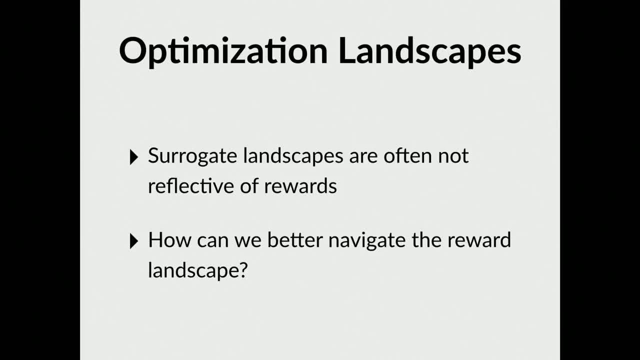 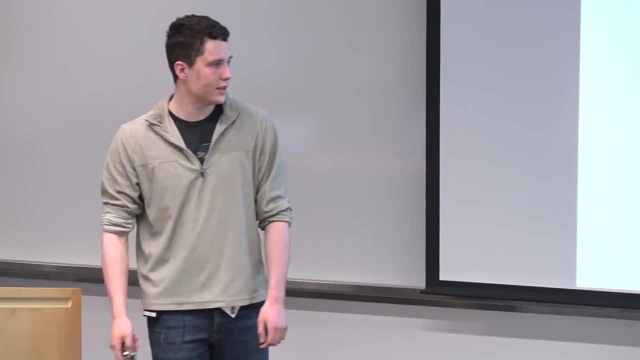 reflective of the landscape. They're reflective of the true rewards and it'd be great to understand why and how that impacts the optimization process. It would also be great to understand how we can better navigate the reward landscape, because it seems like the circuit reward maybe is not the best way to do this. 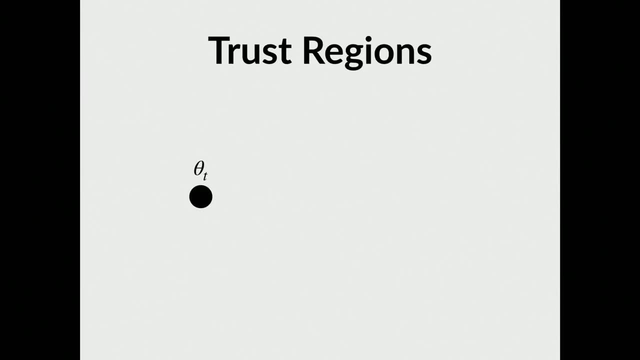 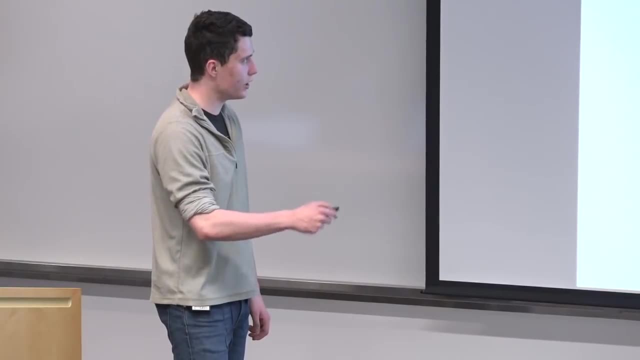 The final aspect of these policy grading methods that we're going to look at is trust regions. So in parameter space you can think of our optimization process as follows: You have this original point in optimization space, then you take a step and you go to the next point. 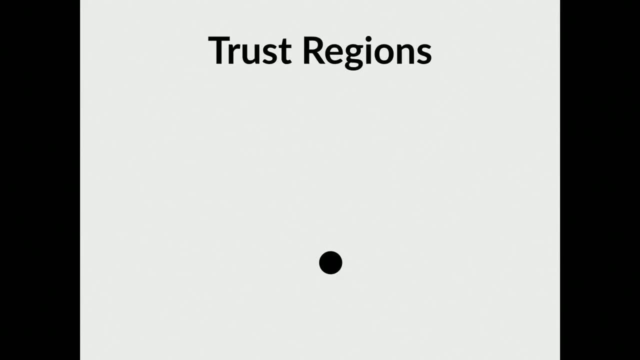 you take another step and you go to the next point, so on. At every step, what happens is you take a bunch of trajectories and you make sure that the step that you take, based on those samples, is within a trust region. So each one of these steps has to be within 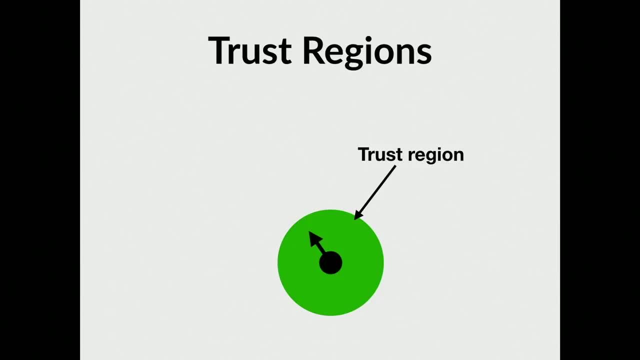 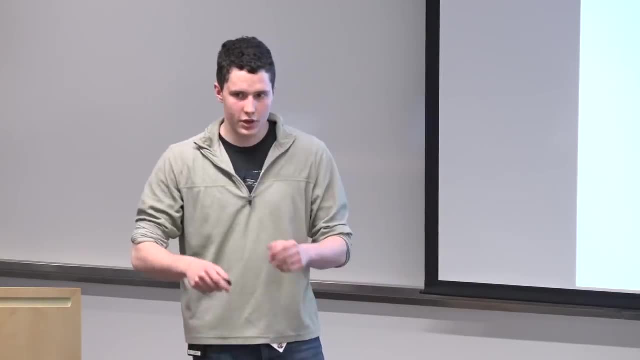 this trust region because the samples that you take are only informative locally, around where the current agent is, because that's where you took the samples. So you want to make sure that the steps that you actually take are actually informed by the samples that you took. 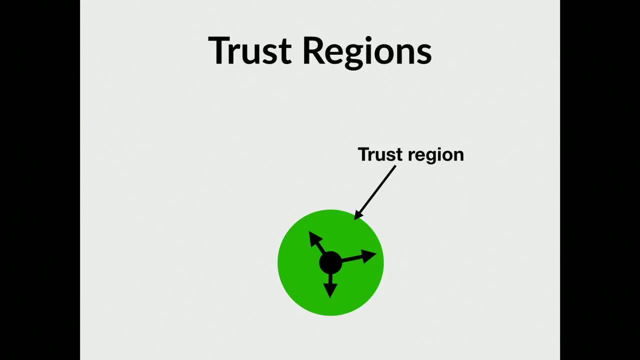 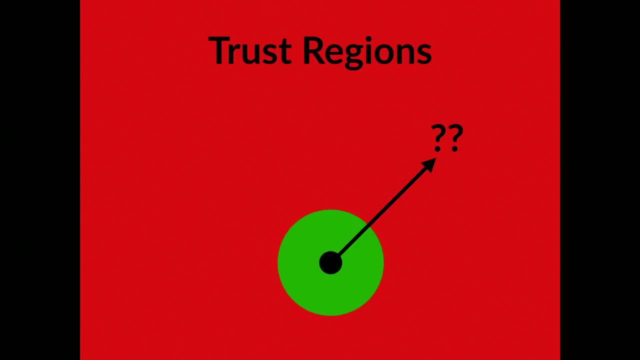 So the idea is that you want to be able to take steps in this trust region, but if you go outside the trust region, then it's a little unclear about what you're actually going to get, because you didn't take samples there. you took samples here. 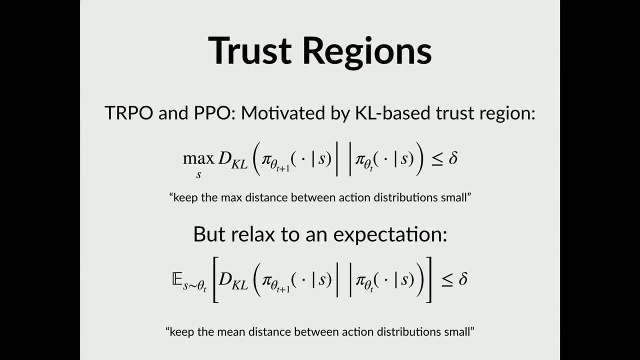 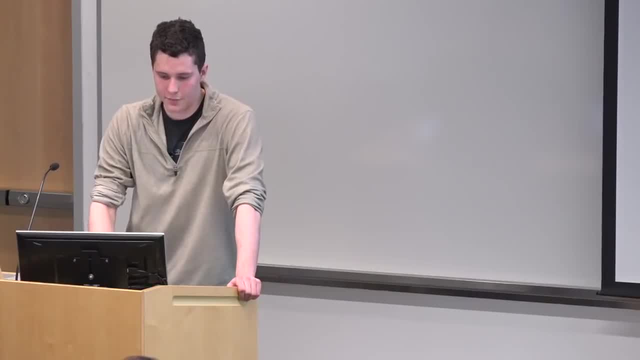 So what PPO and TRPO use? they're motivated by this KL-based trust region where you're looking at the maximum, maximum KL, KL distance between the action distributions induced by states. So intuitively you can think of this as make sure. 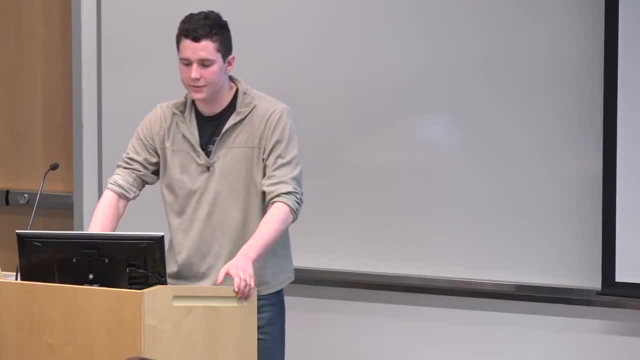 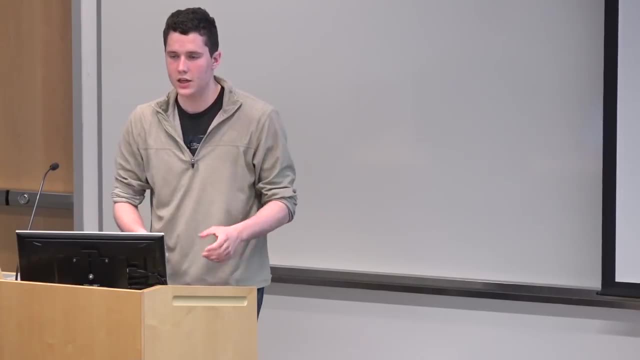 that, even across all the states that you could possibly see, make sure that the way that I choose my action is not too different from my current policy to my next policy. So when I take a step, I want to make sure that in my next policy 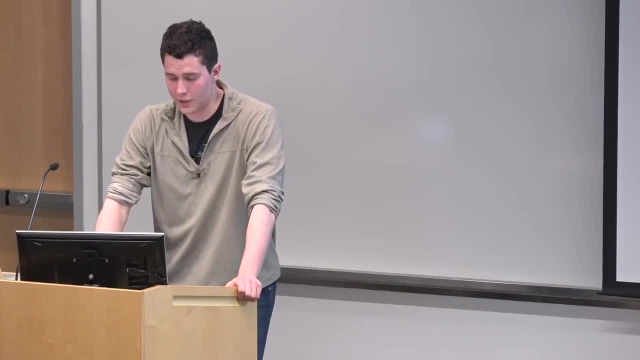 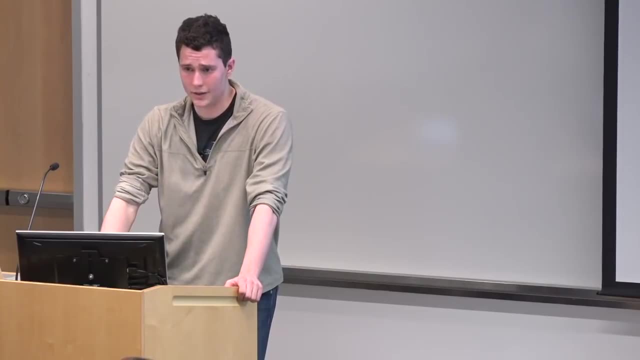 it's not going to be too different than the way that I take my steps and the way that I take my actions, Even across all the states. But this is hard to enforce in practice because we don't see the whole state space. So instead, what we do is we relax to an expectation. 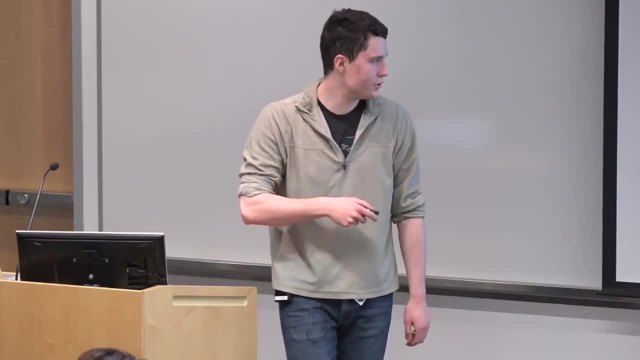 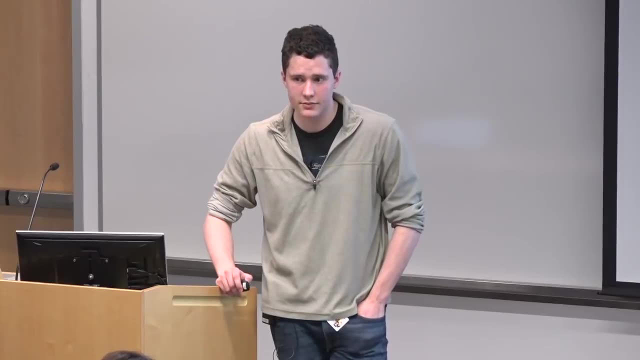 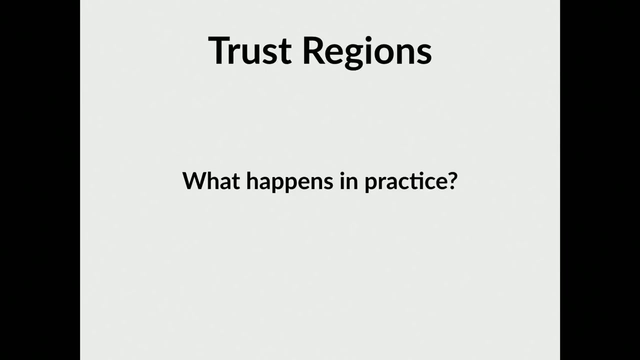 and what we see here instead is we want to intuitively constrain the mean way that we take actions at every state. Does this make sense? So what we want to see here is what actually happens in practice. Does our next agent actually satisfy this constraint? 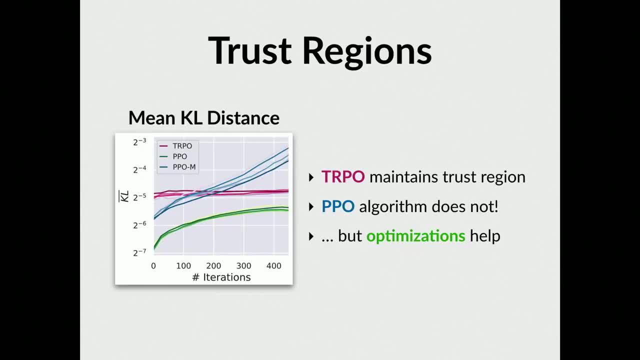 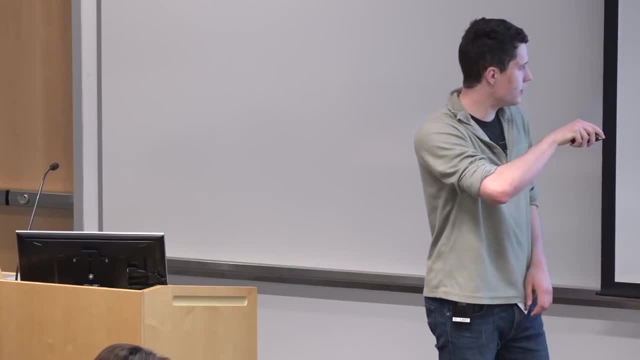 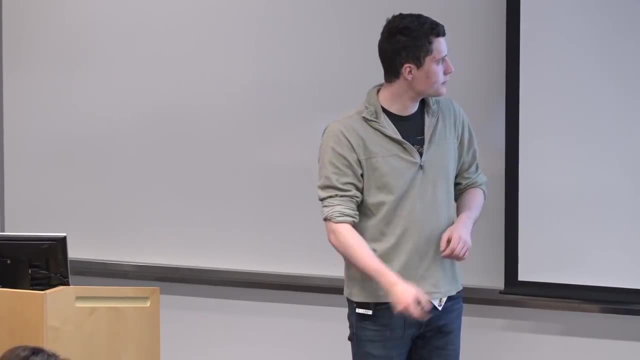 And so right here is. this represents the iteration in our optimization process. So there's 450 steps and we're going to look at every step. we're going to see what the mean KL distance was between our current agent and the next agent. 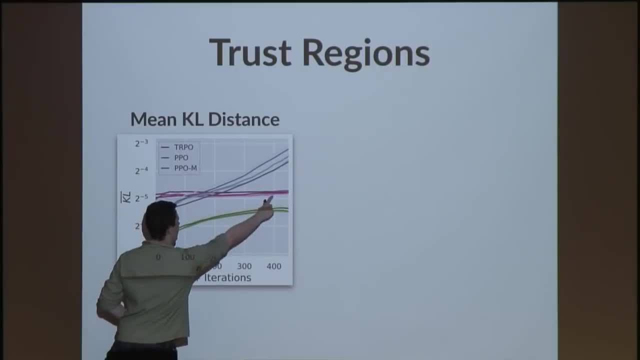 And so it should be around here, which is what TRPO gets, and TRPO actually does this very nicely and it really maintains the trust region. Is everything clear? so far, It's great, Okay. So what the PPO algorithm does not? 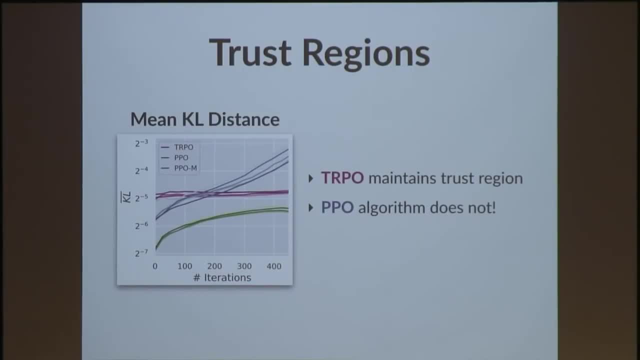 So you can see here that we go from two to negative six KL mean KL to two to negative three KL across the point of training, and it doesn't look like there's any sign of stopping. But interestingly so, the optimizations help quite a lot. 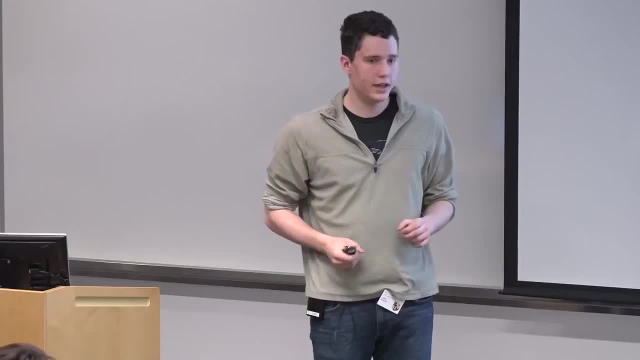 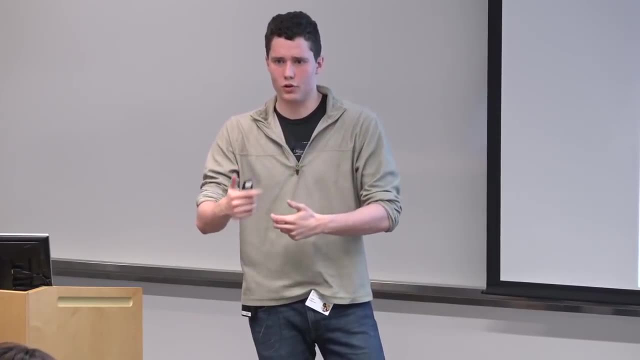 So we have this core PPO algorithm and it purports to keep this mean KL the same, or it has a relaxation, but it purports to. this is the overall goal of this algorithm is to keep this mean KL the same while relaxing this constraints computationally. 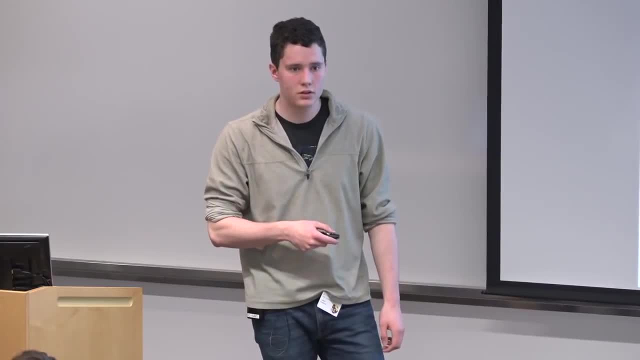 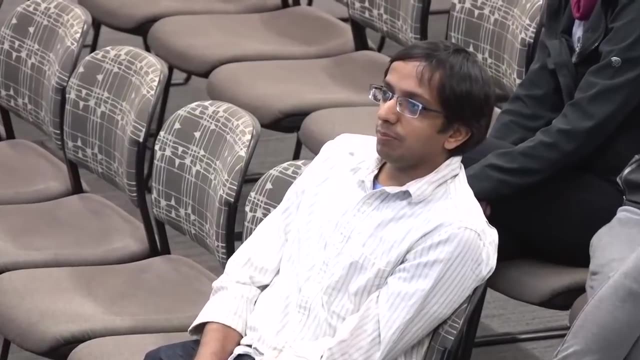 so they're easier to compute. So is it just the loss in Taylor approximation, the going from two to the minus five, to two to the minus three? I'm sorry, what Like PPO is using a more approximate form, right? So I mean there is going to be a loss also, just 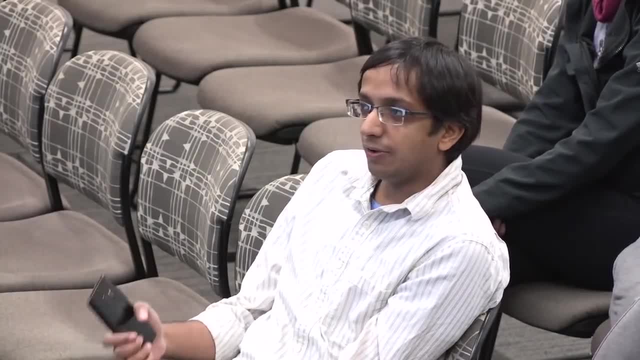 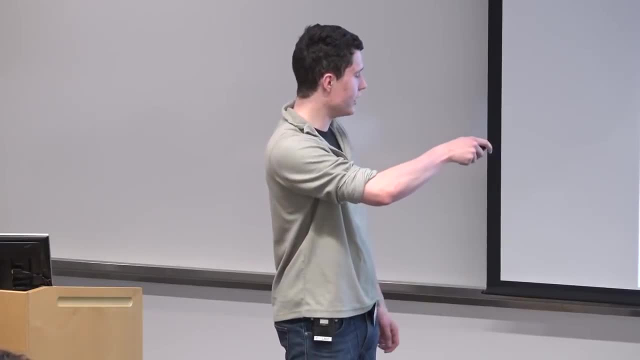 from Taylor's approximation, that's invoking Yes, And do you have a sense of whether it's all attributable? Yeah, So that's really interesting. Yeah, So that's what we're looking at right here is the fact that this algorithm and 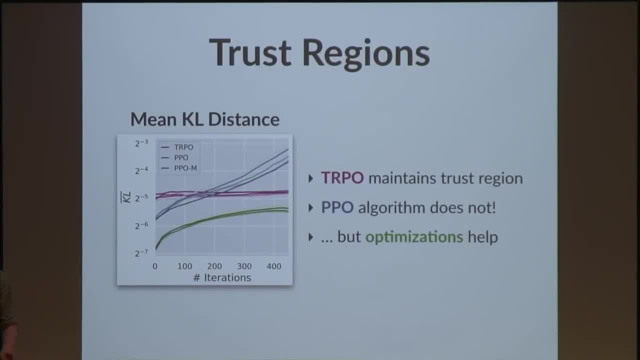 this algorithm use the exact same enforcement method. Like these two methods in terms of, if you just read the paper, you would think that these would enforce. this mean KL just as well, because they use the exact same enforcement method. But when you put all these different optimizations on top of PPO, 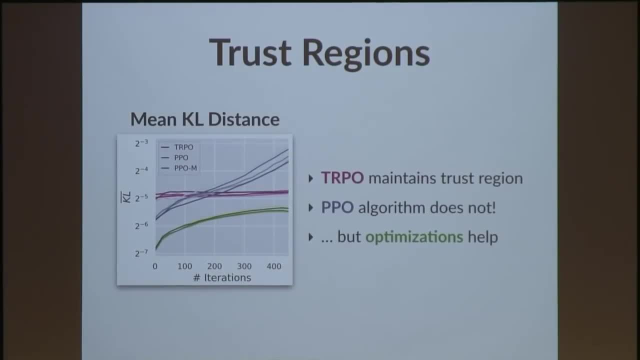 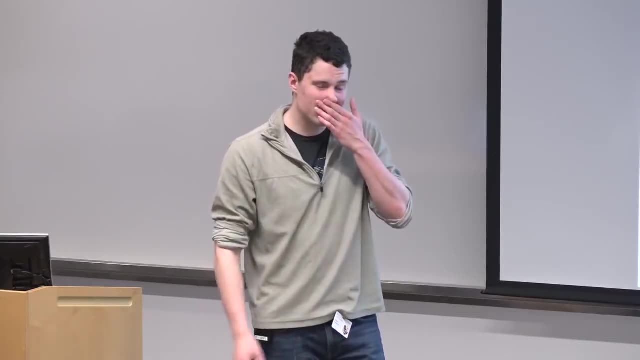 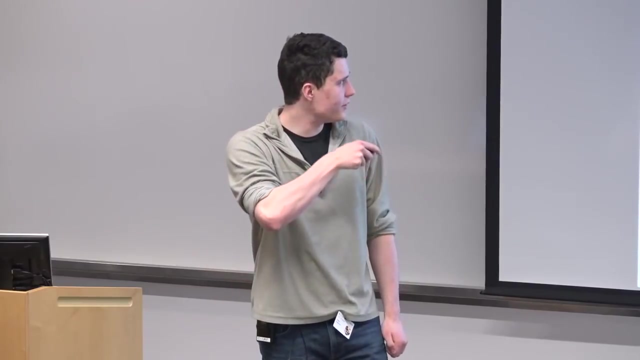 it turns out that you can get significantly better trust region enforcement. These optimizations include like learning rate annealing, like value clipping, and so on, and using like orthogonal weights, and so on. So it's unclear exactly what is causing this trust region to be enforced. 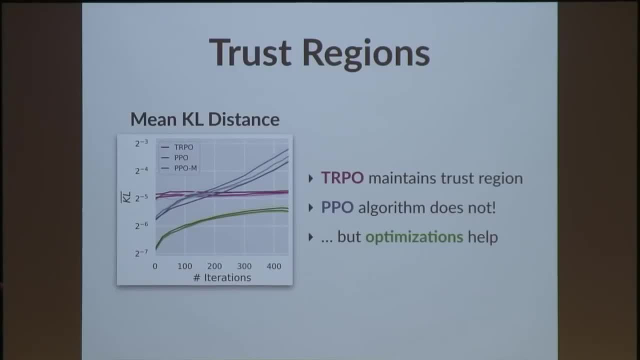 but this trust region not to be enforced because they are the same algorithm. So this is PPO, green is PPO and this blue one is PPO-M, which is like PPO minimal, which is what you would get if you just implemented the PPO algorithm. 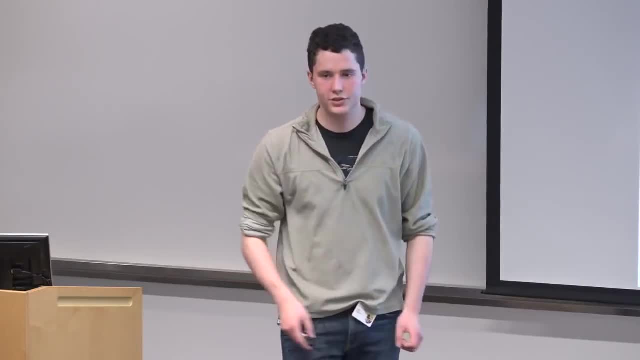 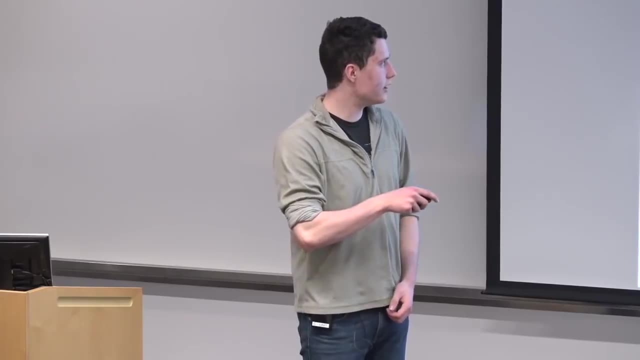 as stated in the original paper, Then this is what you get when you use all the different optimizations that you find in the OpenAI GitHub repository. So what's interesting here is that, even though the enforcement method mechanisms- if you just looked at the algorithm- 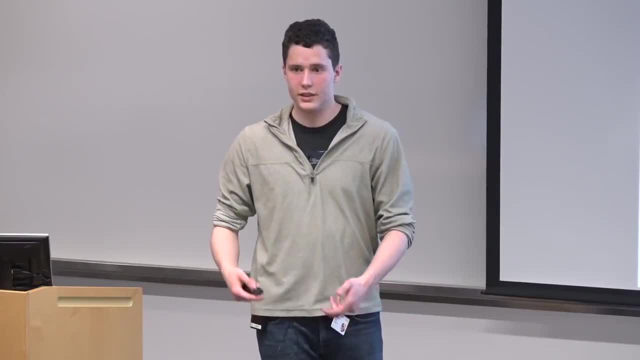 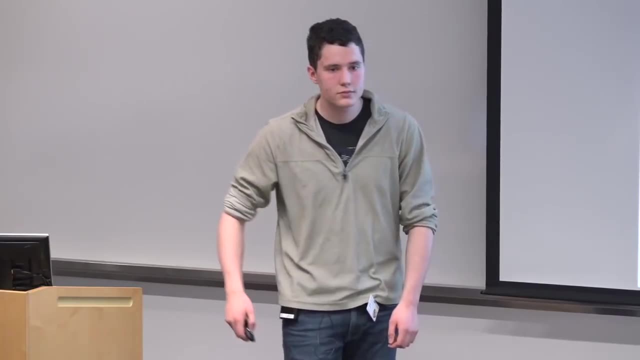 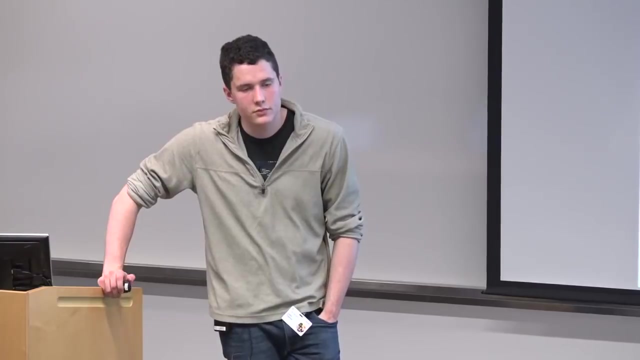 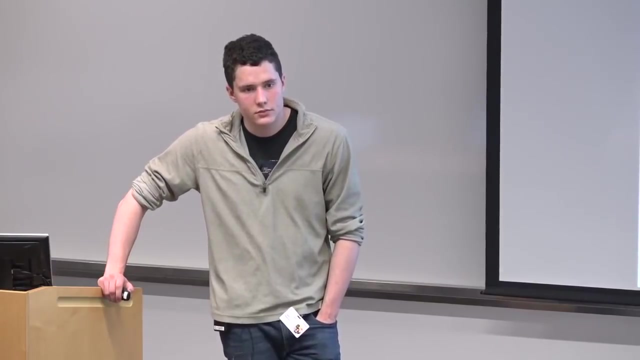 appear to be the same. the optimizations cause the actual enforcement and practice to be drastically different along these two algorithms. I mean, this part is not as surprising just because presumably a lot of the optimizations were done to actually stabilize the numerical aspects and at least if your policies are changing in a more stable fashion. 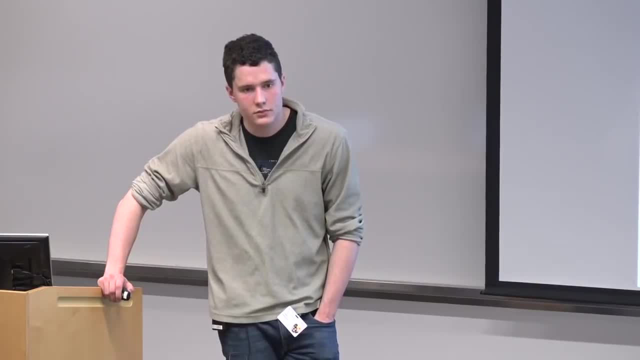 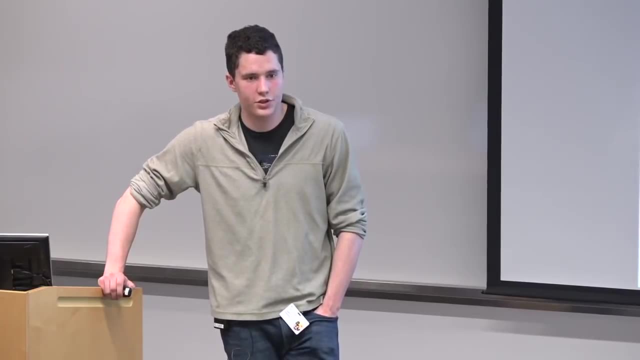 then, by definition, trust regions are going to be better maintained as well. So what they optimize for here is not: they aren't trying to make anything more stable. What they're trying to do is maximize total rewards at the end. right, Right, But they're presumably trying to do it in. 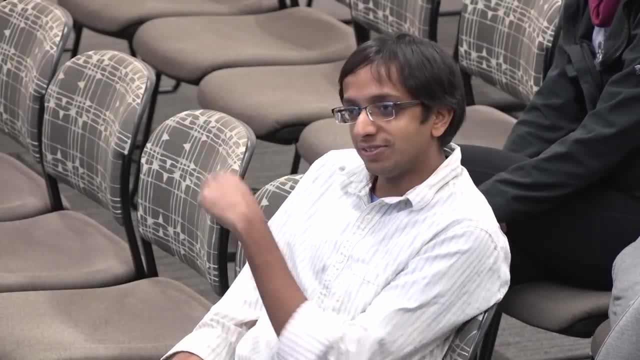 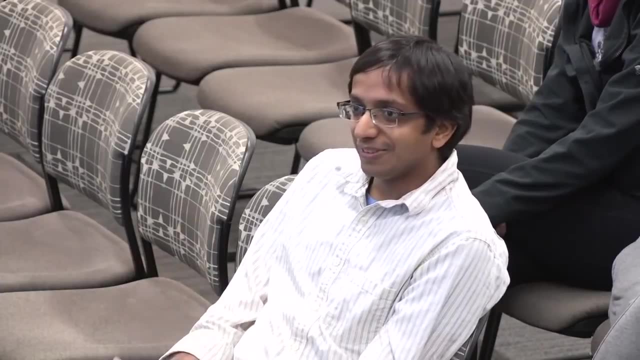 a somewhat more reliable way, In a more reliable manner across the different tasks that they're evaluating on. So it might very well be an artifact of Right. It could be an artifact of that optimization. I guess what's interesting here in general is that 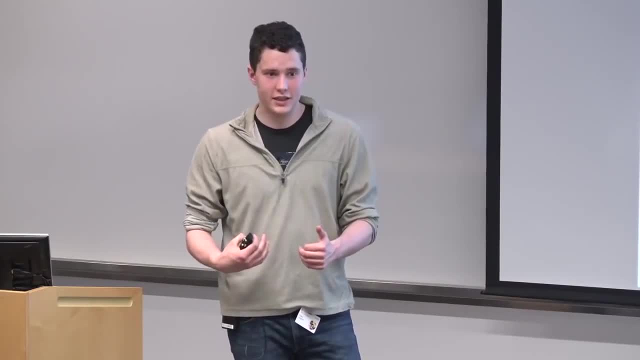 I don't know, maybe this is just me, but when I look at the optimizations that I don't see like maintaining trust regions at all in any of them. Like the only mechanism that I actually see in the algorithm for maintaining trust regions is like: 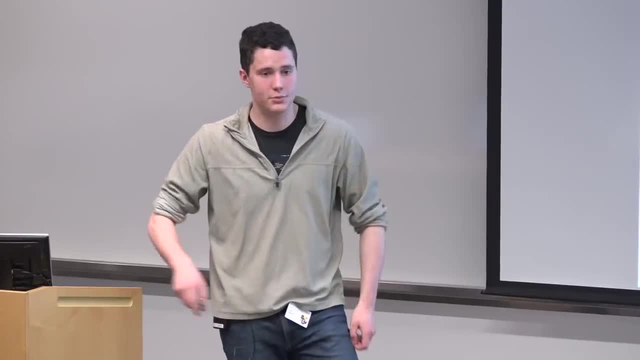 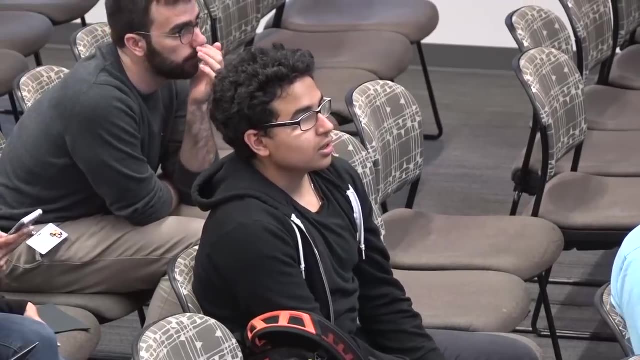 the key PPO like ratio clipping thing which is kept constant across both of these. So isn't it interesting that like, or at least it's somewhat surprising to us that like the mechanism that's designed to maintain a trust region does not seem to be? 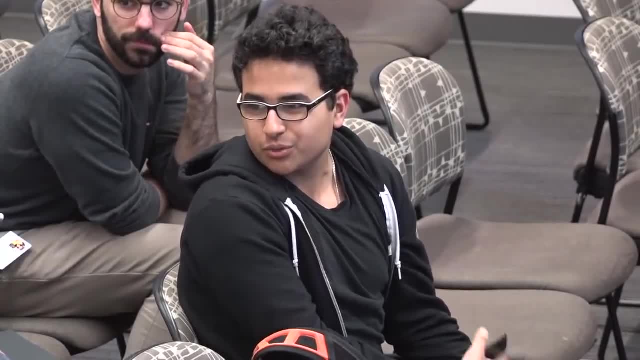 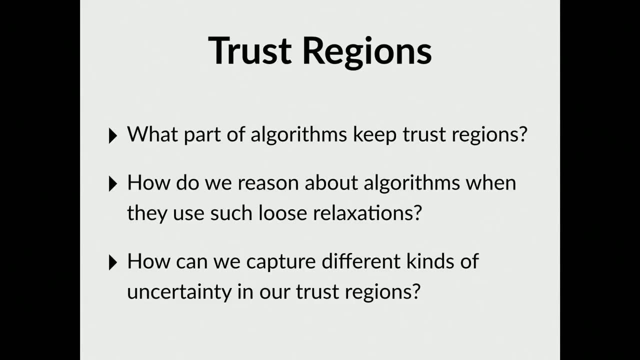 the thing that's actually maintaining the trust region. It seems to be like some other stuff that we added on top. So I guess, as we just talked about, one of the key questions to ask here is what part of these algorithms are actually doing what. 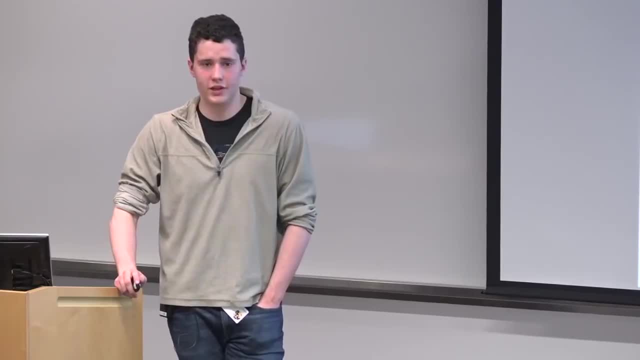 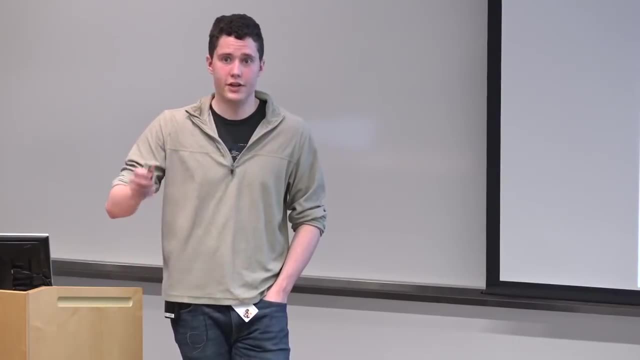 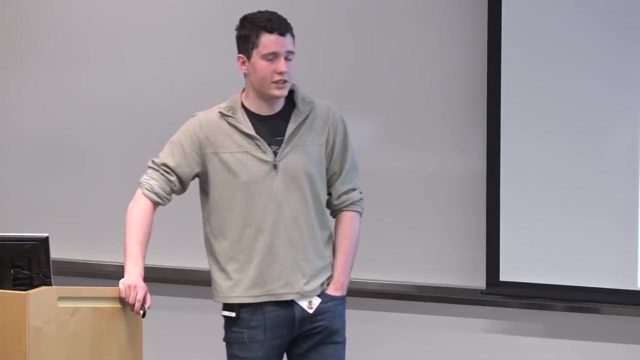 How do we reason about these algorithms when they're using such loose relaxations to the original trust regions that they were supposed to be theoretically- at least in terms of theoretically- groundedly- using? Not only that, but how can we capture the different kinds of uncertainty that we have? 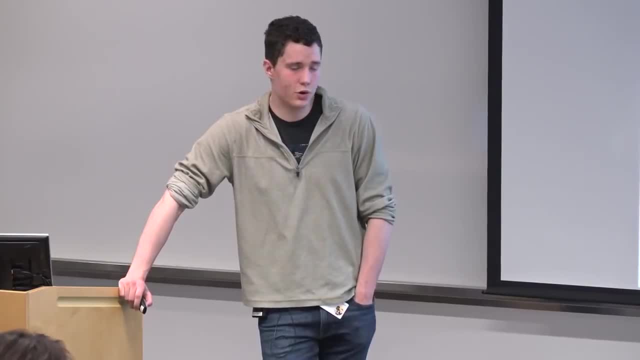 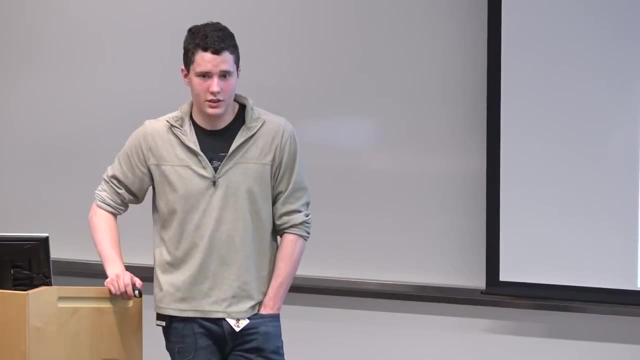 in our algorithms, in our trust regions. So the original trust regions that motivate the trust regions that these deep RL algorithms use don't take into account stuff like bad value functions or really unconcentrated gradients and so on. So it'd be great to see what kinds of trust regions 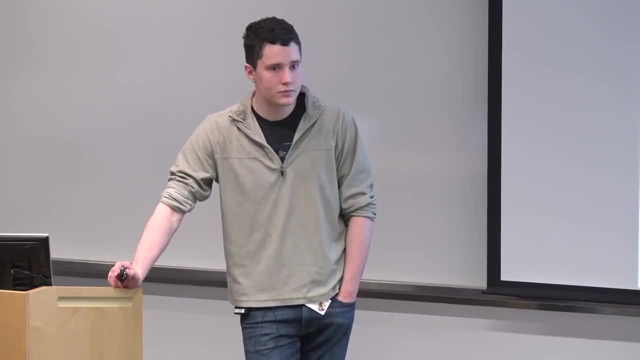 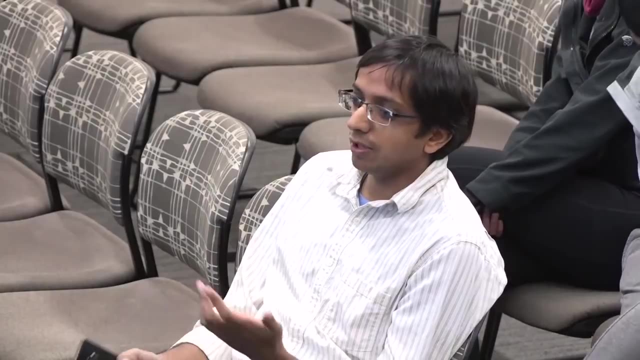 we can come up with that. take these into account. I guess the difficulty I'm having with this part is so. PPO is fundamentally like: once you do a Taylor approximation of KL, sure you could still go back and measure KL, which is what you're doing. 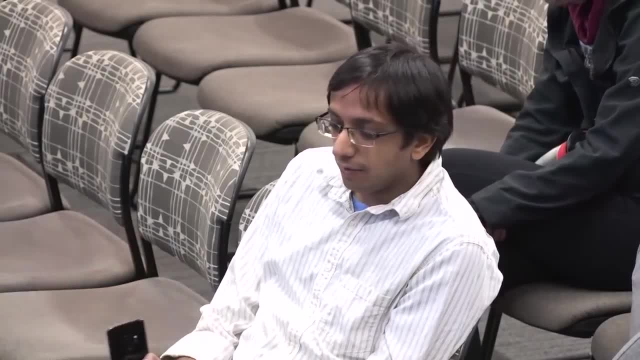 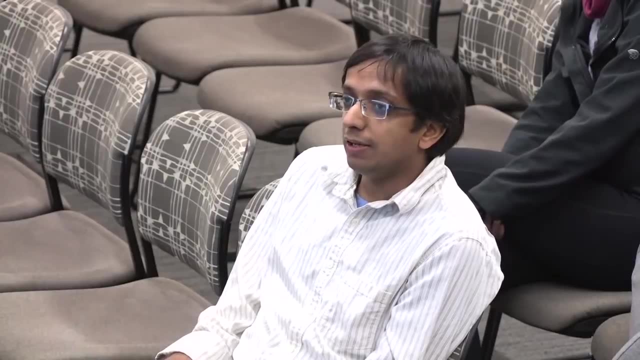 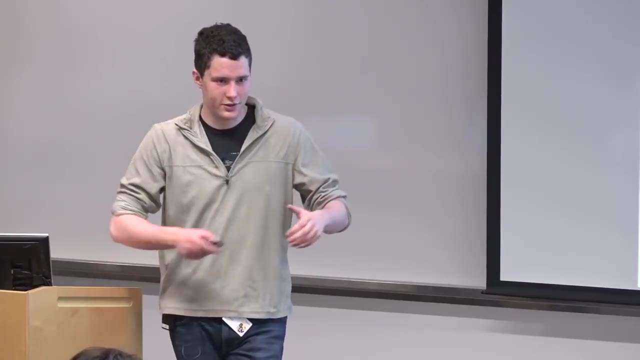 but you could also say that it is just defining a different notion of what a trust region should be. and what do things look like if you actually just evaluate what PPO is enforcing? Yeah, We actually looked at that too. I didn't choose to include that in the slides because I didn't want to. 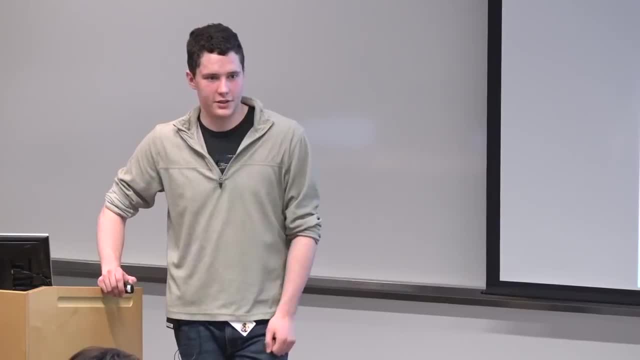 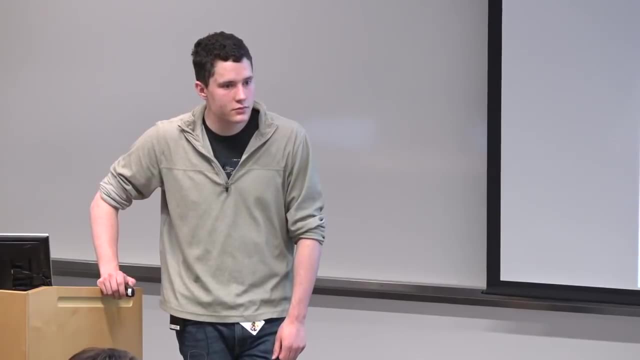 I thought it would be too much, I guess, but I'm happy to talk about that. We have that in our paper. Sure, What's the main takeaway from this part? Because all of these, I mean even the PPO paper. 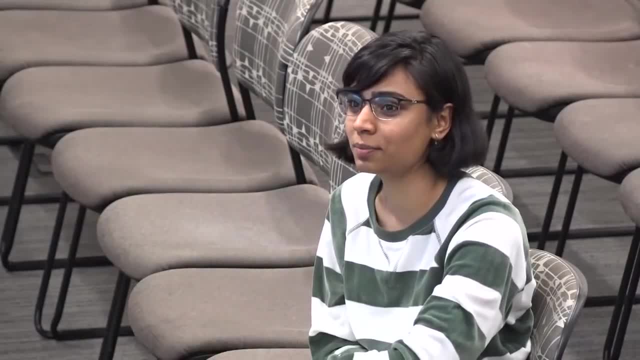 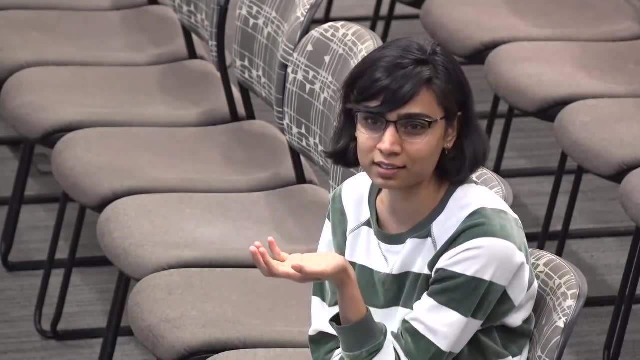 they say that, yeah, we use like a very loose relaxation, but empirically we observe success, which is essentially what this section of the presentation is also saying- But it doesn't seem to be due to the relaxation. You could just not have the relax. 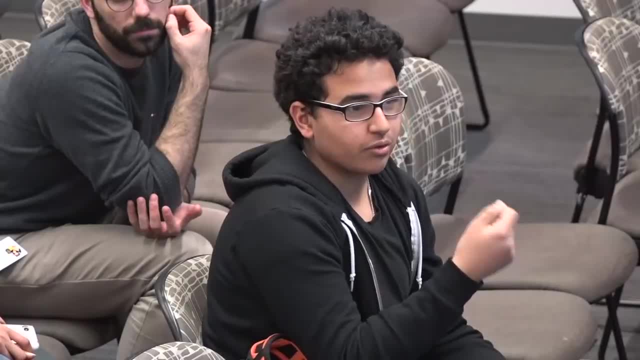 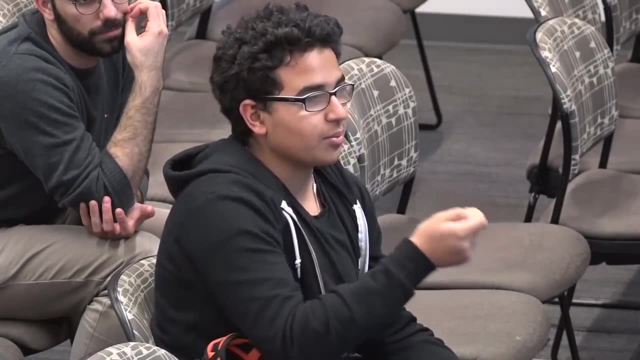 It turns out that if you just remove the relaxation that PPO does, but you do all the optimizations and you do them slightly better, you can just enforce the same trust region. So the whole clipping thing, you can just set the hyper-parameters. exactly right. 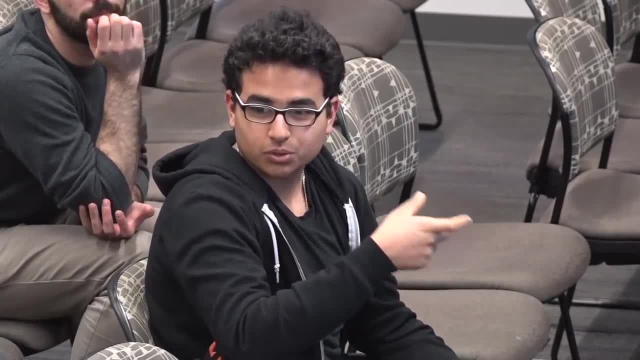 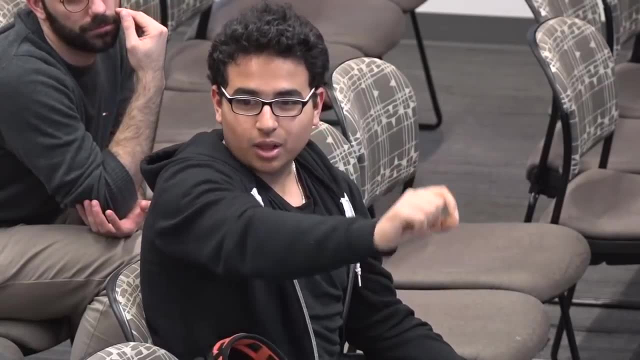 so that it never leaves the clipping thing and then it's all fine. So the clipping doesn't actually seem to be doing it. It's more like the optimizations that we added on top of the clipping thing make the optimization so nice that you don't actually need the trust region in the first place. 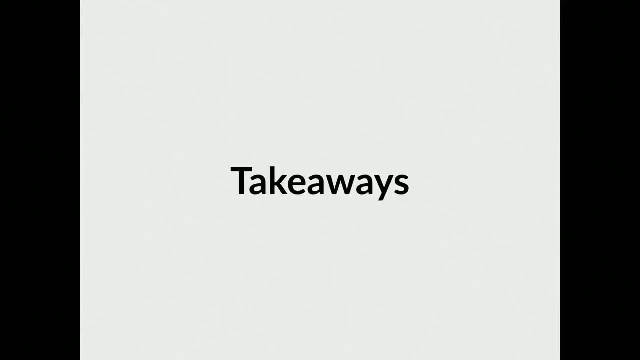 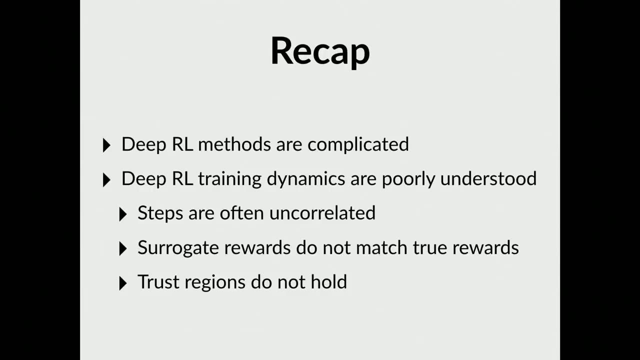 So just general takeaways that we can get from this. In general, these deep RL methods are really complicated and they have a lot of moving parts and they're hard to understand. Not only that, but these deep RL training dynamics are really poorly understood. 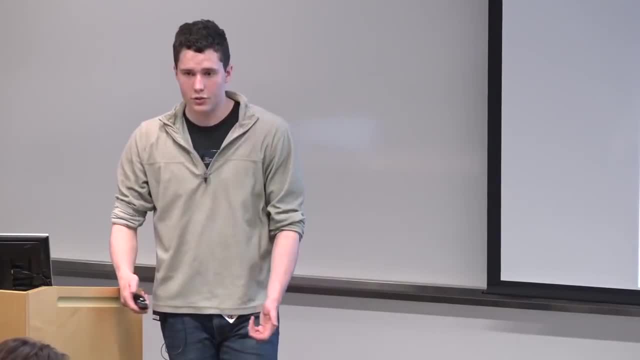 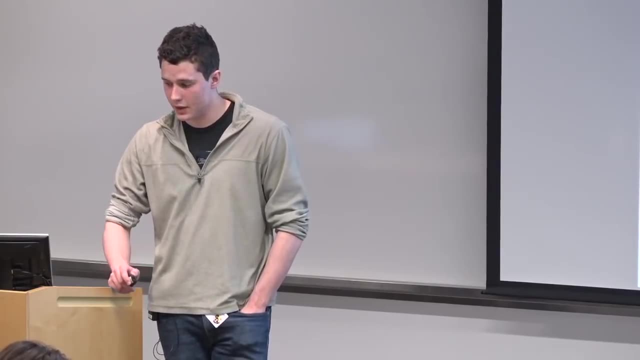 The steps that we take are often really uncorrelated. The surrogate words don't match the true rewards and the trust regions don't hold, oftentimes, at least for the reasons that we think. So the question is: the big question here is: how do we proceed? 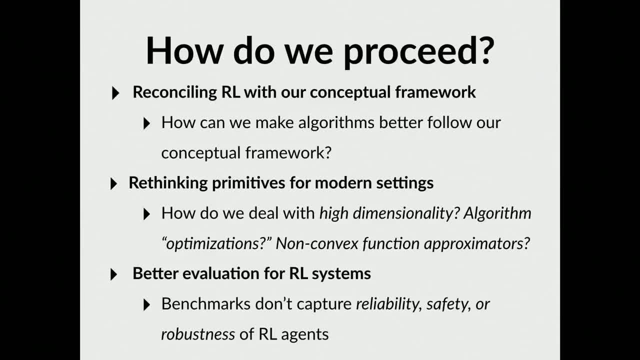 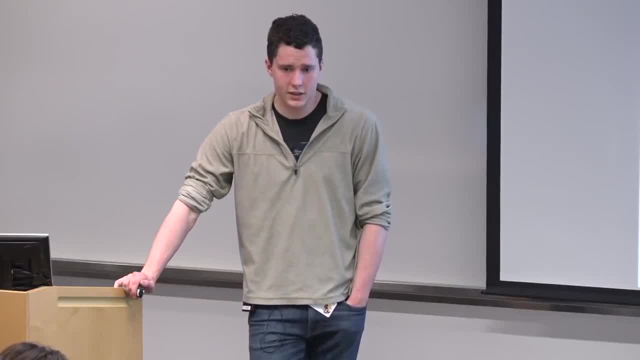 What are we going to do in the future about this? So the first thing that we might want to do is try to reconcile RL with our conceptual framework, try to make our deep RL algorithms actually match the policy gradient framework better. So how can we do that? 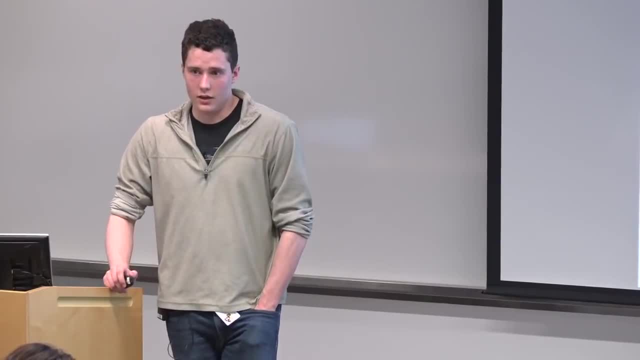 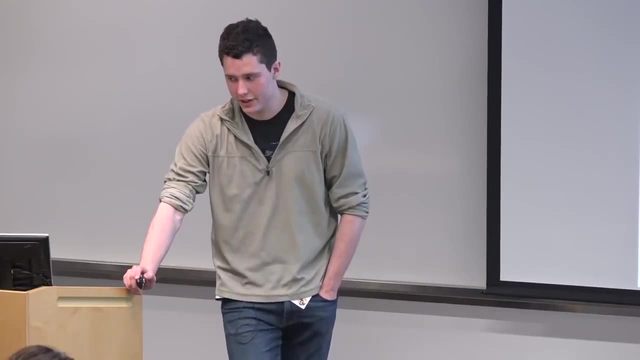 Another step that we could do is try to rethink our framework for these deep RL methods, try to move our framework closer. So for that we would have to figure out how to deal with high dimensionality and these algorithms, different kinds of optimizations that they put on top of. 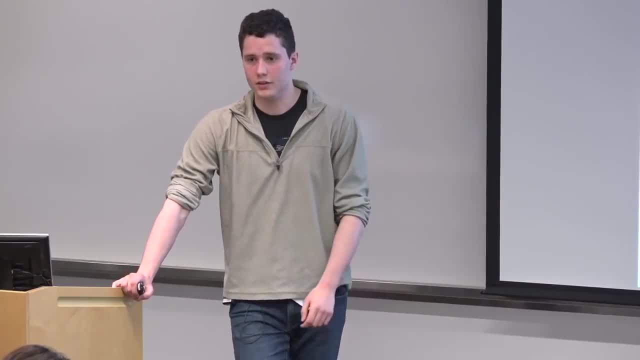 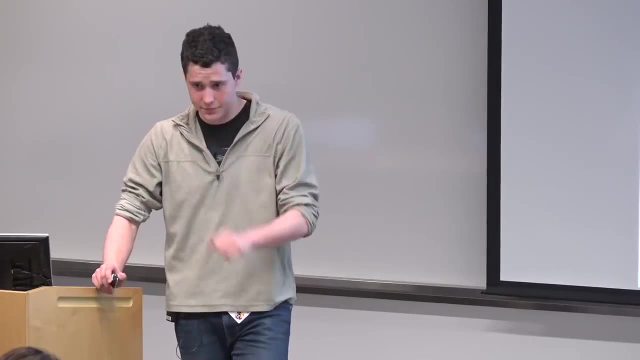 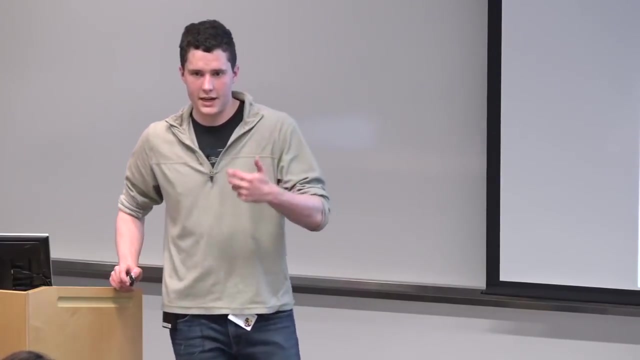 the on the core method and not only that, but dealing with these non-convex function approximators and deep learning, deep networks. And finally, our results suggest that we need better evaluation for RL systems. We have to move past a return-based centric benchmark system. 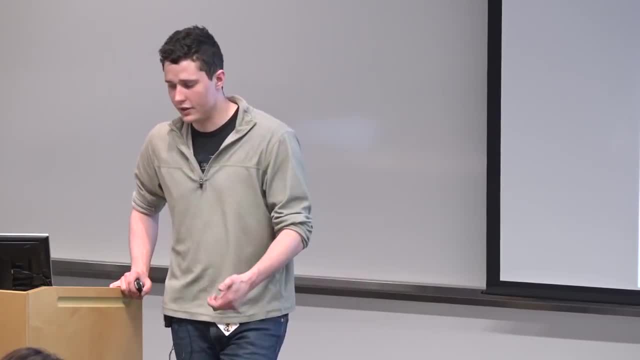 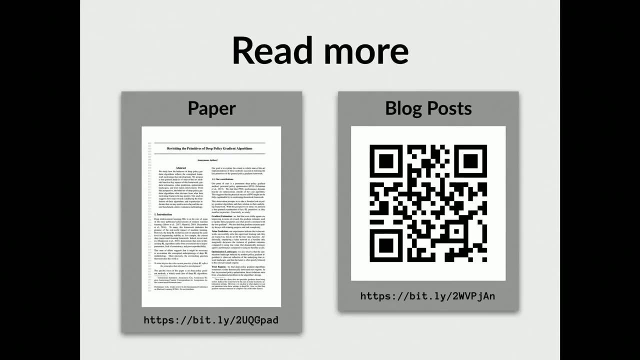 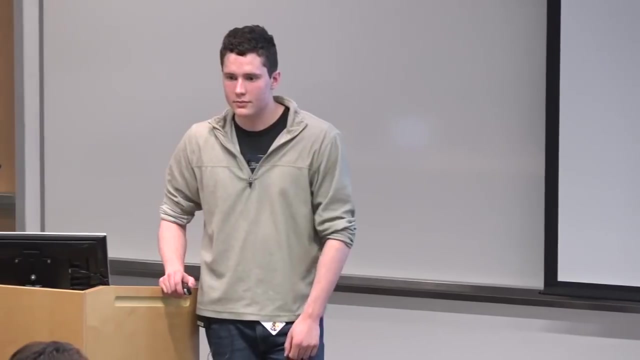 and try to look holistically at all the different aspects of these algorithms, like trying to look at reliability and robustness and safety. And if you want to read more, we have a paper and we also have a bunch of blog posts- More questions. 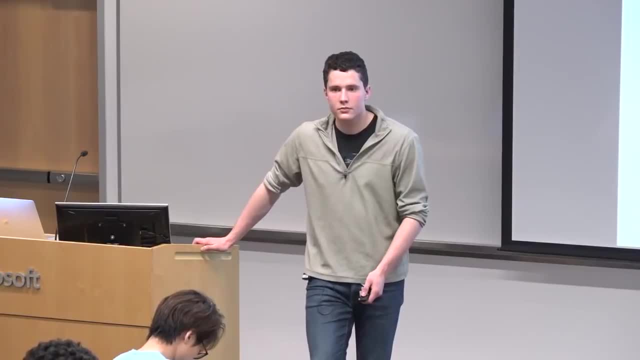 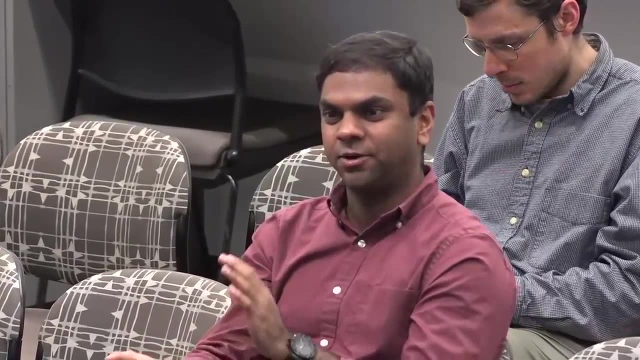 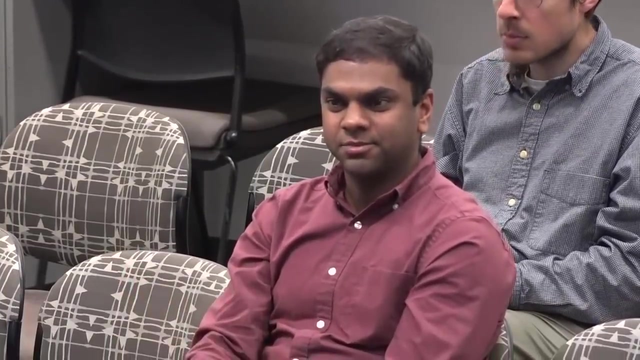 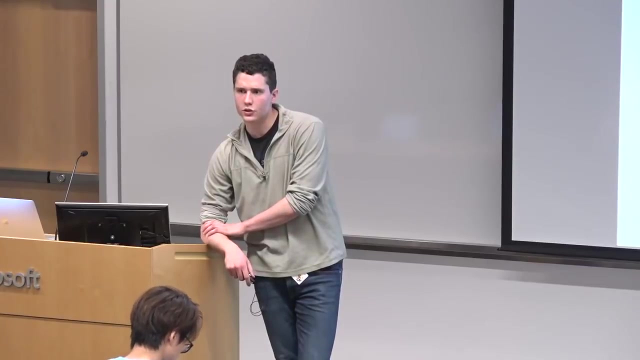 I'm quite curious to see: do you run similar probes on some either bandit-like settings or just supervised settings to see how much the gradient estimation issue or the trust median issue? Yeah, So we actually looked at using SGD to maximize, or one of our buddies looked at maximizing. 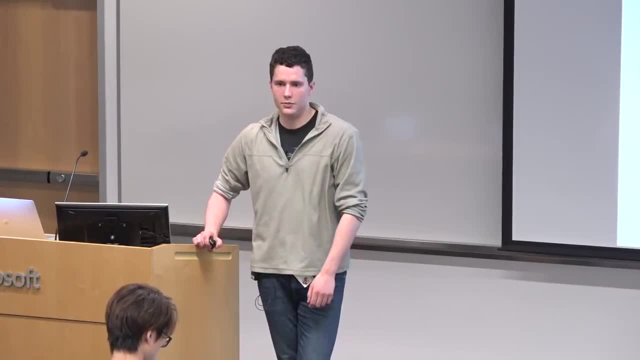 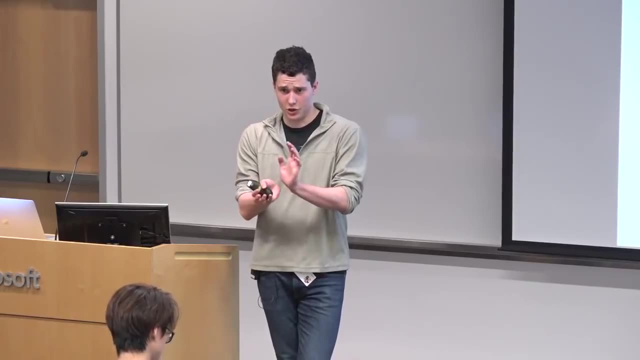 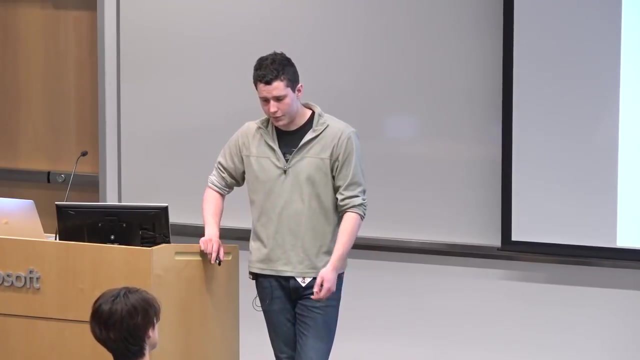 basically just looking at toy settings in SGD, like using SGD to maximize a quadratic or something. So it turns out that you can make this step super uncorrelated. you're still going to maximize the quadratic Pretty well. So we thought that was pretty interesting. 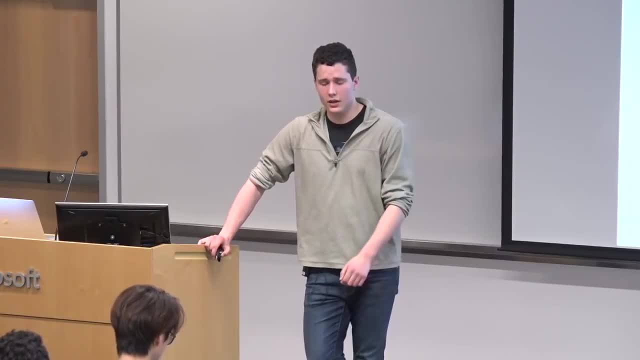 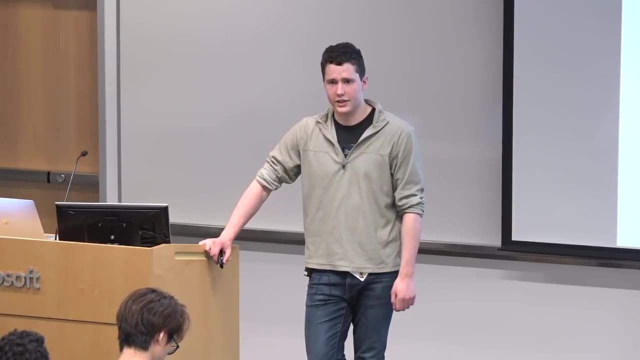 but the dynamics in RL are very different, I guess for the reasons that we mentioned before about lack of independence and non-stationarity. So we've looked at some experiments that are similar in these regimes. I think bandits would be a great place to look as well. 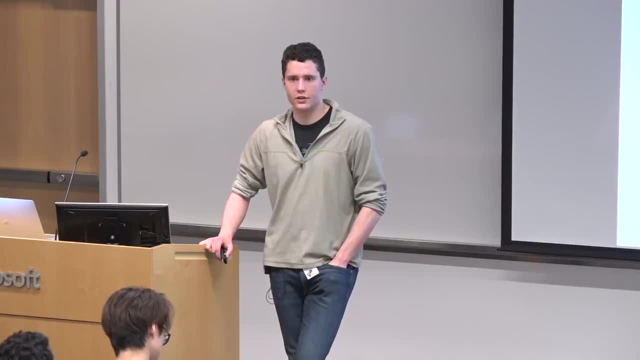 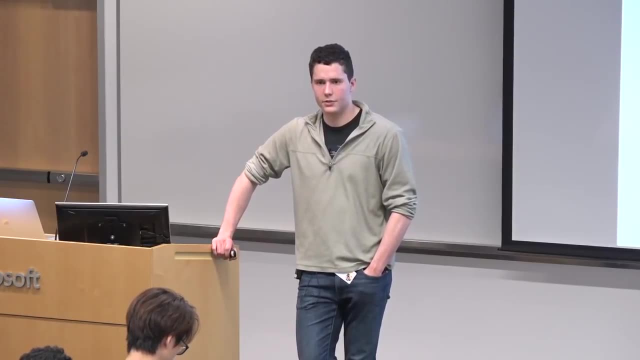 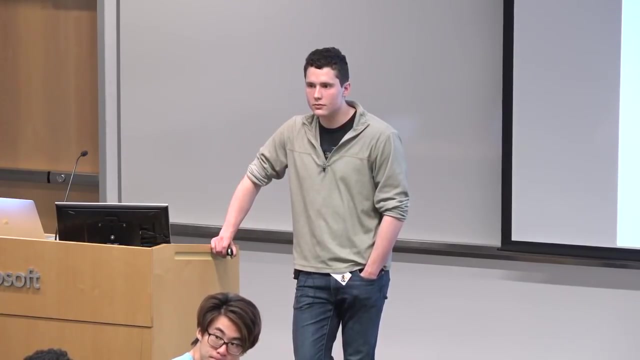 But I think bandits are very theoretically well understood and there's not too many moving parts in them. right, There's a core algorithm, but I think we could look at. I'm just still a little bit confused about the part that your gradients seem to be very uncorrelated. 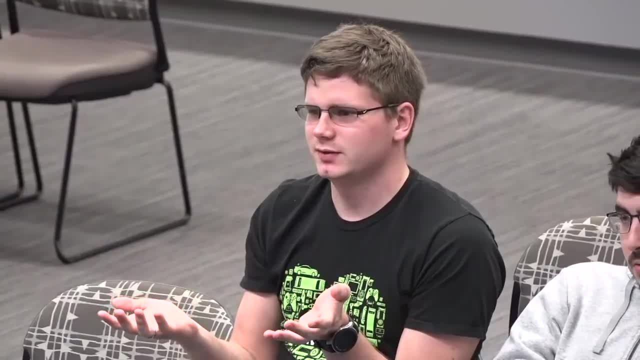 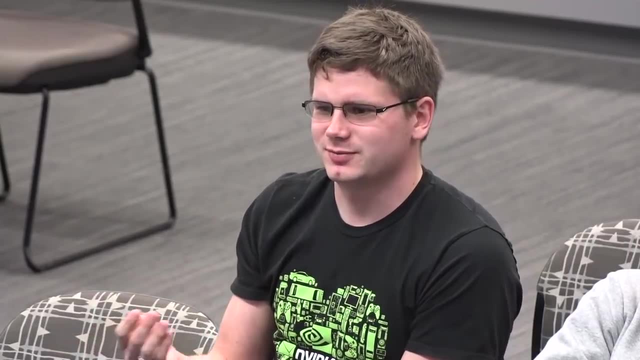 and your reward seems to be going down most of the time. So is it just pretty much like taking random action? What if you actually try to just, instead of following your gradient, just take a random direction and then keep it if it becomes better, or something like that? 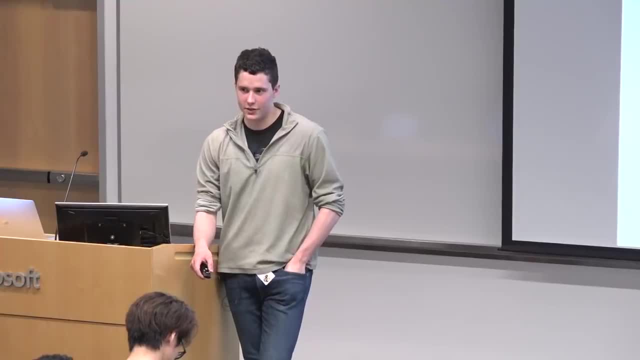 Yeah, So that's actually a technique that people use. that's like finite differences methods. There's a paper from Ben Racht about it, called random Search is a competitive baseline. Yeah, Random search is a competitive baseline for D, bar, L or something. 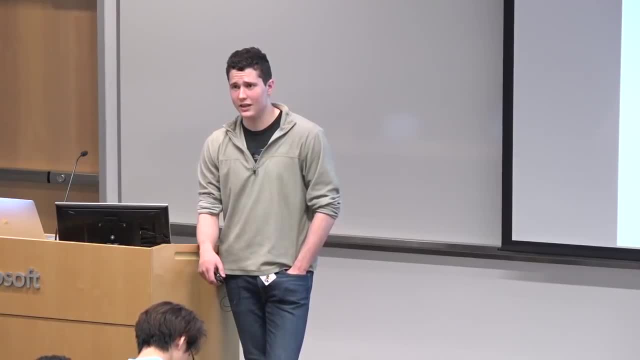 It was a good paper, pretty interesting paper at least. So basically what they do is they just take a bunch of random directions and see which ones do well, and they do a bunch of other optimizations on top of this. They do some wacky stuff about throwing away different directions. 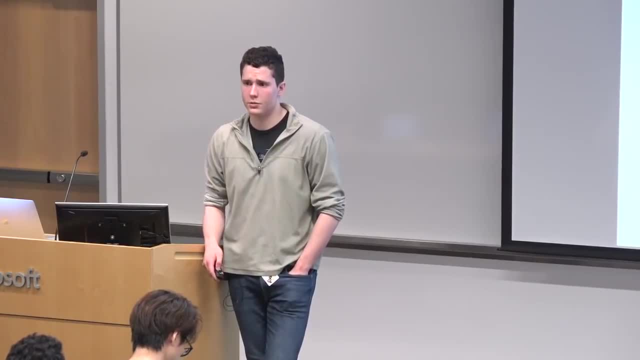 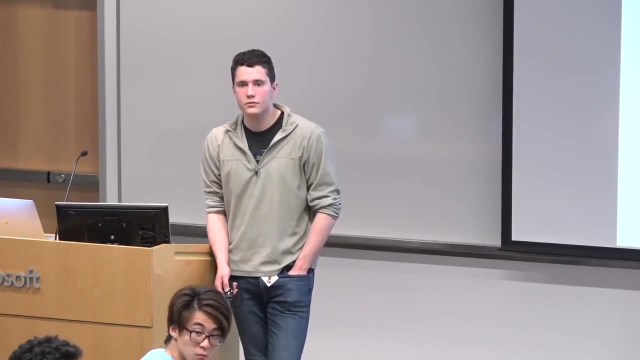 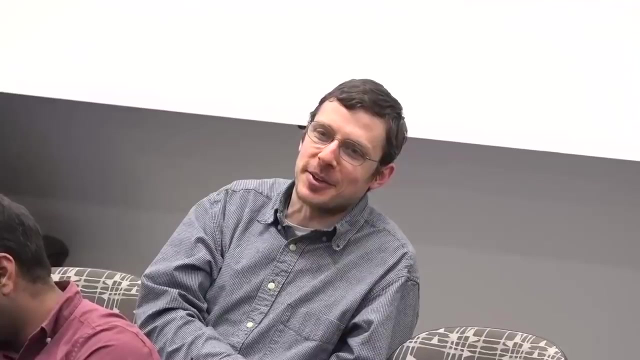 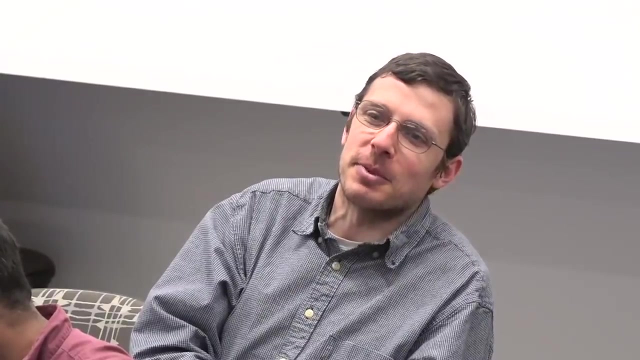 But yeah, it's the same core algorithm and it works pretty well. So if you were going to start from scratch approaching this problem domain, are there things you think you would leave out of the present framework for RL or replace with something else? 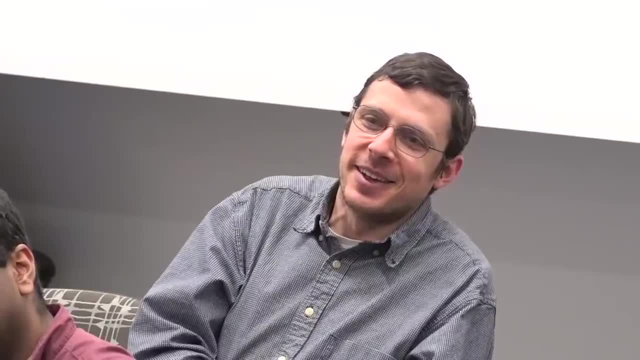 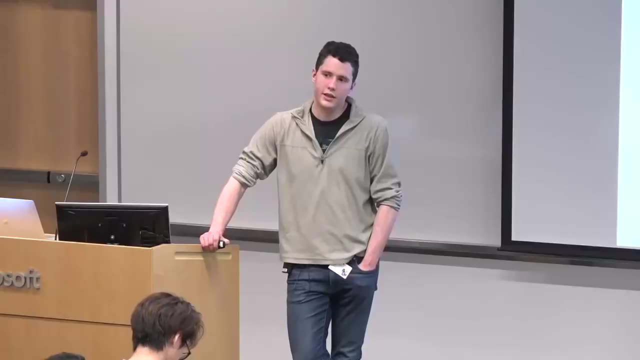 or what kind of ideas do you have about how to avoid having some of these issues at all? Yeah, So I think that it would be great to look at as we design these algorithms. it would have been great to look at how the different optimizations that we use actually impact the performance. 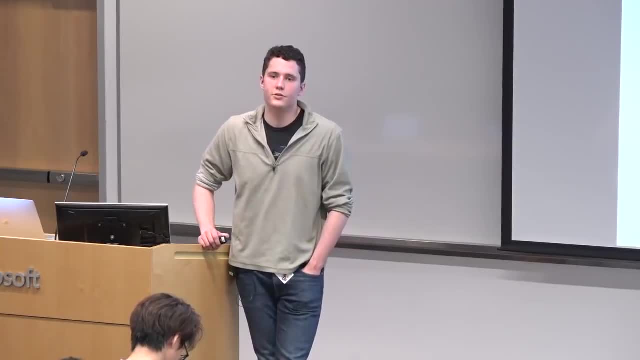 I mean. so the policy gradient, the framework that people came up with, is not intended for the deep RL methods or for these kinds of tasks as much. So I think it would be good to design. I'm not sure, I guess, about how I would design the framework. 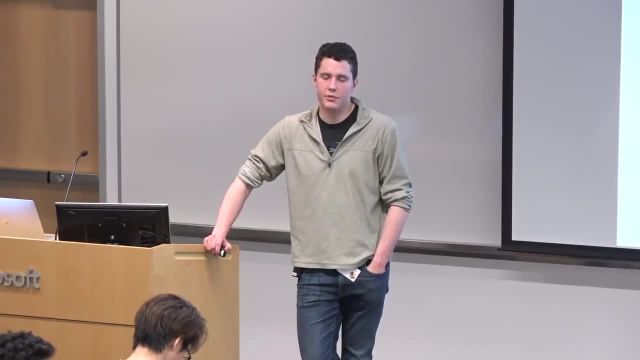 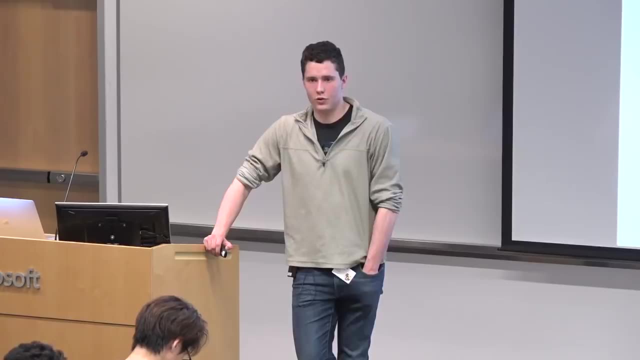 but I think that in general, when developing these kinds of methods, I would be more careful about looking what the impact is of different algorithmic aspects and trying to really understand what's causing performance and what's causing reliability or unreliability or lack of performance. 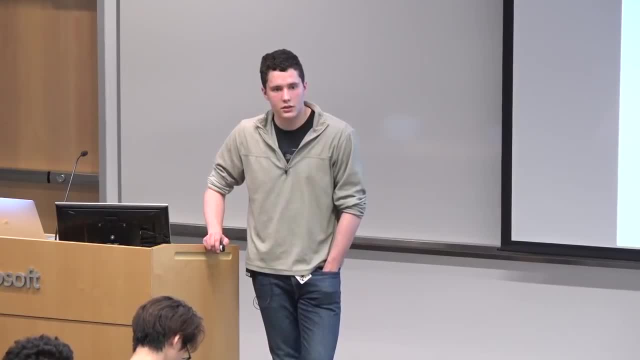 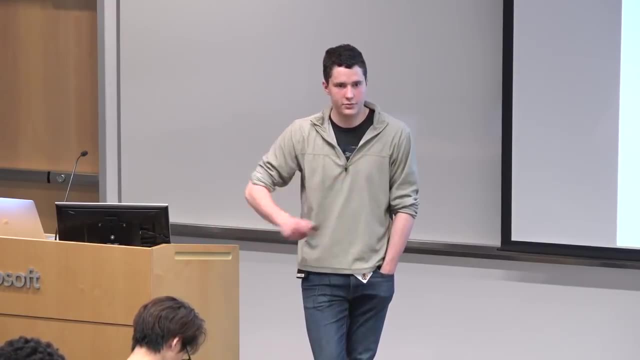 Yeah, Have you tried just using linear model, as in like it's a problem here caused by your network? Yeah, So actually you can solve this without any deep learning using a linear model with these algorithms. Right, I'm saying like, have you done experiments? 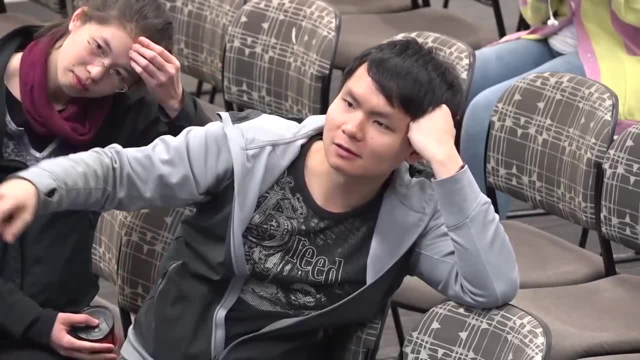 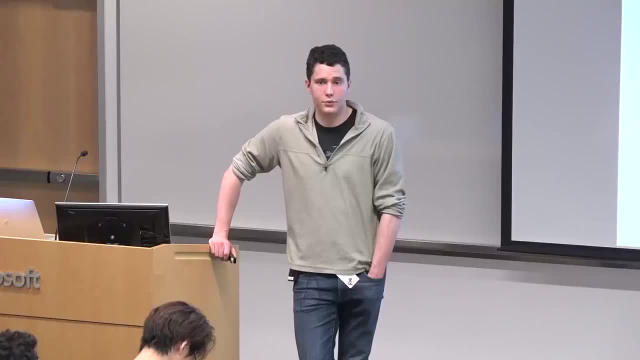 Have we done experiments on this, Like, say, like the optimization landscape, you have a linear function approximator. Does it also look like that? Yeah, That's a great question. I would suspect that these environments would be similar, but I think that it would be interesting to look at. 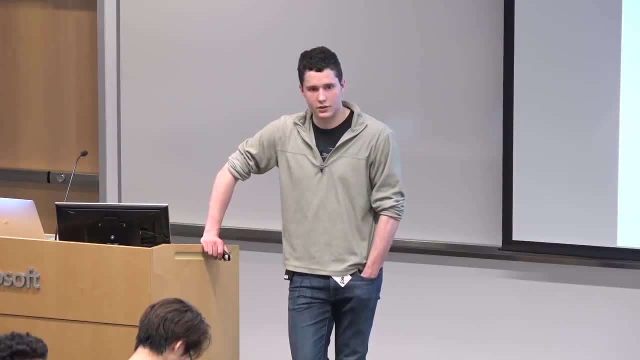 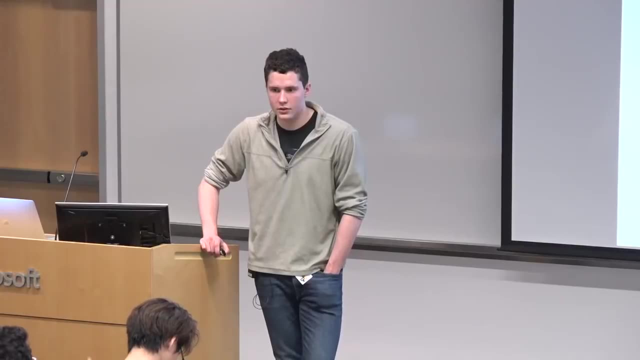 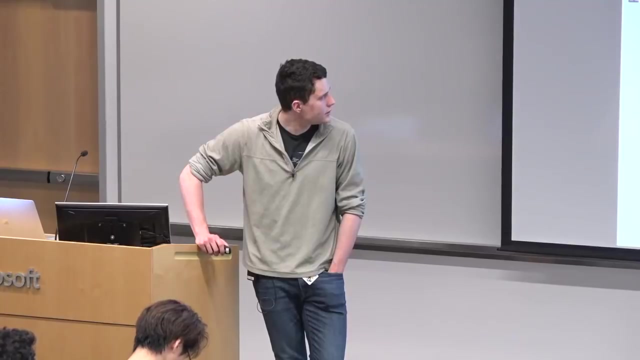 Actually so Ben Rec's paper uses a linear approximator, The random search one. Yeah, Andrew, do you have something? No, no, It's the surrogate landscapes look like vaguely linear, even for the two-layer. Yeah, So if you look at the surrogate landscapes, 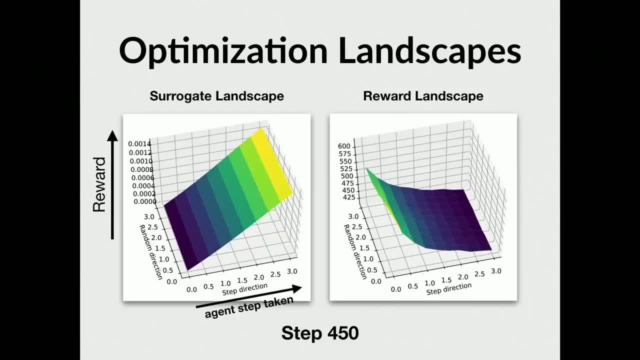 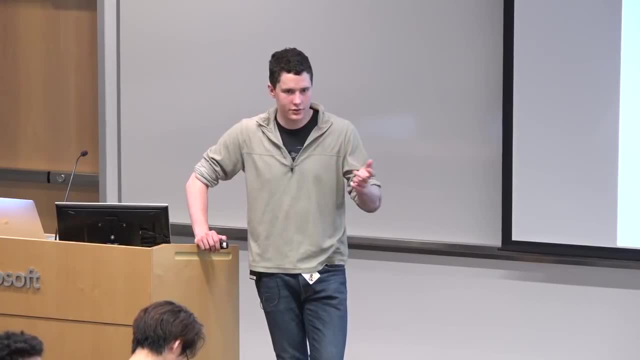 For the later stuff. Yeah, So if you look at the surrogate landscapes, they're vaguely linear, which makes sense, because I don't know if it makes sense, but they are. But the actual thing you're optimizing is linear in the outputs of the network. 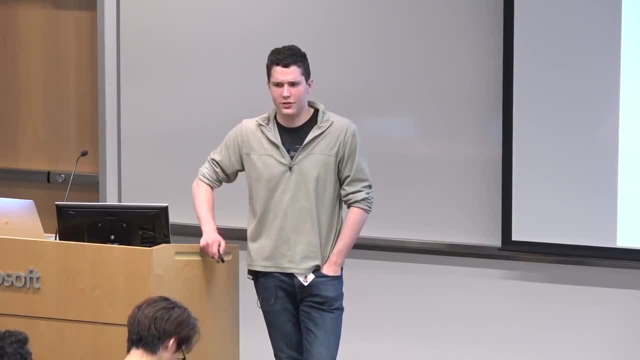 So these look pretty long. Yeah, I mean, I don't know if that's it, I'm not sure if that's a good connection. If you have a multi-layer linear network, then the optimization is not linear. Yeah, Absolutely. 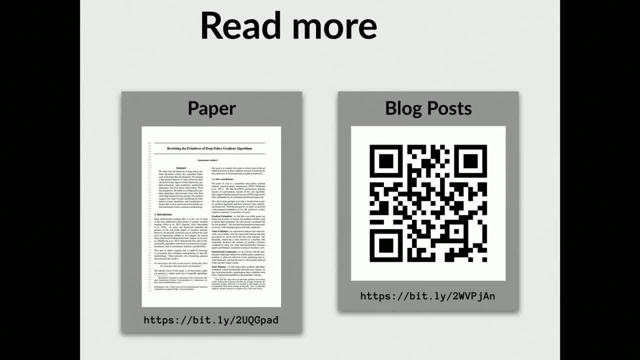 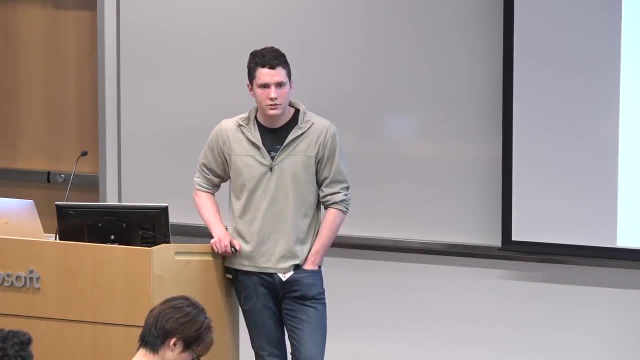 What was the network architecture used for all this? Yeah, Oh no, It was a two-layer MLP. Was the learning rate used for most of these? It varied a lot per experiment. I think we used whatever the best one it was during hyperparameter tuning. 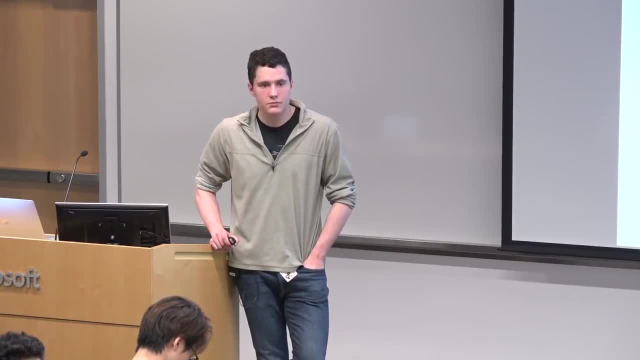 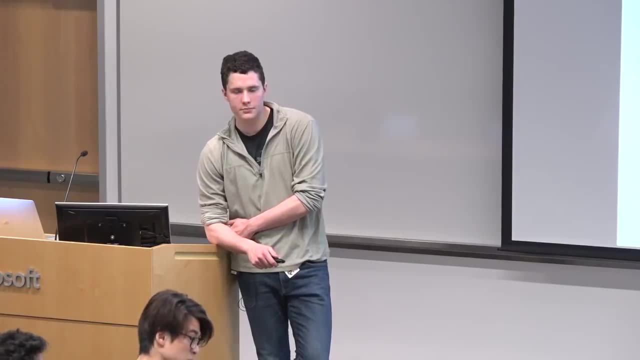 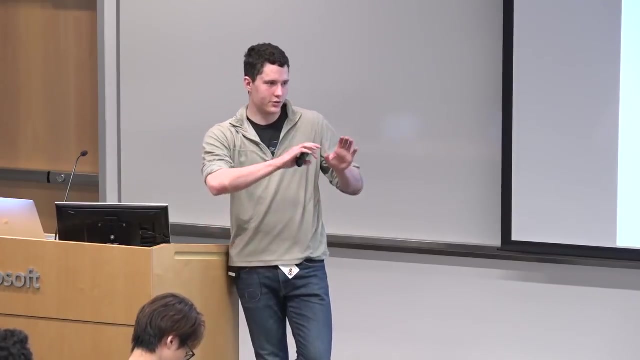 So like 10 to the negative four. I saw earlier you had this plot. Yeah, I think it was probably something around 10 to the negative two and 10 to the negative four. Do all the environments show plots like this? Yeah, So in our appendix we have everything. 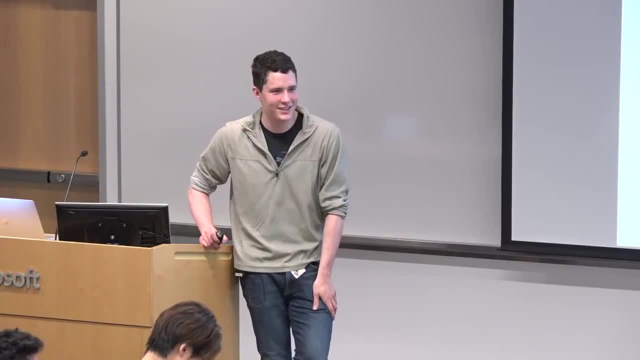 We have like 30 pages of appendix or something So you can take a look at that. So I mean for easier tasks. they look much better. I would say We mostly looked at it in this Walker2D, which is the hardest one. 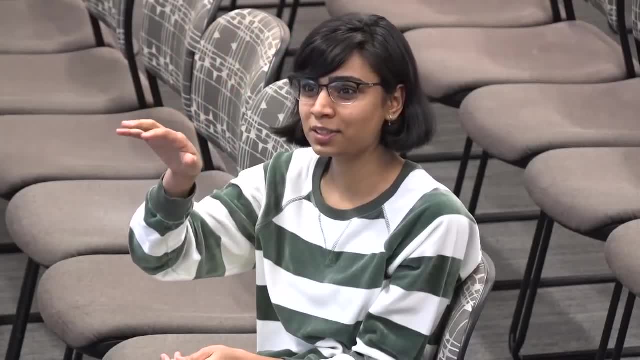 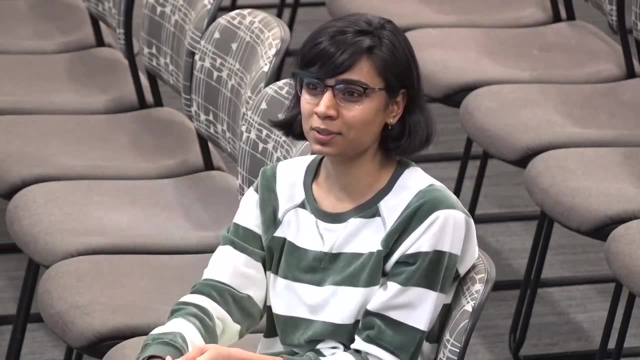 Yeah, It's curious. You would imagine that more unstable environments- probably they're more sensitive but more stable, and perhaps things that balance they're more unstable, whereas maybe things like cheetah and stuff they're more stable. I think that was the rule, but apparently not. 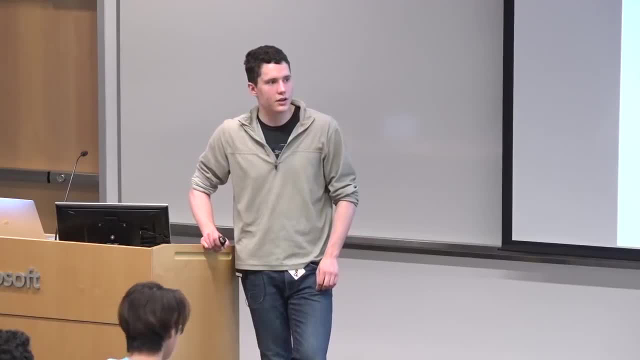 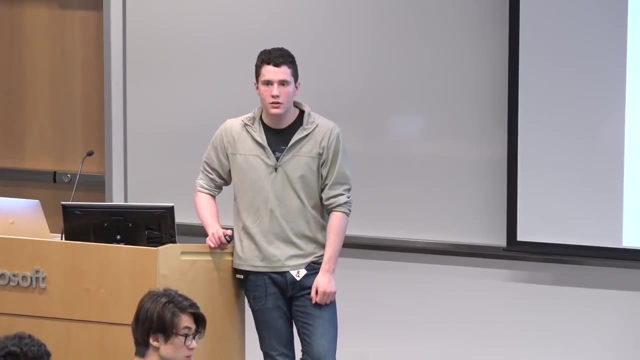 Yeah, I guess I'm not sure. I'm not sure. I don't really have a good intuition for how the different games should work. Maybe I missed this. So, thinking about RL evaluation, do you have a constructive suggestion for how we might go? 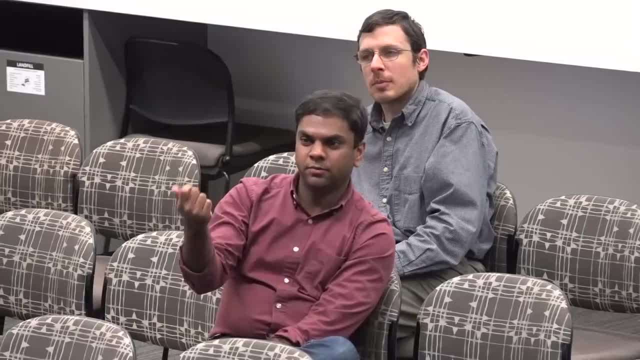 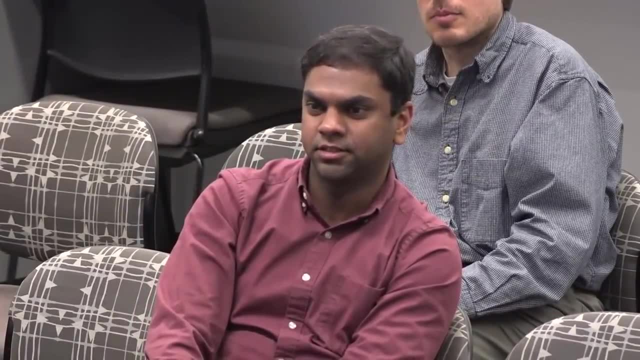 beyond just benchmarks and eventual average rule, What might be an alternative evaluation that exposes, like this, hypersensitivity to hyperparameters and things like that? Yeah, I mean, so we never talked about ideas for that. We haven't talked about ideas for that yet. 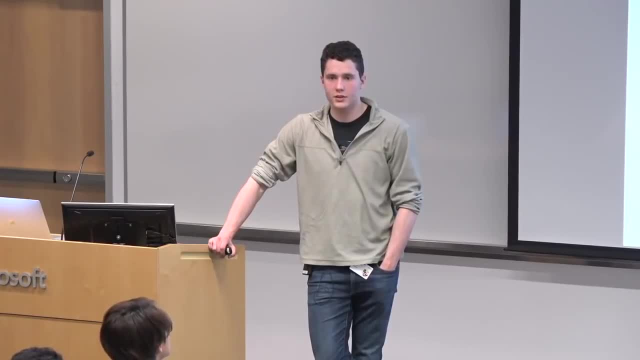 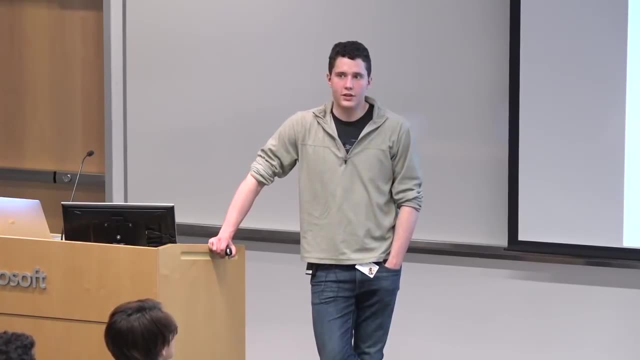 I guess we haven't thought about that too much. I would say that one thing would at the very least so. if you look at a lot of these papers when they showcase results, they show the results in a way that makes it look more stable than it is.